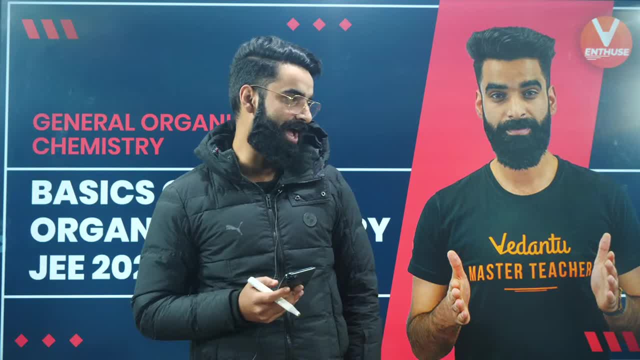 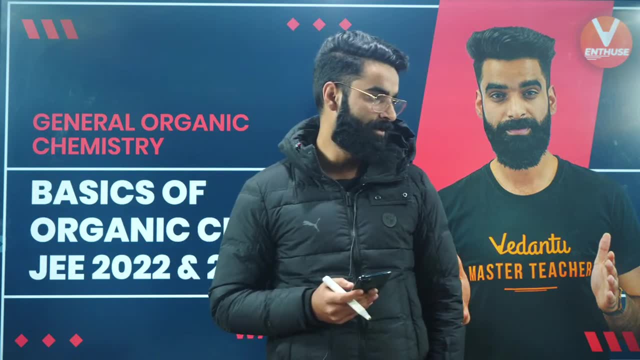 Hello Dark Angel, Hello Ishpreet, Hello Good and Bold Girl, Hello Roshni, Hello Syed, Hello Praneesh, Hello Aishwarya, Hello Dakshin, Hello Shruti. 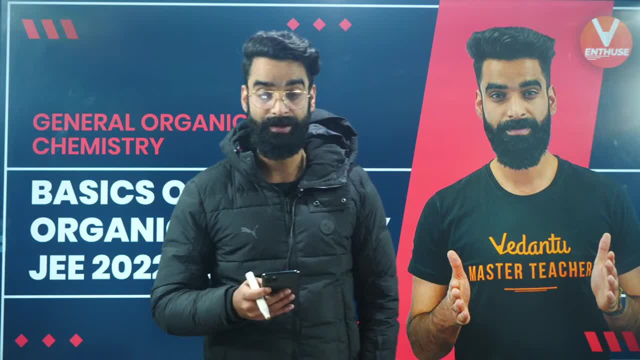 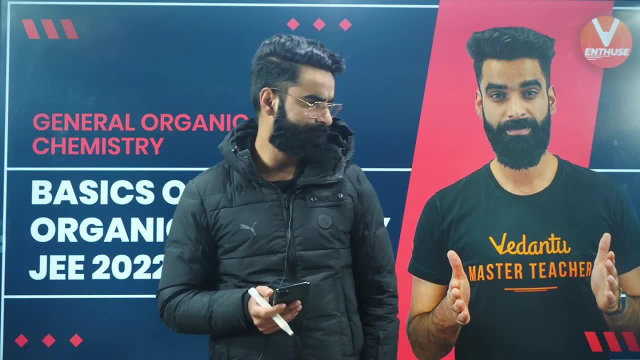 Welcome back, Welcome back, my dear people. Welcome back, Welcome back. Just give me some green seal from the chats first of all, so that I'll get to know that I'm audible and visible to you guys properly. Yes, Welcome back people, Welcome back. I'm doing good, I'm doing good. How are you guys doing? 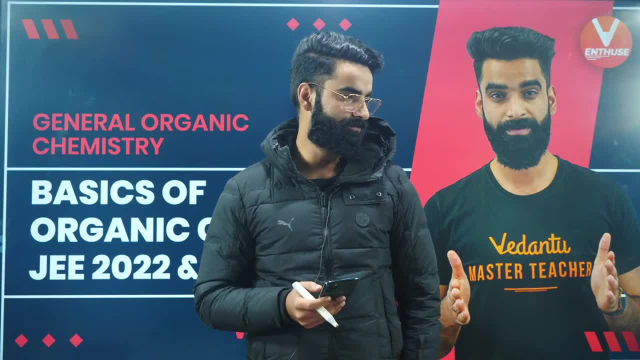 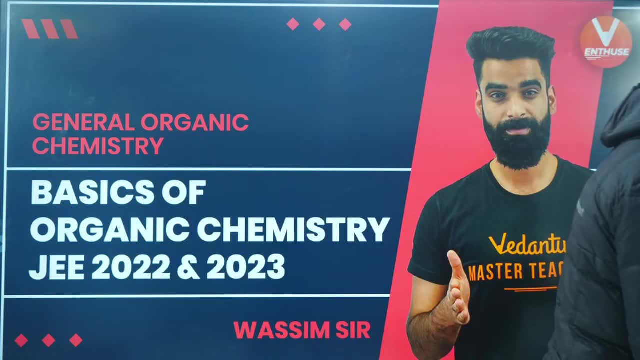 I'm doing good, Aisha. How are you? I'm doing good, Syed. What's up with you? So I think I'm perfectly audible and visible to everyone, right? Okay, just give me a second. We will be starting right. 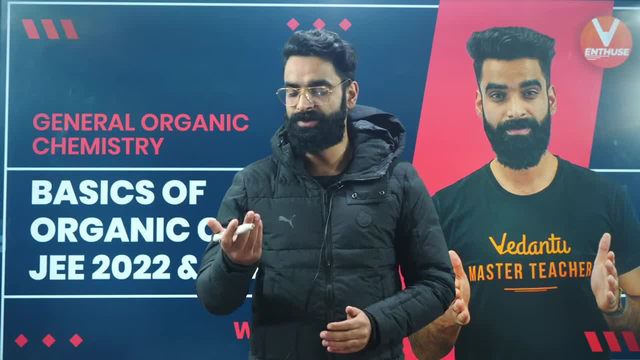 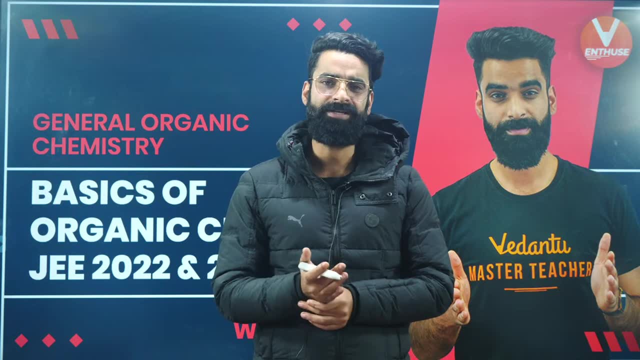 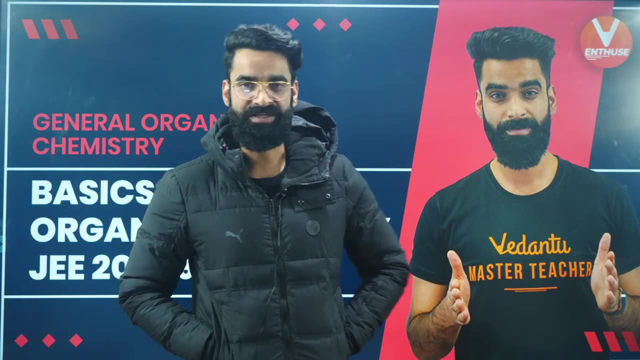 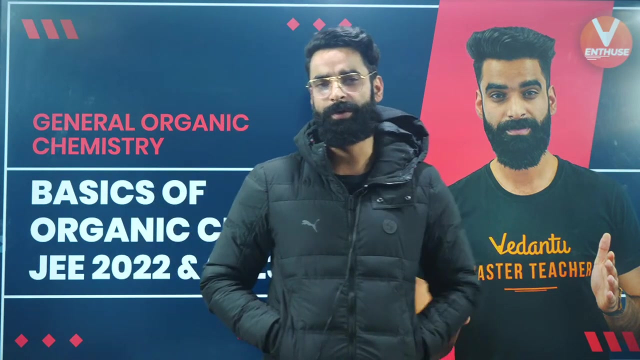 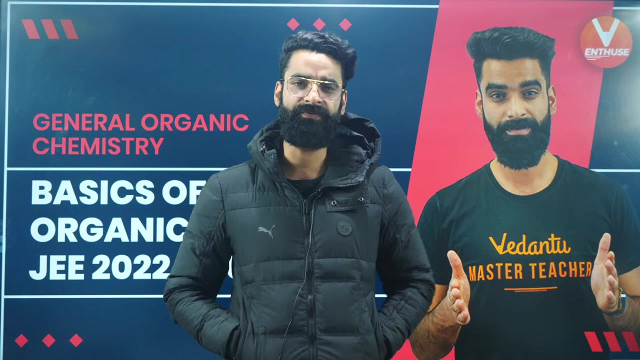 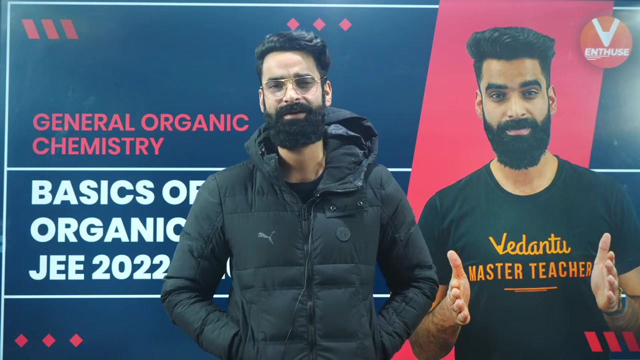 Okay. so, people, as you all must be knowing, tonight we are going to start one more chapter right of your class 11th chemistry, which is one of the most important chapters, right from your organic chemistry Chapter is going to be GOC right, which is basically general organic chemistry, right? So what all things we are going to cover in the tonight's session? in the tonight's session, we will be talking about something really interesting which is going to be very, very helpful to you, right for your entire organic chemistry right. I'm going to talk about some basic, basic things, right, which you must know before starting the actual organic chemistry right. 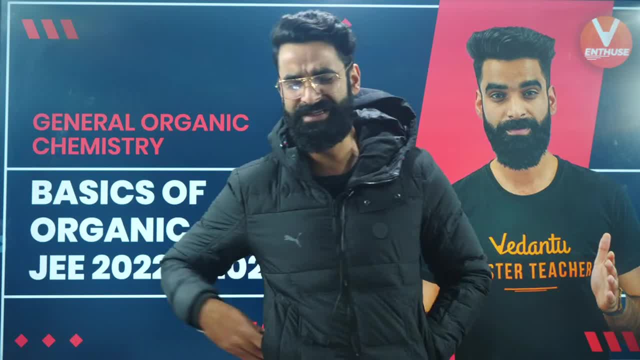 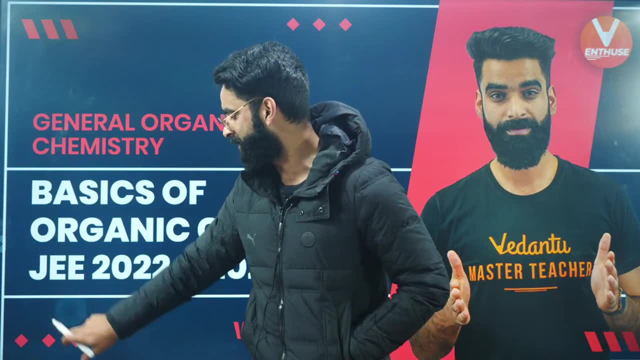 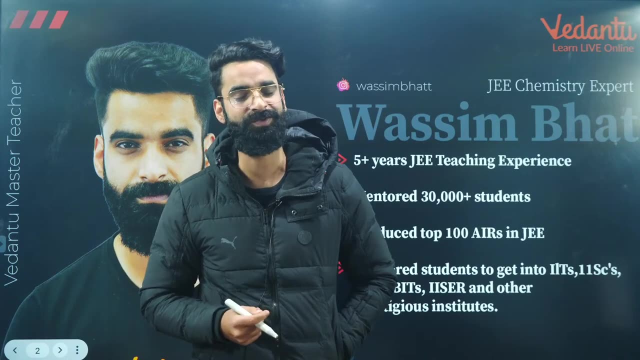 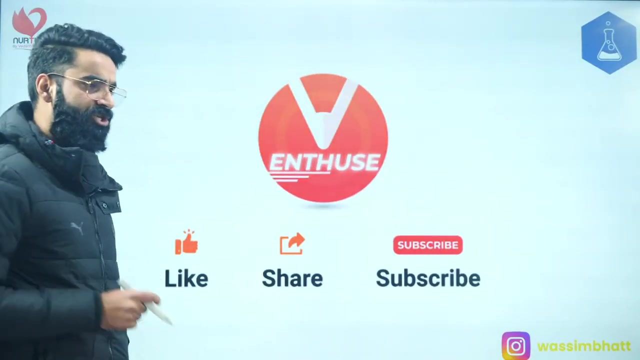 Yes, so these are basically going to be the basic things of the GOC which I'll be covering in the tonight's session, right? So before starting the session- the ones who have just joined in, the ones who are new to the channel- let me introduce myself. Well, my name is Vasim Bhatt and I'm your chemistry master teacher, writer on this VJNTO channel, right? At the same time, the ones who have not liked the video yet, please do like the video. share the video with your friends, do subscribe to the channel and do not forget to hit the bell icon so that you get notified when I post a new video. 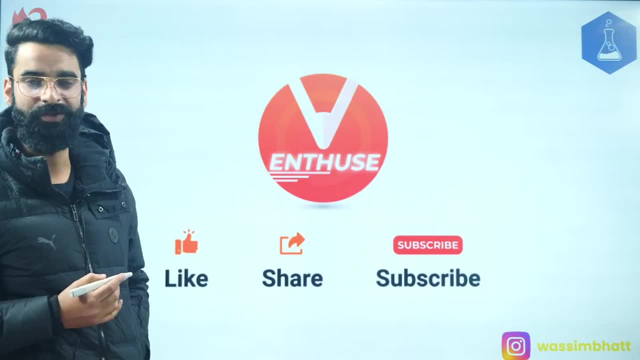 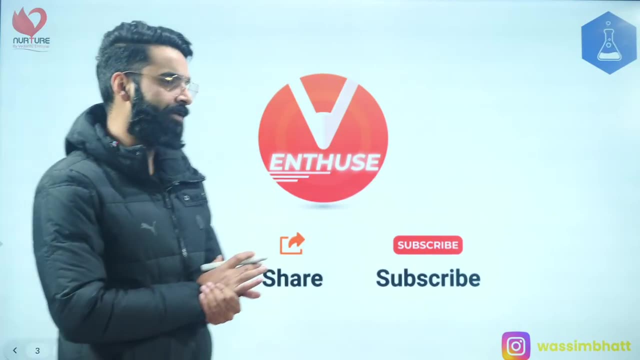 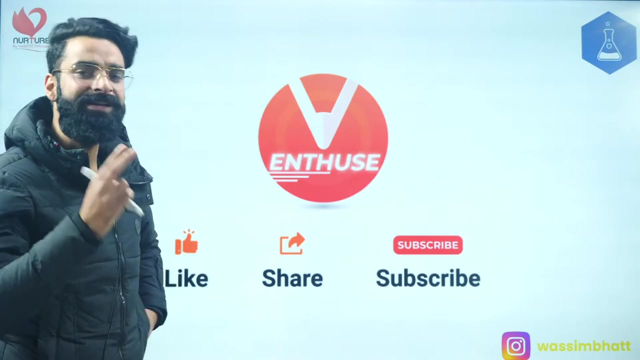 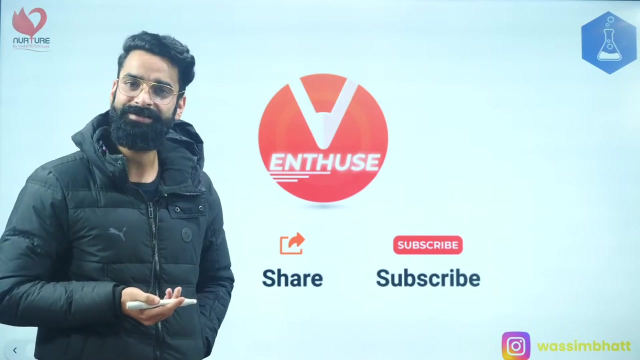 notification of every single session which we take live on this VJNTO channel, right? So do like the video, share the video with your friends and do subscribe to the channel as well. Yes, Dinesh, ionic equilibrium is not completed yet, Absolutely. I'll be taking sessions for ionic equilibrium as well. So we'll be parallelly taking two chapters, general organic chemistry and at the same time we'll be doing the ionic equilibrium as well. Correct, Right? So first of all, you guys can let me know in the chats if you all are super, duper excited for the. 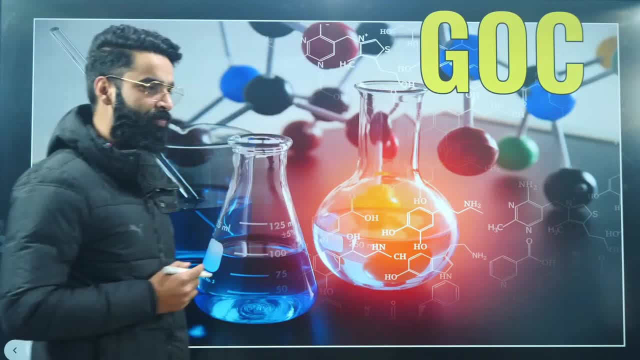 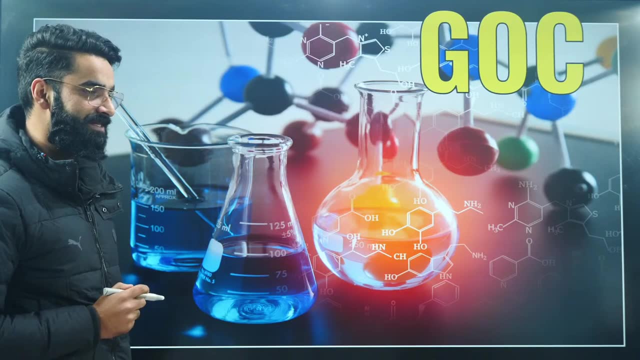 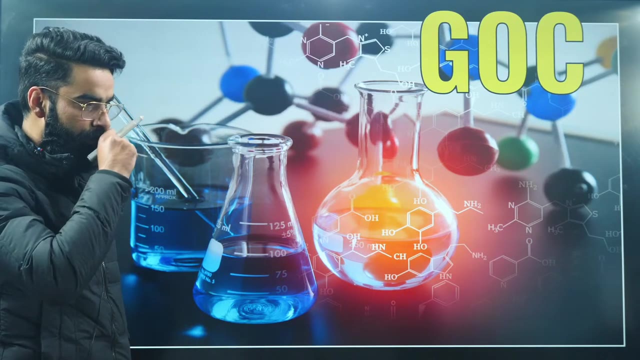 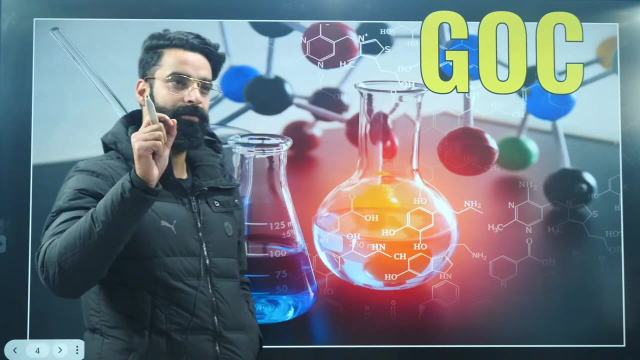 tonight's session. right, Let me know fast in the chats if you all are super duper excited for the tonight's session. Let me see the Josh of the session. Yes, Let me see the Josh of the session first. then we'll be starting the chapter. right, Josh is high, it seems. Yeah, All right, Wonderful, Wonderful guys. First thing, before starting the session, whatever I'll be writing on the screen, I want you guys to take a note of every single thing, right? 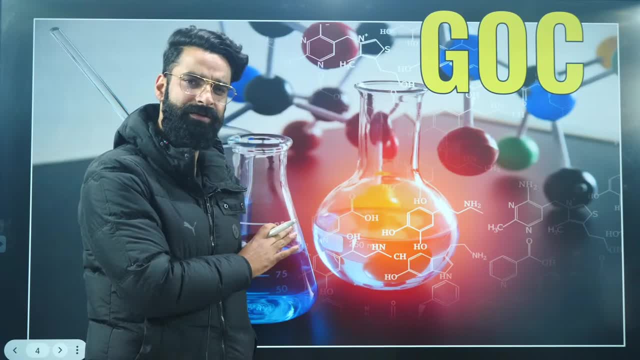 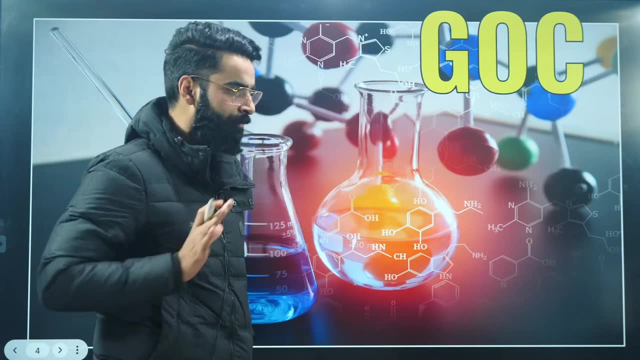 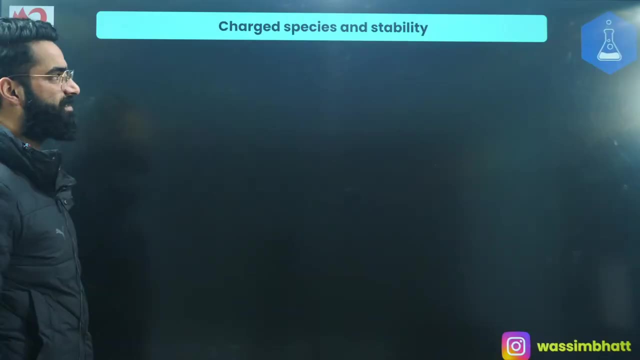 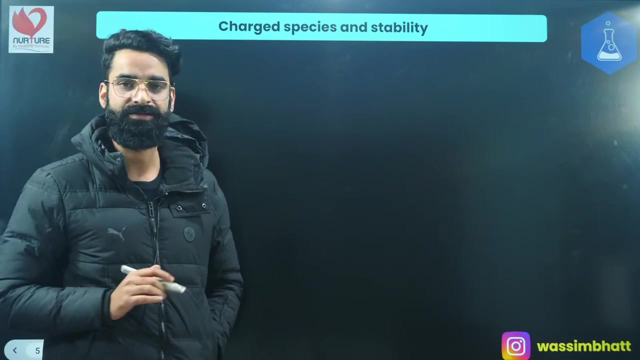 Whatever single thing will be mentioned on the screen, right? I want you guys to take a note of every single thing from the session, correct? It's going to be very, very important things which I'm going to discuss in the tonight's session. Yeah, So, without wasting a lot of time, let's get going. Let's get started And let's first of all talk about the charged species and their stabilities. This is the first basic thing which I'm going to cover in the tonight's session. Okay, 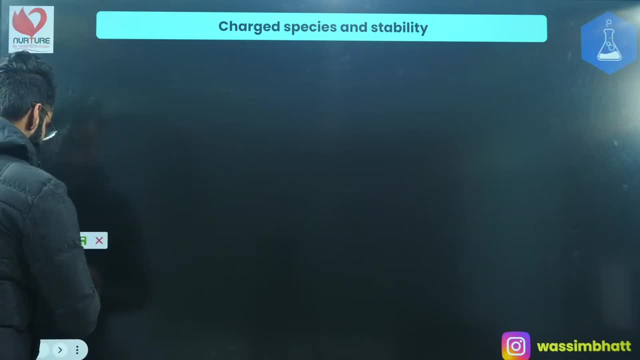 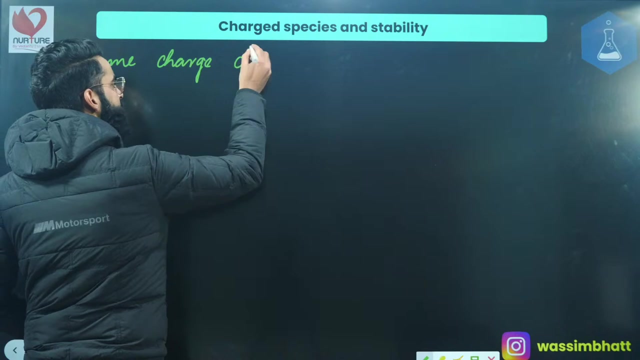 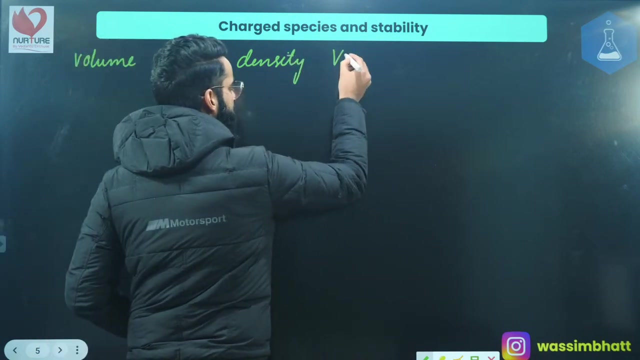 First of all, I'm starting this general organic chemistry with a term which is called as volume charge density. I'm starting the general organic chemistry with a term which is called as volume charge density, Volume charge density And this volume charge density is represented with VCD. VCD stands for volume charge density right. 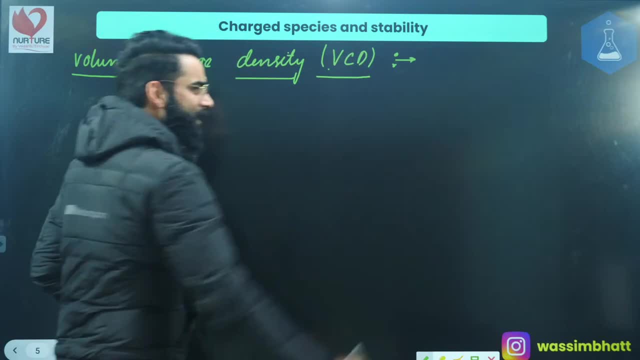 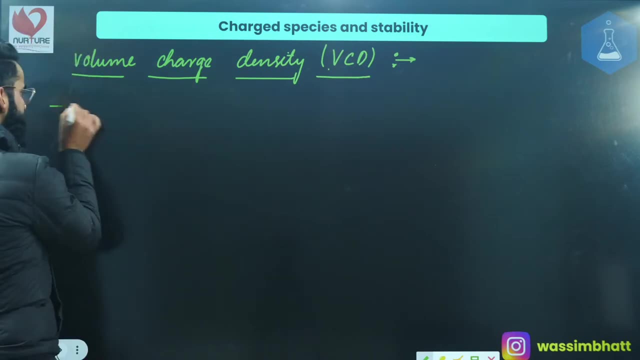 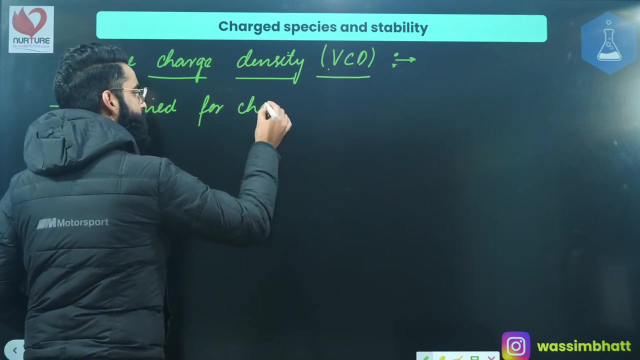 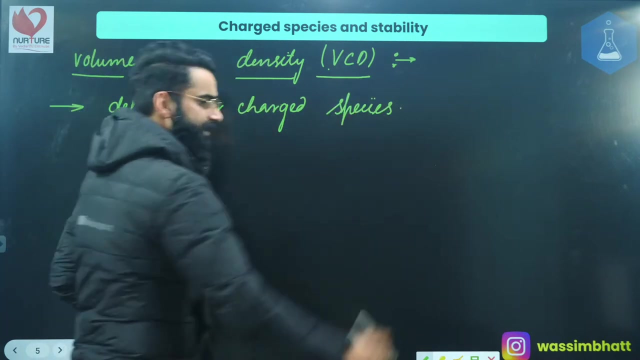 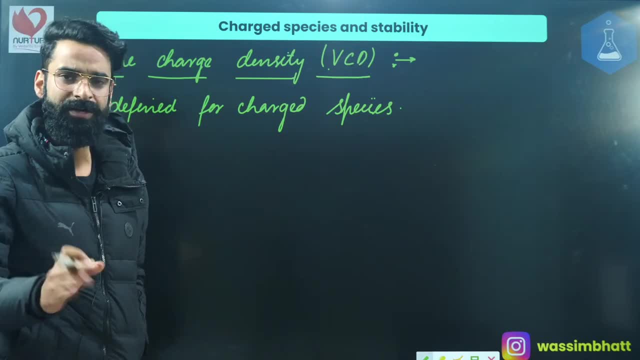 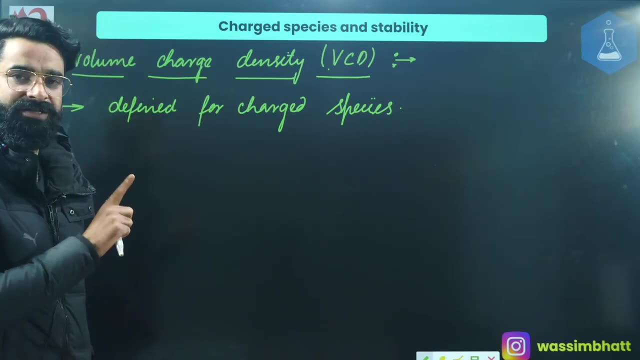 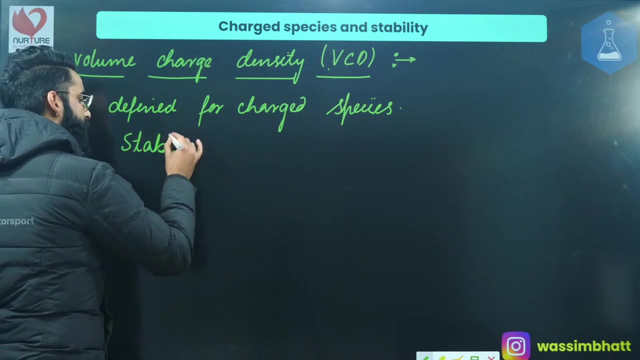 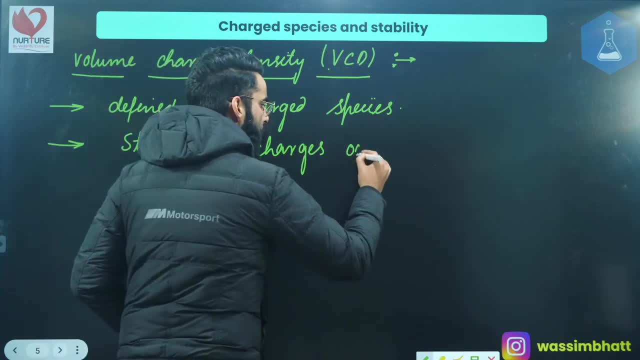 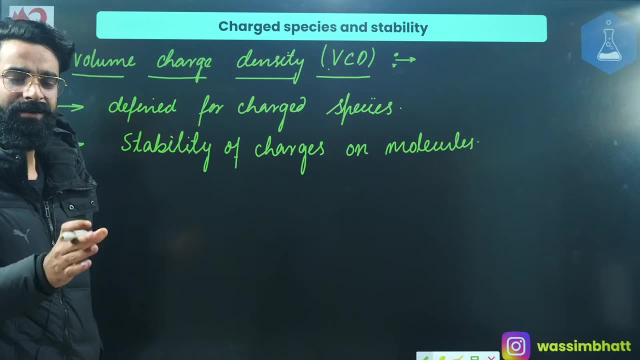 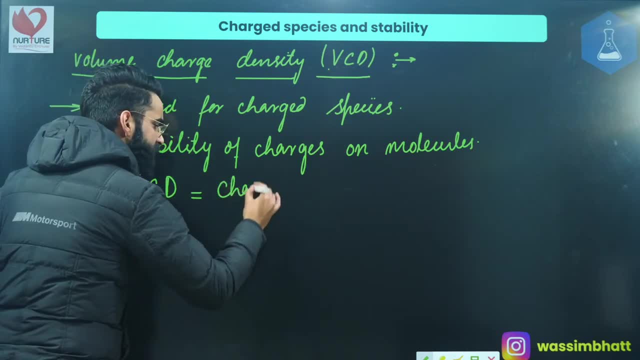 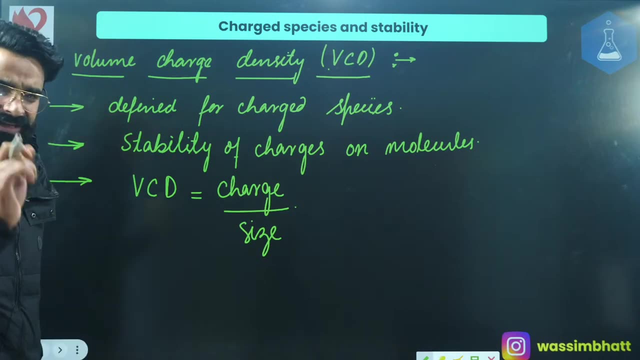 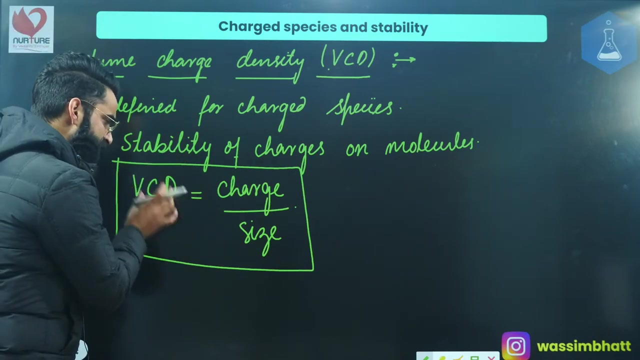 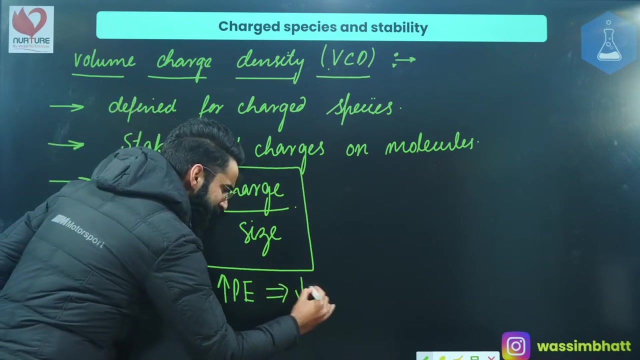 more the volume charge density of a specie, more is going to be the potential energy of the specie. more the potential energy of the specie, less is going to be the stability of the specie, less is going to be the stability. 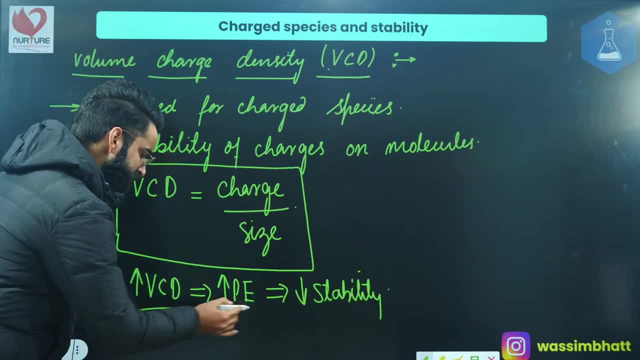 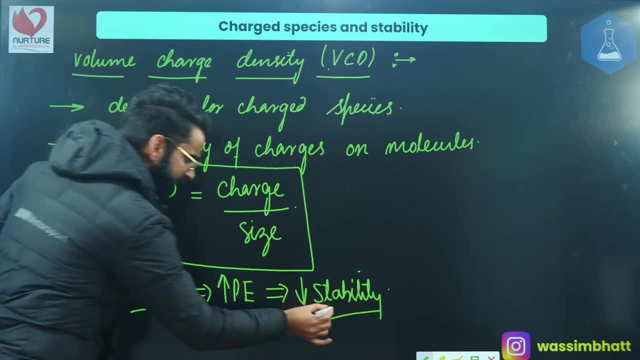 of the specie right. More volume charge density means more potential energy means less stability. or you can generalize a statement over here: Volume charge density is inversely proportional to stability right. This is a general thing which I'm generalizing over here. This is: 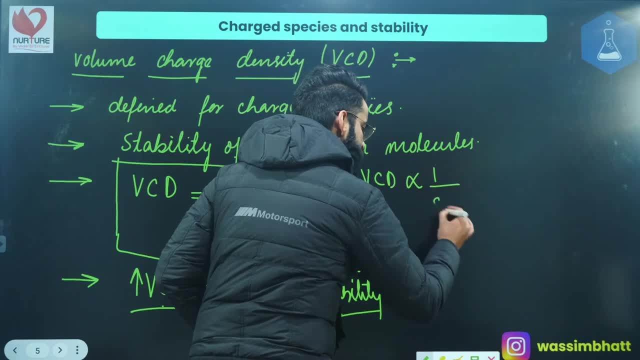 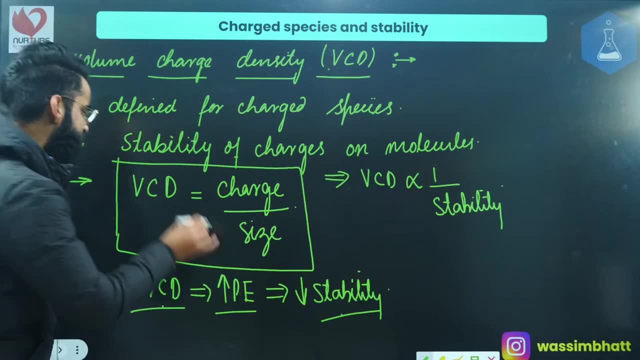 volume charge density. It is inversely proportional to the stability. These are some basic things which I want you all to take a note of first of all. yeah, So first of all, this volume charge density: it is defined for the charged specie and volume charge density of any charged. 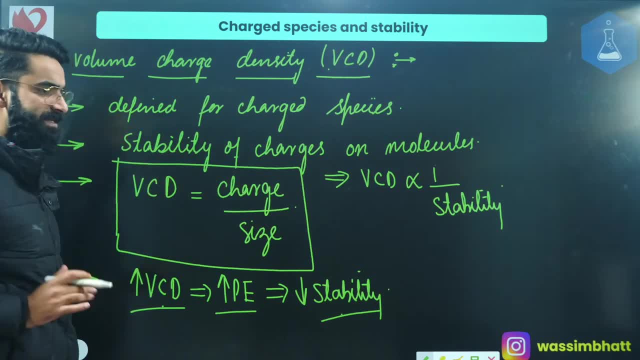 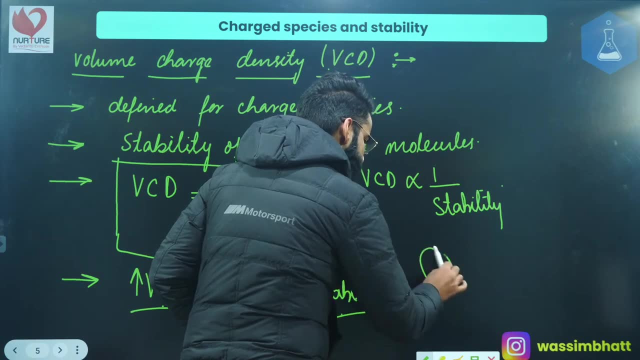 specie is always equal to the charge present on the specie divided by size of the specie. right? Let's say I've got two species over here. Let's say I've got two species over here. This is one specie. This is one more specie, right? Let's say both the species are carrying. 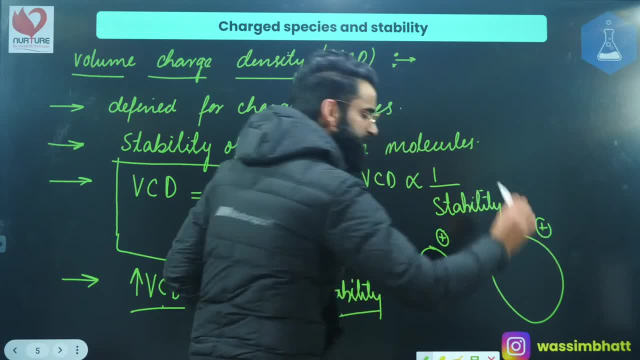 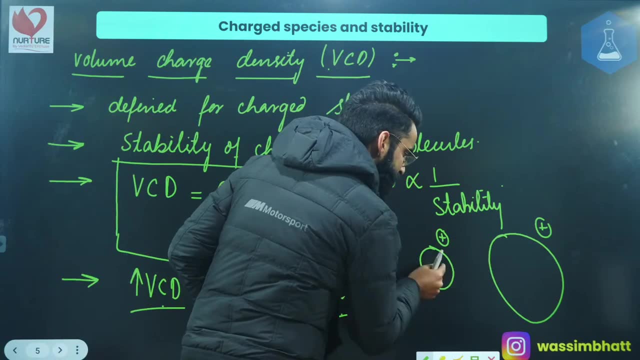 same amount of positive charge on them. Let's assume both the species are carrying a positive charge, same amount of positive charge on them. So for these positively charged species I will be defining a term called as positive volume charge density For these two species. 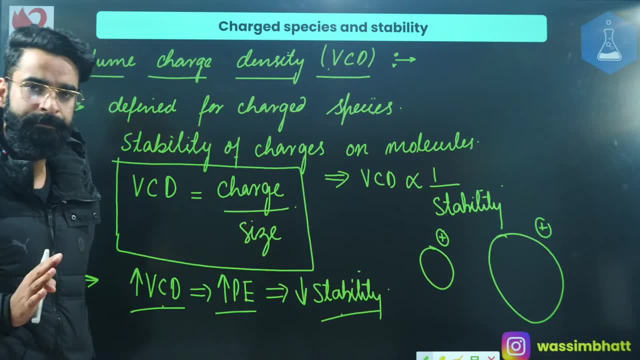 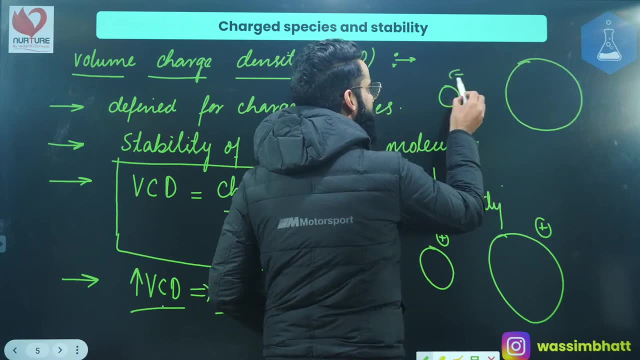 I'll be defining a term called as positive volume charge density right. Yes. Similarly, if I'll be having two species- one, two, three, four, five, six, seven, eight, nine, ten, 11,, 12,, 12,, 13- and they will one, one, two, three, four, five, six, seven, ten, 12.. So 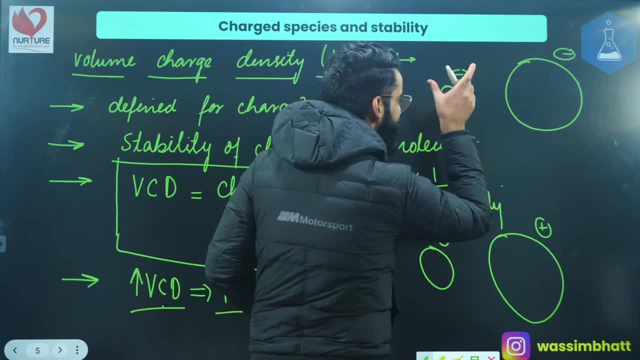 we will be configuring a gauge of one like this one Like this one like this, this scanning the negative charge and this specie carrying the same amount of negative charge right. For these two species, I will be defining the negative volume charge, density right. 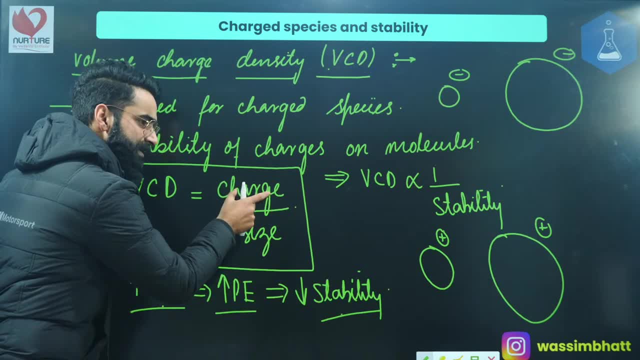 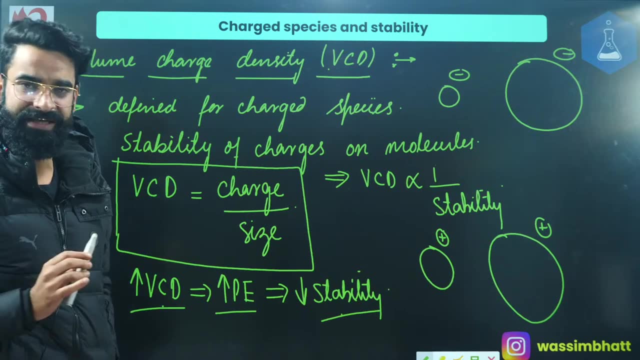 Volume charge density, be it positive or negative, It is directly proportional to the charge present on specie and worse, He proposed out, to the size of this specie. right, It's directly proportional to jobs. president, on specie, university proportion. on the size of the species. 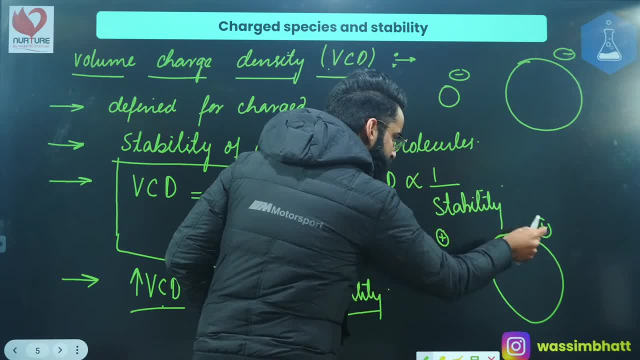 If I ask you, among these two species, is the amount of positive and negativecipe? the numbers are not secret, is it correct? Is it because they are이었ingly pick it? the size, amount of positive charge same present on them? absolutely, amount of positive charge is same. 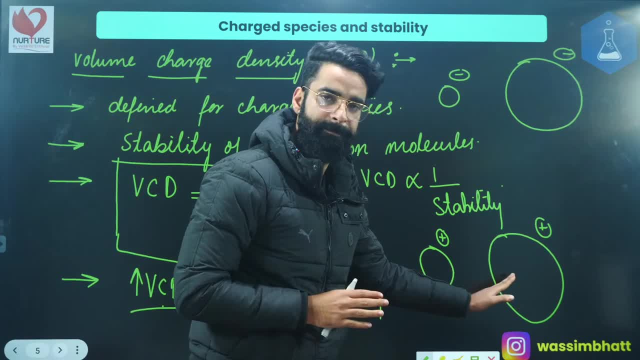 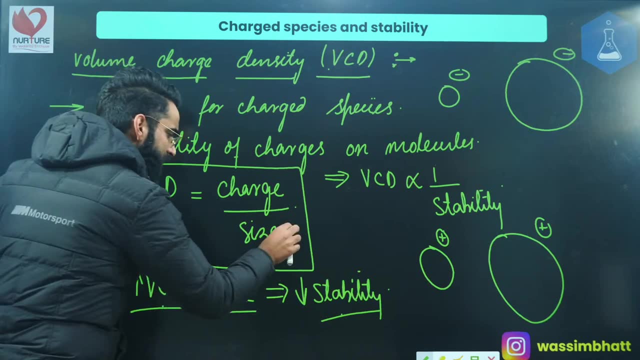 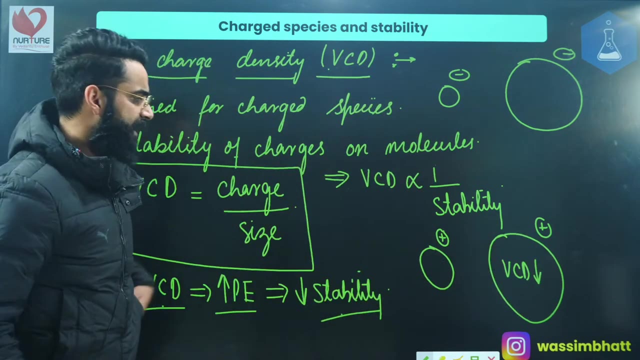 present on them. right amount of positive charge is absolutely same. present on them, yes, but over here size of this specie is more. if size of the specie is more, that means volume charge density of this specie will be less. volume charge density of this specie will be less. and if volume charge density 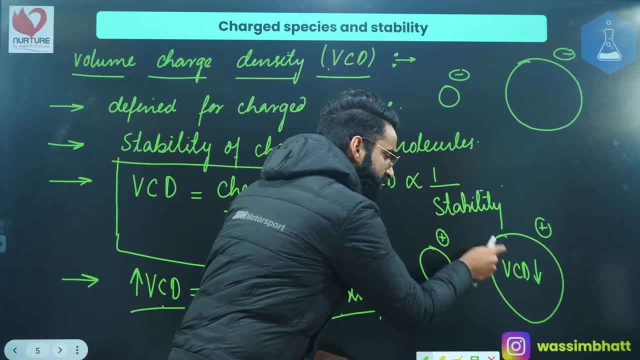 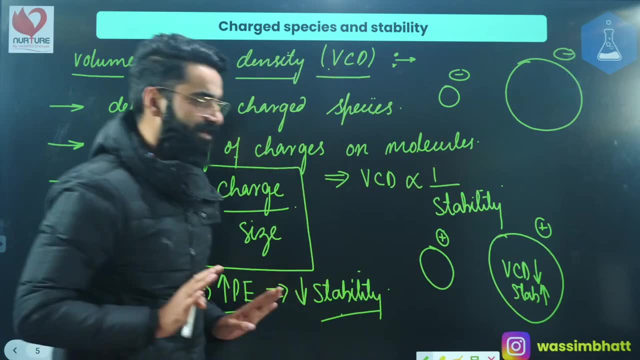 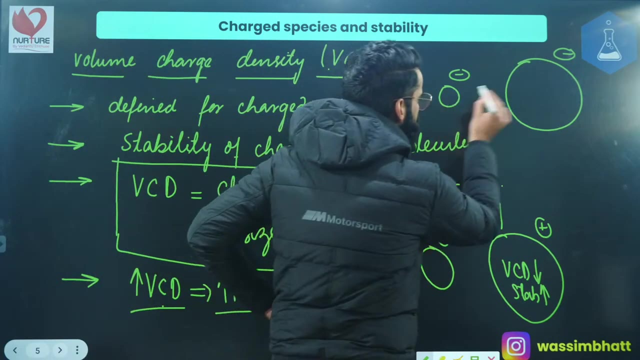 of this specie will be less. that means stability of this specie is going to be more right. you can say: stability of the positive charge on this specie is going to be more. as simple as that, right. stability of positive charge on this specie is going to be more. yeah. similarly, we have got two. 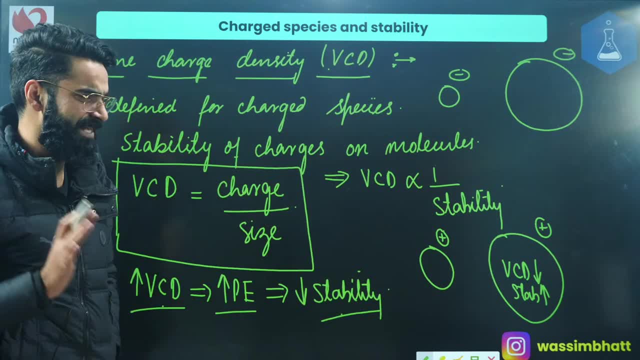 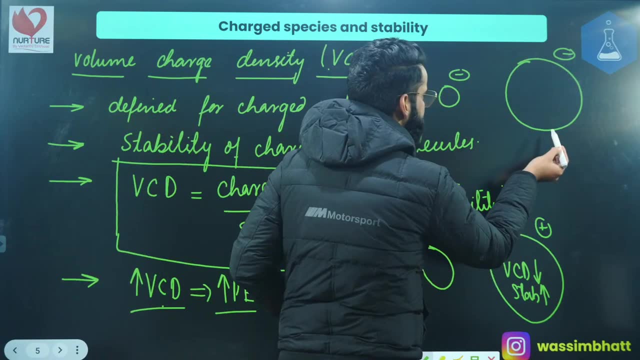 more species carrying same amount of negative charge. for example, same amount of negative charge correct. first of all, the amount of charge present on both the species is same, but their size is different. more the size, more the size, less will be the volume, charge density and less the volume. 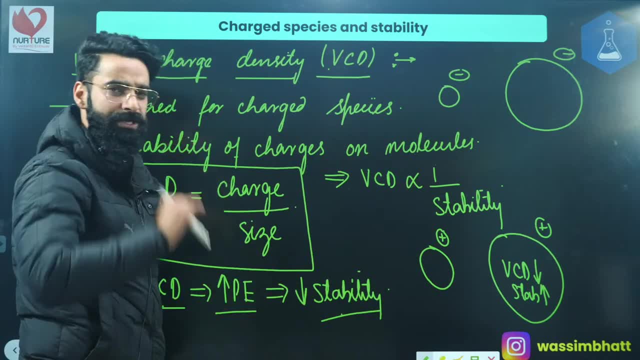 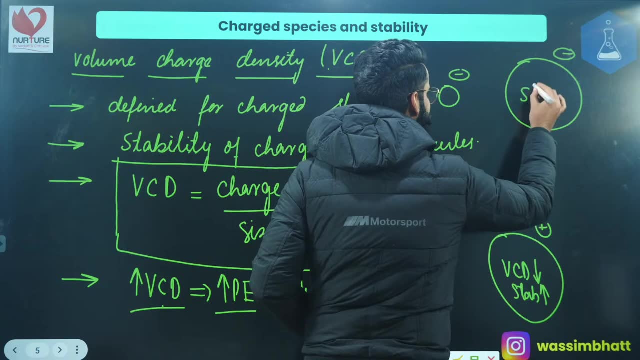 charge density. more is going to be the stability. if i ask you where among the two, where in among these two species, negative charge will be more stable, you will say negative charge will be more stable on this specie. you will say negative charge will be more stable on this specie. right, whenever i compare. 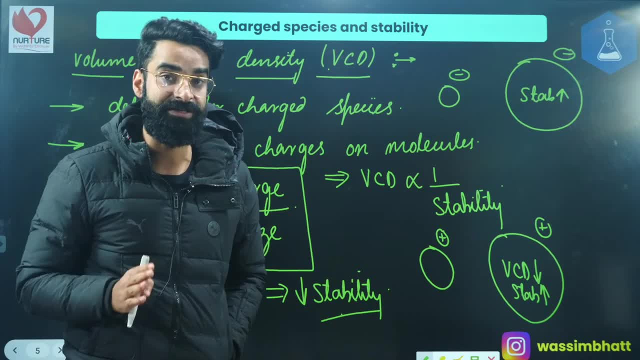 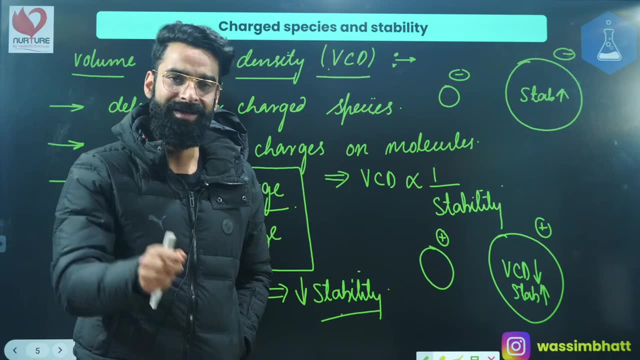 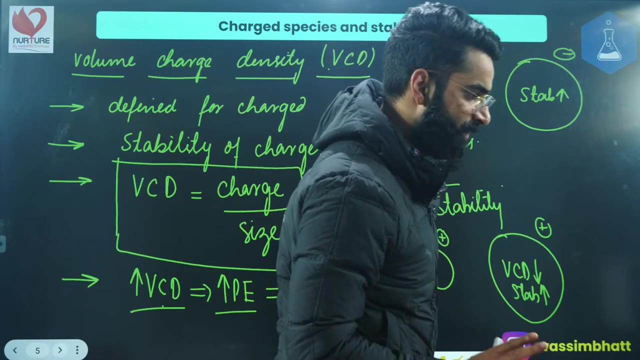 the stability of the charges on the basis of volume charge density. whenever i'll be comparing the stability of the charges on the basis of volume charge density at that point of time. do you remember? lesser the volume charge density, lesser the potential density of the volume charge density, more the stability. as simple as that, right. yes, i'm sure. till here, every single thing will be. 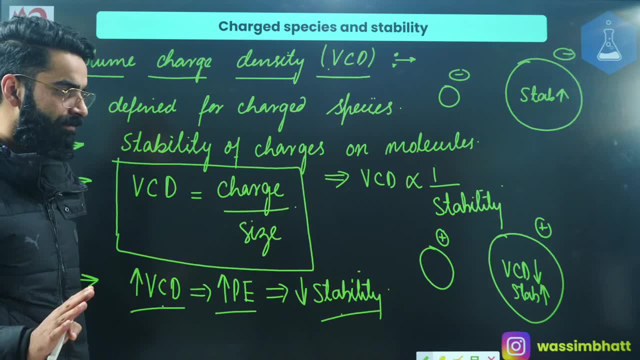 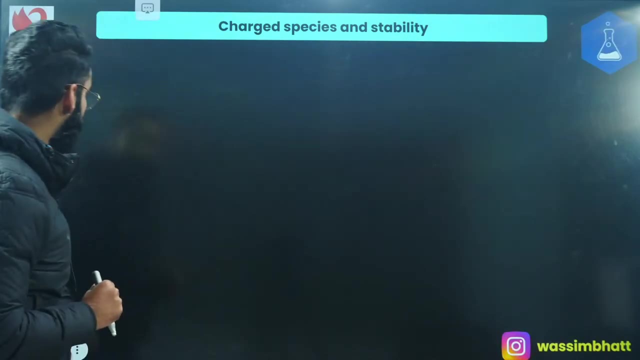 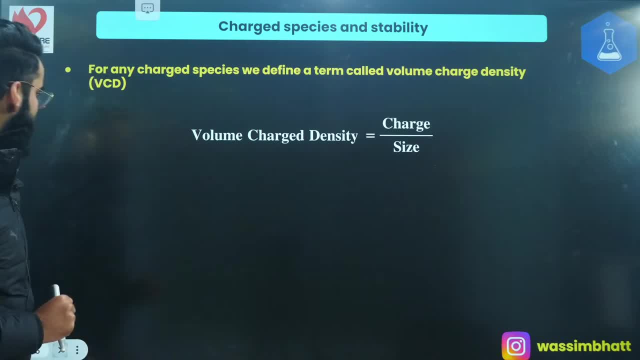 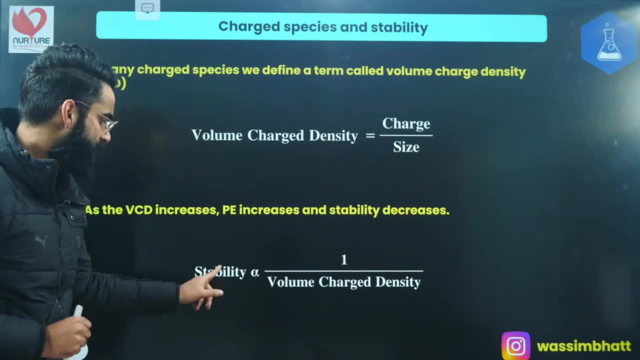 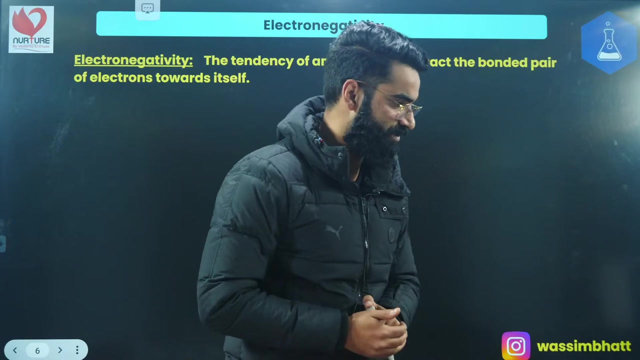 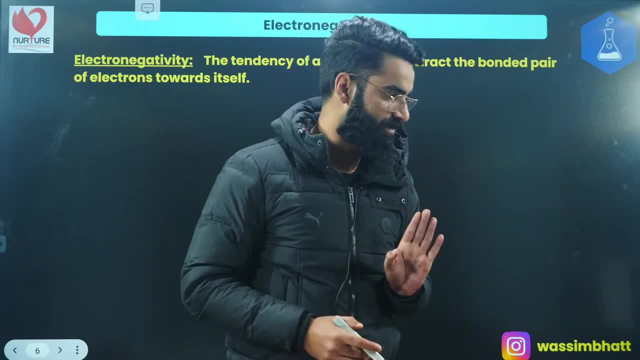 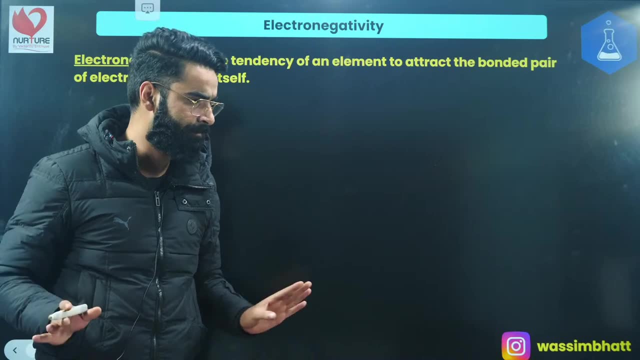 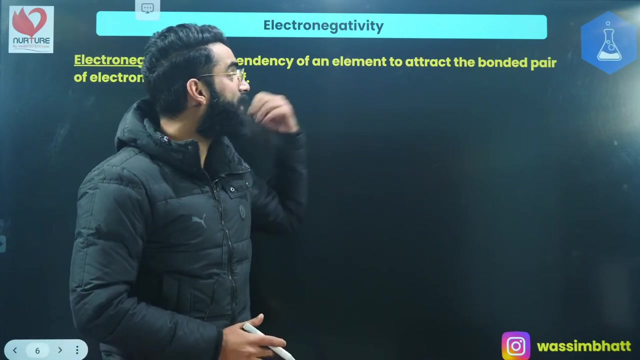 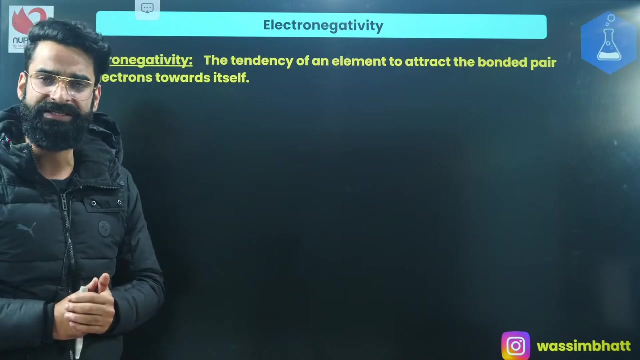 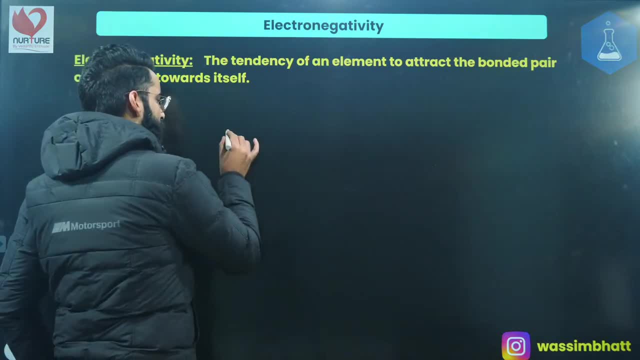 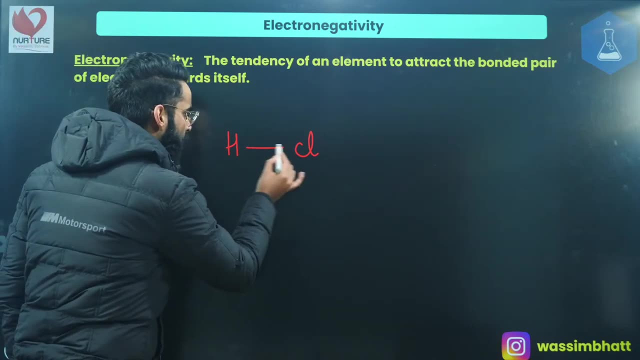 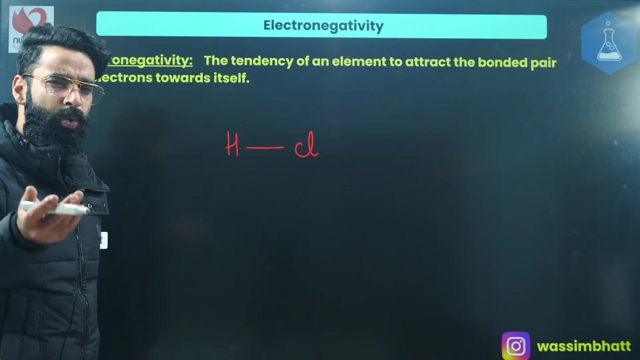 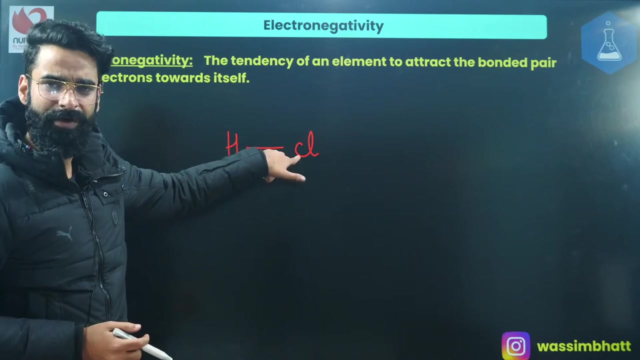 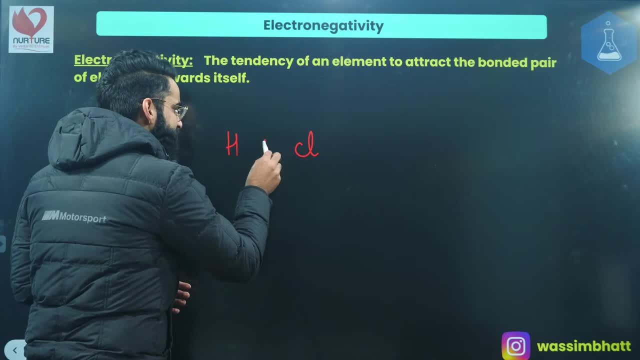 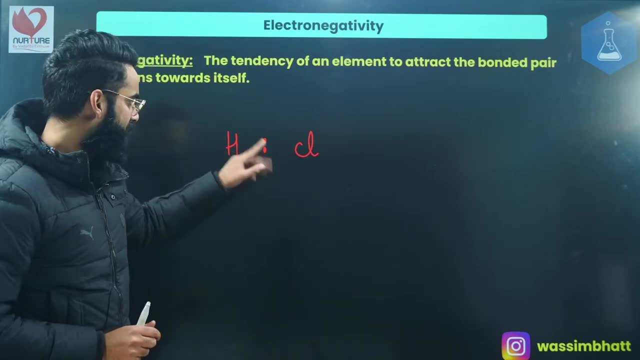 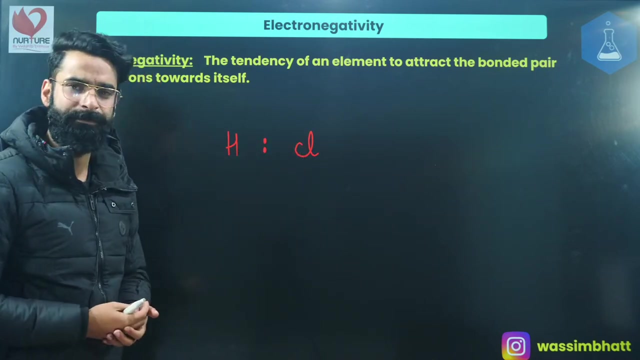 electron pair forming this bond to be at the center. I would expect this electron pair which is forming, which is involved for the bond formation. I mean, I expect this electron pair to be present at the center. But, as you all must be knowing, chlorine is more electronegative than hydrogen. that means 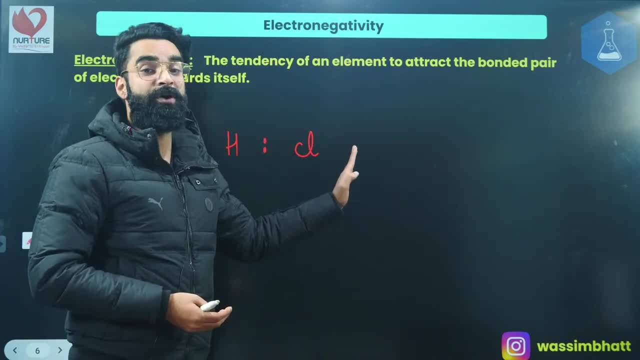 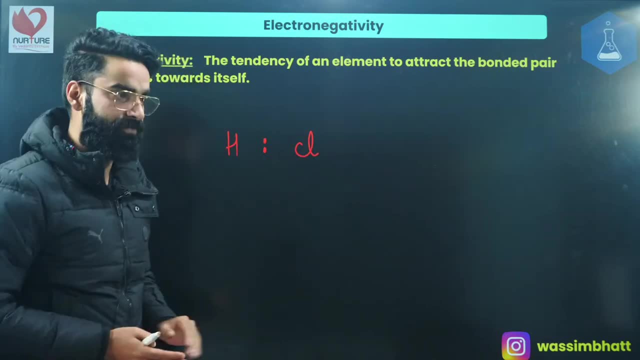 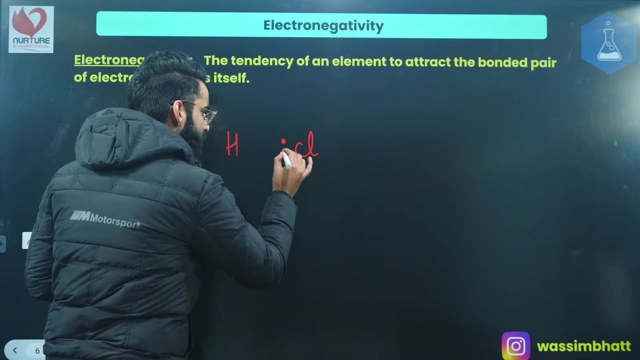 chlorine has got more tendency to attract this bonded pair of electron towards itself. If chlorine has more electronegativity, if chlorine has got more tendency to attract the bonded pair of electron towards itself, I must say this bond pair of electron is going to shift towards chlorine, right? 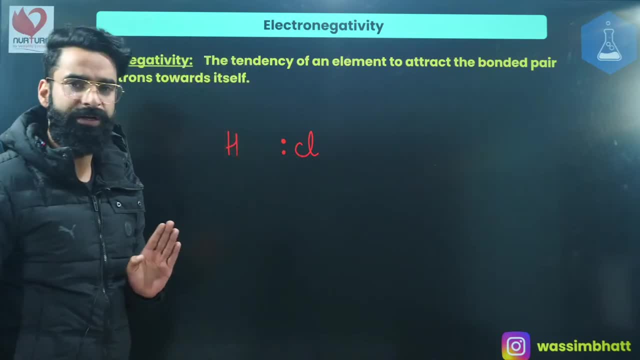 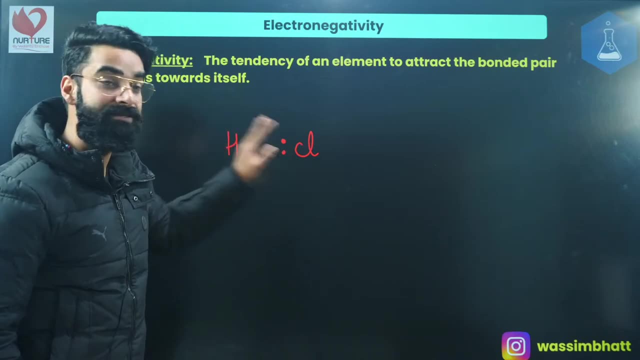 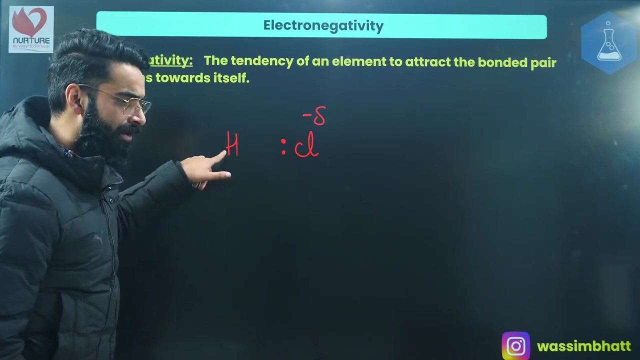 So if the bonded power of electron is shifting towards chlorine, what is going to happen? Can I say electron density towards chlorine is increasing and that increase in the electron density towards chlorine I will be representing that by delta negative right. Can I say there will be decrease in the electron density of this hydrogen. 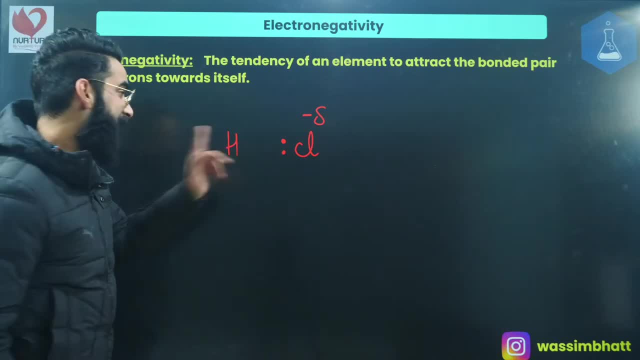 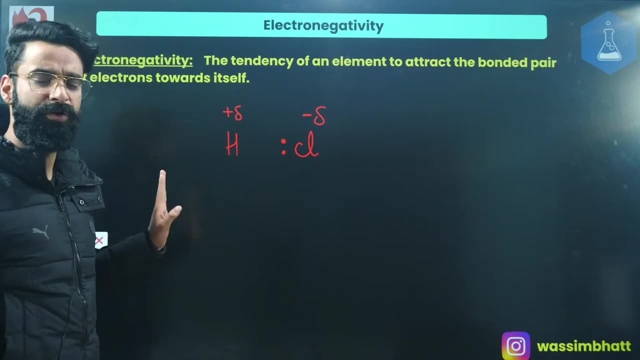 There will be decrease towards the electron density- Yes, Yes- density of this hydrogen. and that decrease in the electron density towards hydrogen I will be representing by delta positive, right? yes, this is something which every one of you would be knowing, correct? so what is electrode negativity? basically, it is defined as it is. 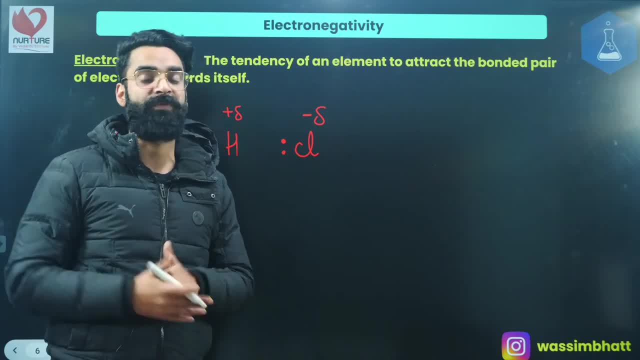 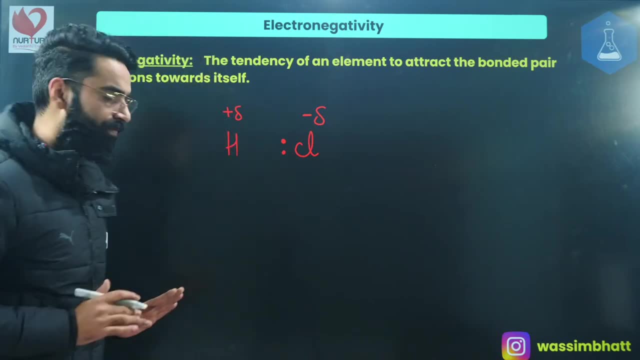 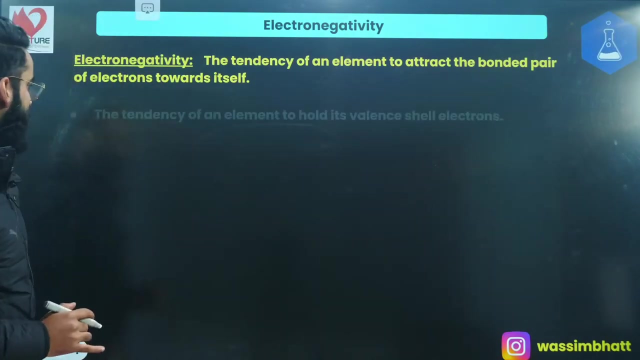 defined as the tendency of an element to attract the bonded pair of electron towards itself. right? yes, as simple as that. this is one way by means of which we can define the electronegativity. what about the another way? what about the another way, right? electronegativity, electronegativity. 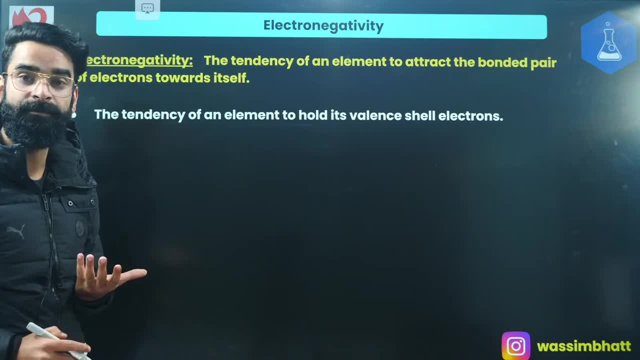 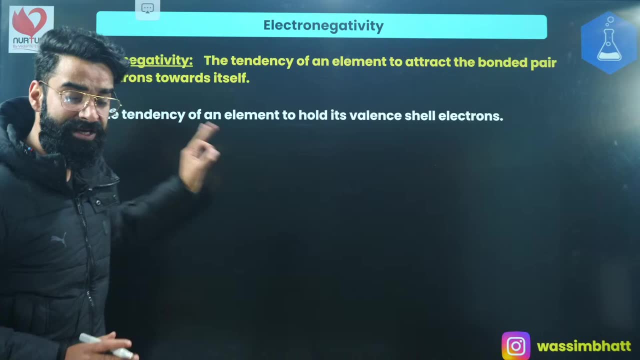 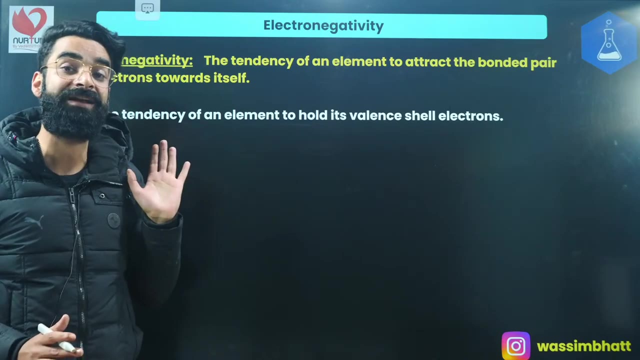 it tells us about the tendency of an element to hold its valence shell electron pairs to shoot to hold its valence shell electrons- right electronegativity of an element. it is going to give us the idea about the tendency of an element to hold its own valence electrons. 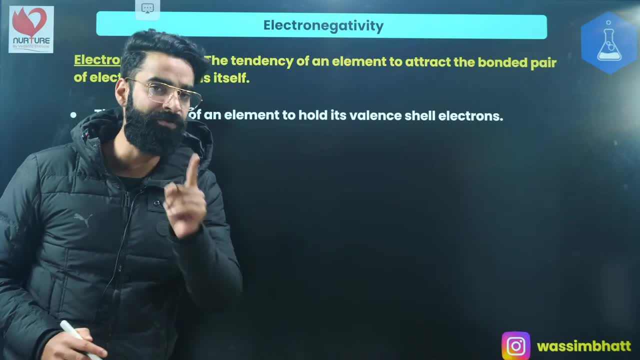 right. more the electronegativity of an element. it is going to give us the idea about the tendency of an element to hold its own valence electrons right. more the electronegativity of an element, more will be the tendency of the element to hold its valence electrons. 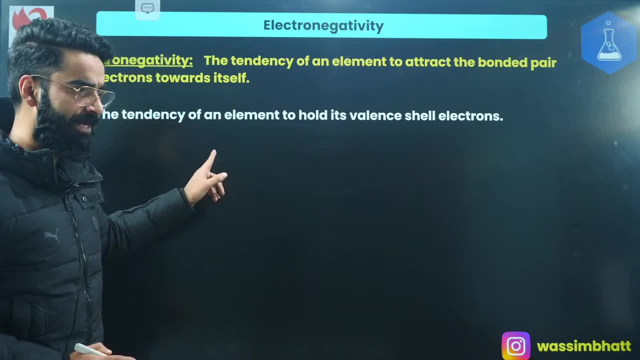 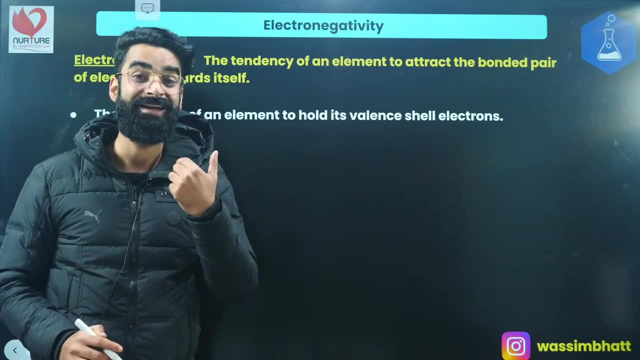 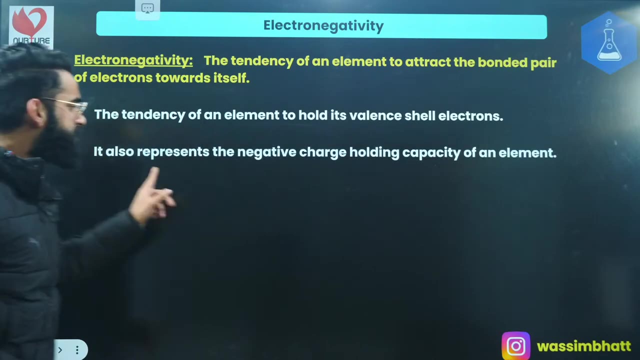 this is one more thing which is really important, right? yes, the tendency of an element to hold its valence shell electrons, right, more electronegativity element, its tendency will be more to hold its valence electrons. yeah, one more way. one more thing: it also represents the negative charge. 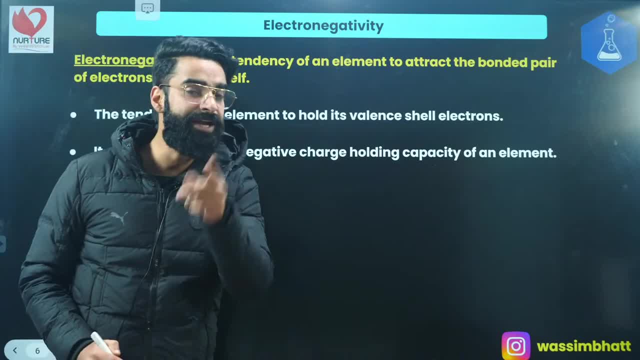 holding capacity of an element. more. the electro negativity of an element equals to more glandular metalization. right, regardless of which elementalians present there isぎ मेberry gì κuse? more will be the tendency of the element to hold the negative charge to sustain. 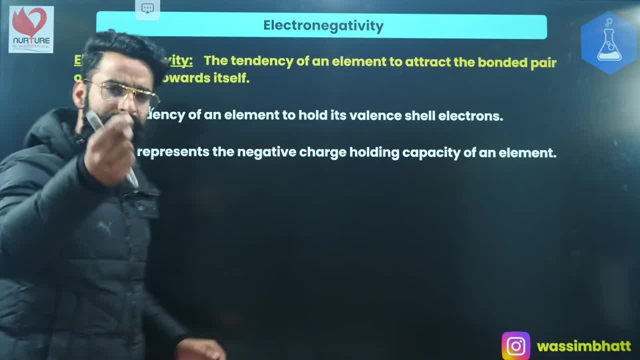 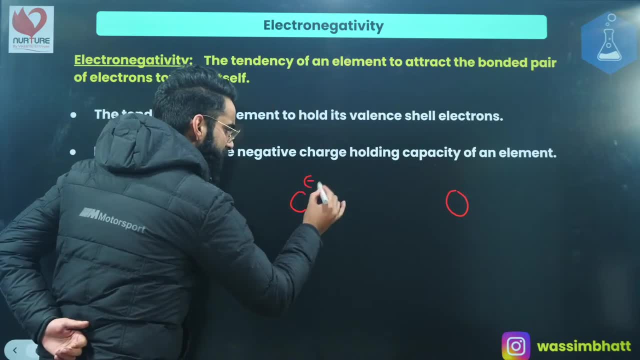 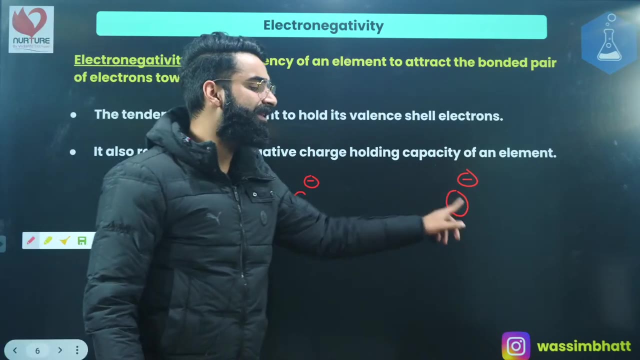 the negative charge to sustain the negative charge. what does that mean? for example, let's say I've got an element carbon over here I've got the element oxygen. let's say there's a negative charge on this carbon. let's say there's a negative charge on this oxygen, right, yes, if I ask you, where will be the? 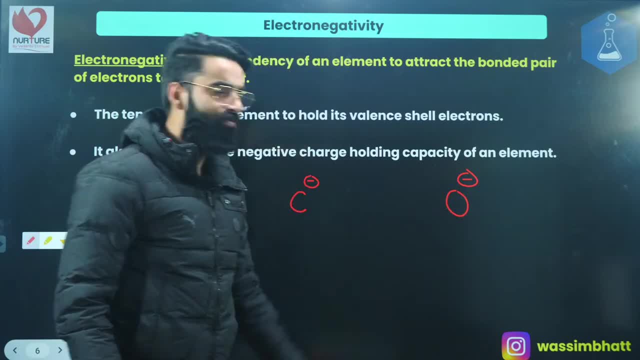 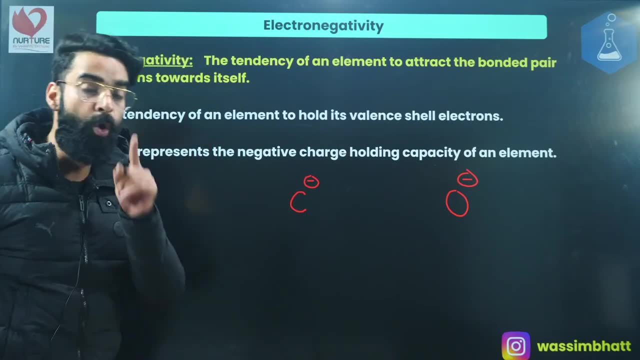 negative charge more stable? if I ask one these two, where will be the negative charge more stable? is it more stable in oxygen or more stable on carbon? as I told you, more electronegative element has got more tendency to hold the negative charge on it, right? yes, 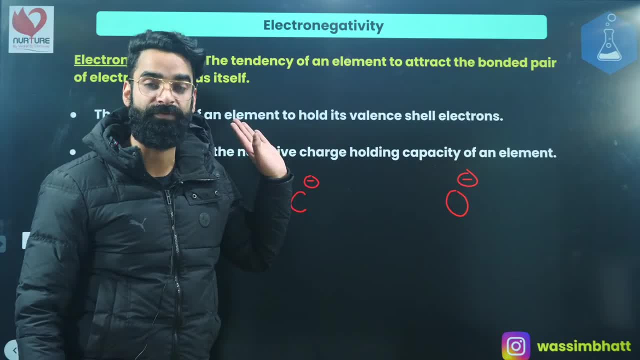 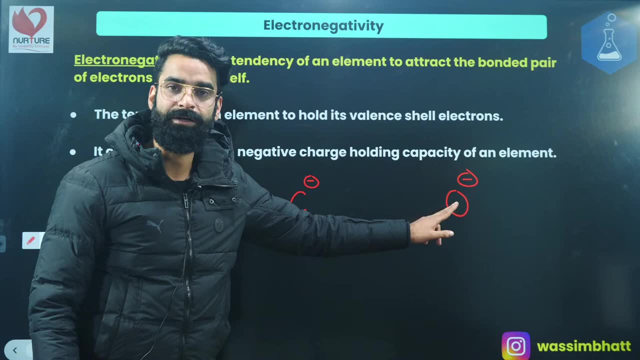 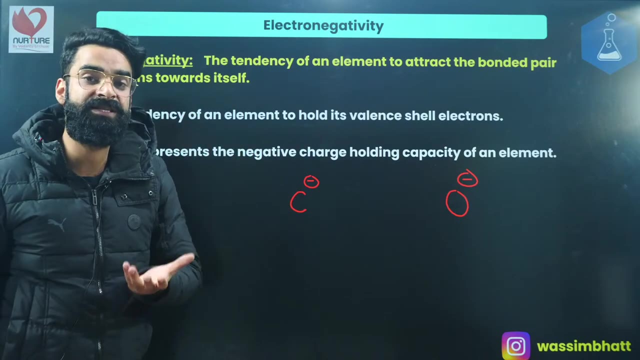 electronegativity it represents the negative charge, holding capacity of an element. yes, right, oxygen being more electronegative, oxygen being more electronegative, it will be having more tendency. it will be having more tendency to hold the negative charge and more the tendency of an. 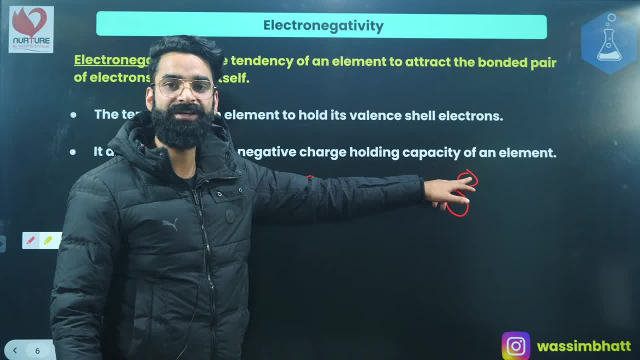 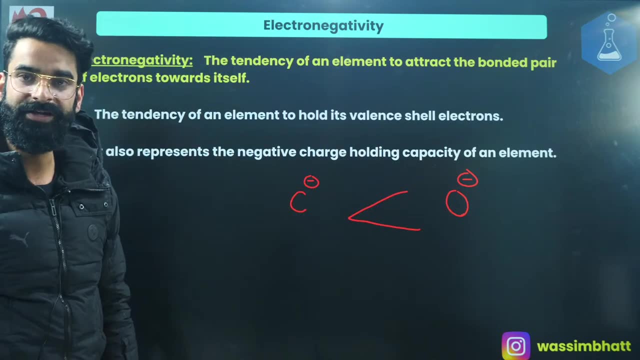 element to hold the negative charge. more is very the stability of the charge at that point of time. so where is the negative charge more stable? you will say negative charge is more stable on oxygen as compared to carbon. right as simple as that. so electronegativity first of all it gives us. 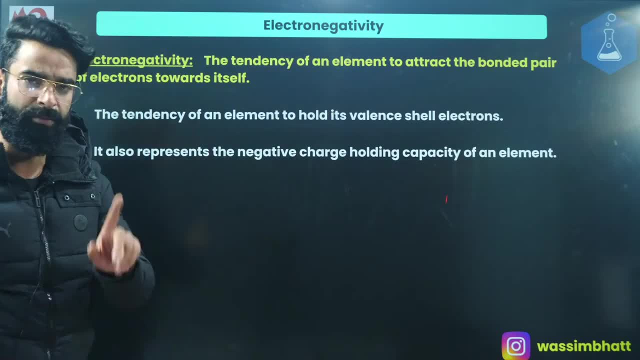 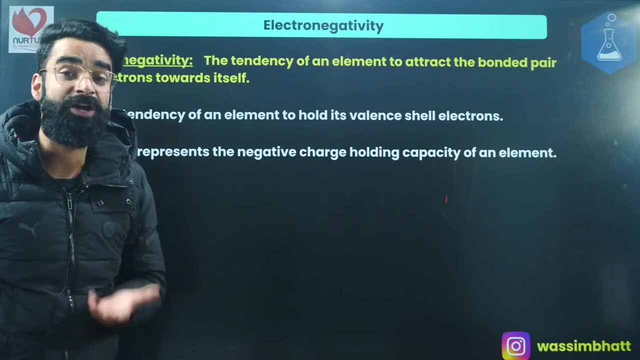 the tendency of an element to attract the bonded pair of electron towards itself. number one. number two: it gives us the tendency of an element to hold its valential electrons. number three: it represents the negative charge holding capacity of an element. more electronegative element has. 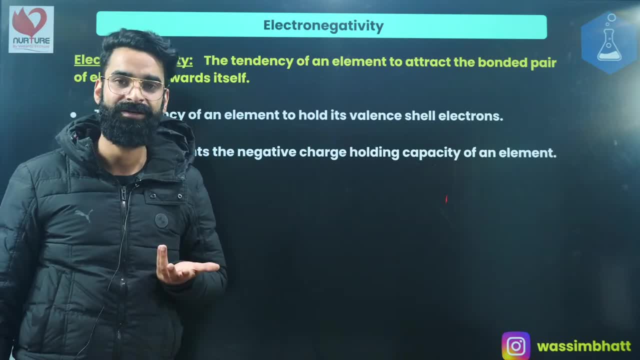 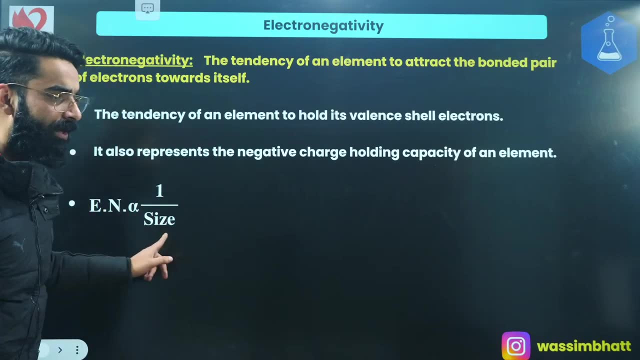 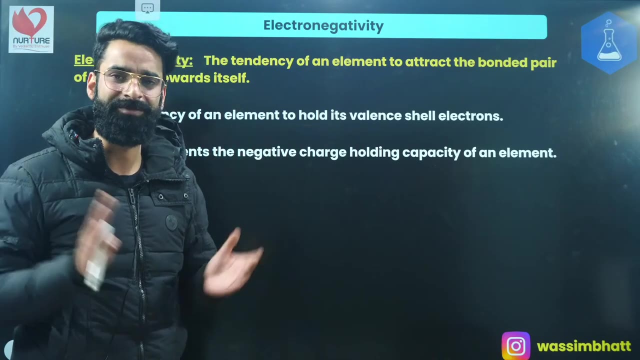 got more tendency to hold the negative charge right. yes, I'm sure this is clear till here, right? this is something which you would have studied in chemical bonding. what is it? electronegativity is inversely proportional to size. lesser the size of the element, definitely more is going to be its. 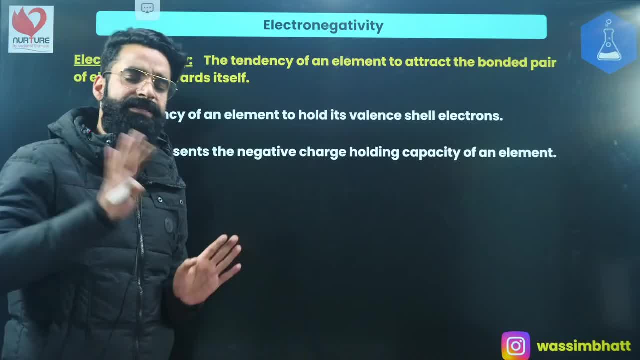 electronegativity. more the size of the element, less is going to be its electronegativity. you all must be familiar with the fact. on the other hand, if you have an element which is electronegative in a periodic table- because that is where the rate of like, if the value of the element is- 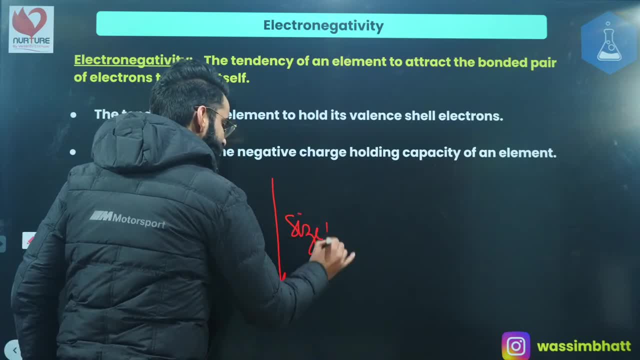 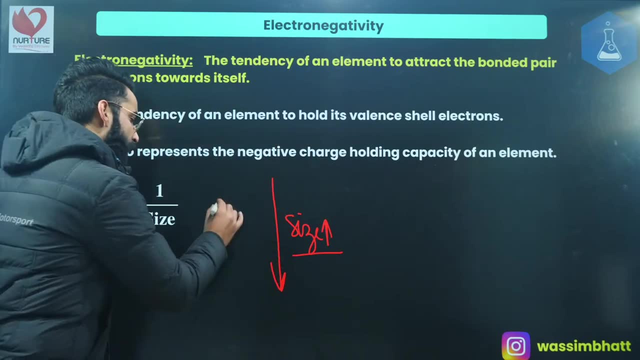 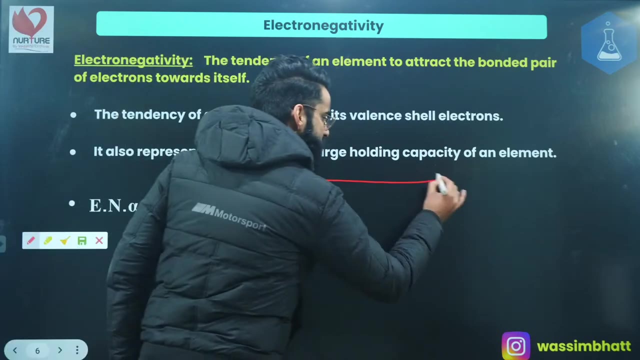 смерed. but if the value of the element is something like this: the weight of the element is reducing or moving from top to bottom in the periodic table, what happens to the atomic size generally? generally it increase. if the atomic size increases generally on going from top to bottom, so on moving from top to bottom, what will be happening to the electronegativity? 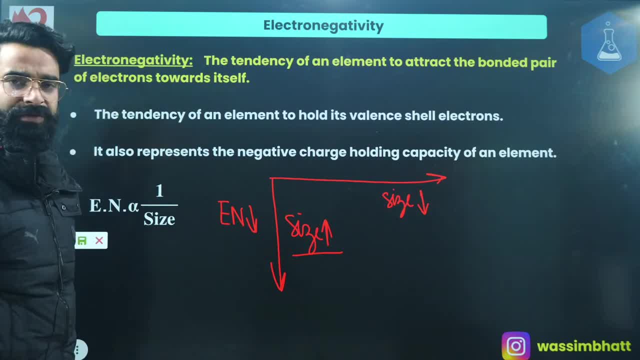 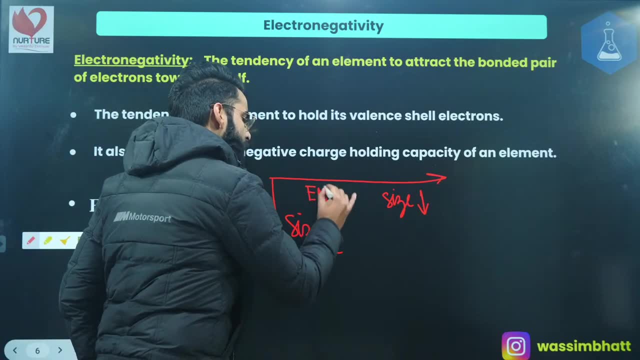 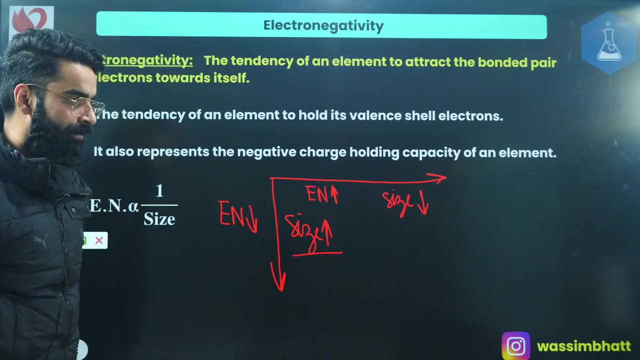 of the elements. it will be decreasing because both are inversely proportional to each other. on going from left to right, what happens to the size electronegativity of the elements will increase on moving from left to right. as simple as that, right? yes, I'm sure this is clear to everyone, right, people? so I'm 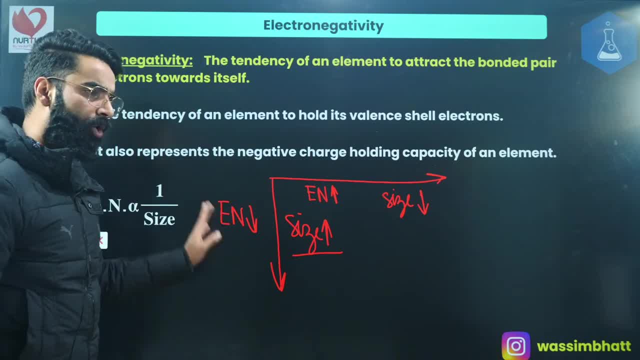 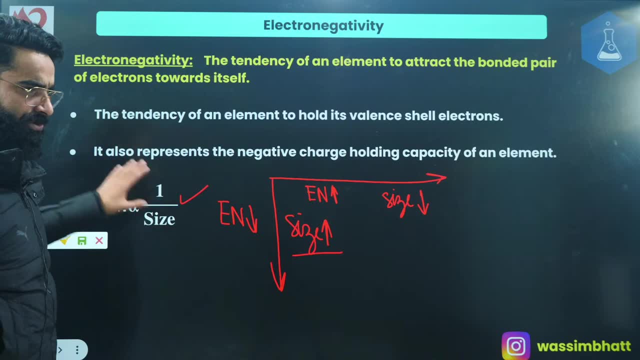 going from top to bottom, size increases. electronegativity decreases on moving from left to right. generally, size decreases, so electronegativity of the elements increases. so do remember this thing as well. there's something, really basics, which you would have studied in chemical bonding as well, right, yes, 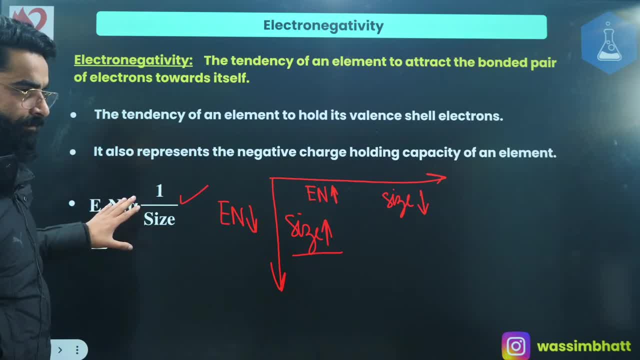 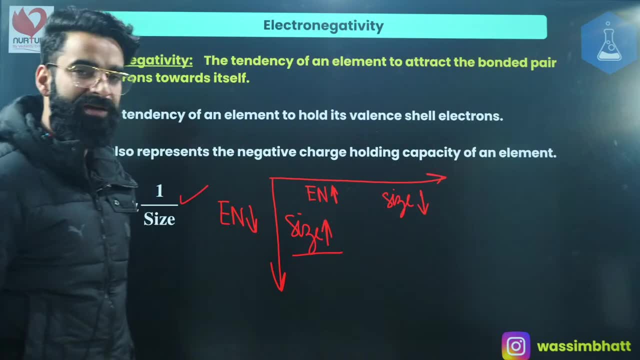 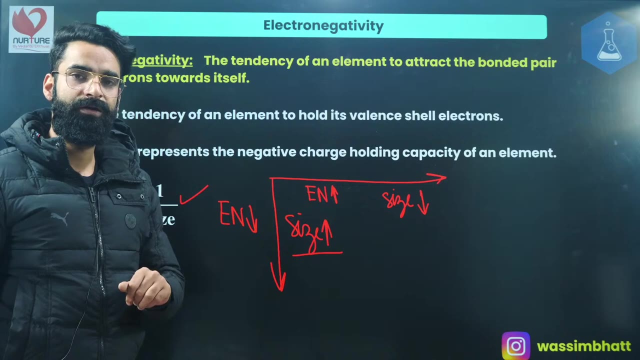 perfect. someone is saying how electron affinity of chlorine is high. bro, you check chemical bonding sessions of mine. you will get to know exactly why electron affinity of chlorine is more than the fluorine in the similar way, in the similar way, why electron affinity of sulfur is more than that of oxygen. you 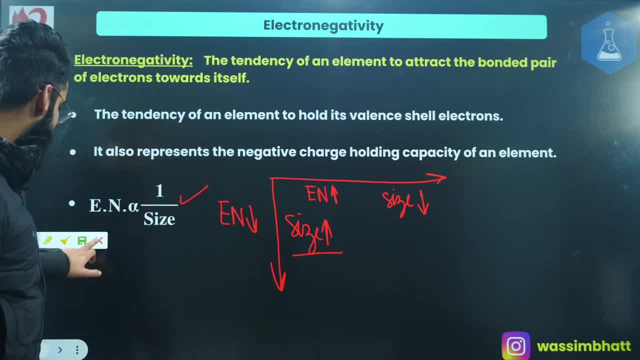 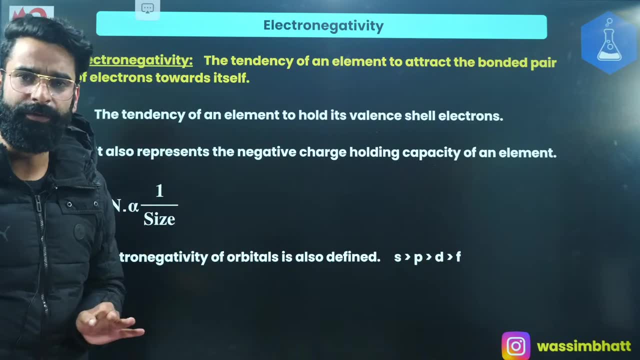 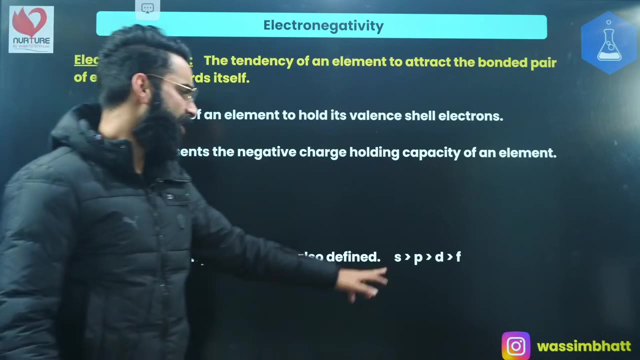 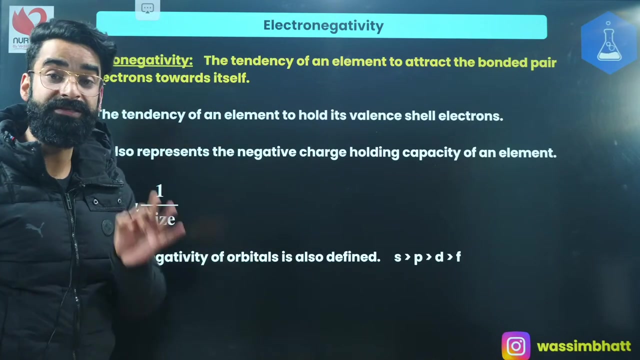 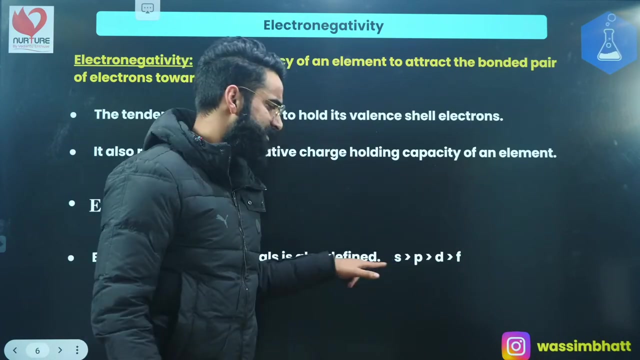 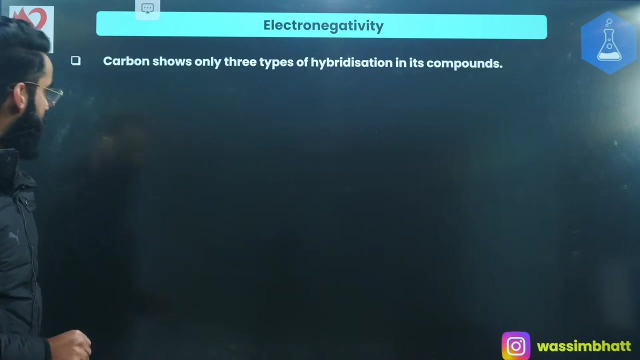 will get the idea in chemical bonding. this is GOC currently going on right, let's not divert the topic. yes, okay, let me tell you- you have a look- what I'm going to talk about- something really interesting. have a look, guys. first of all, let me tell you 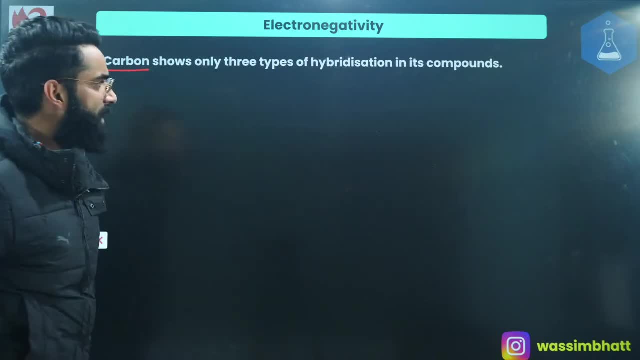 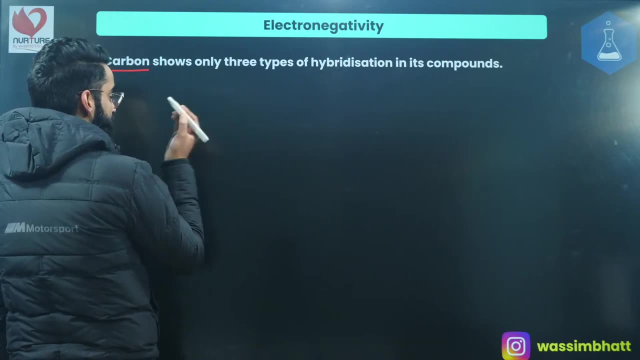 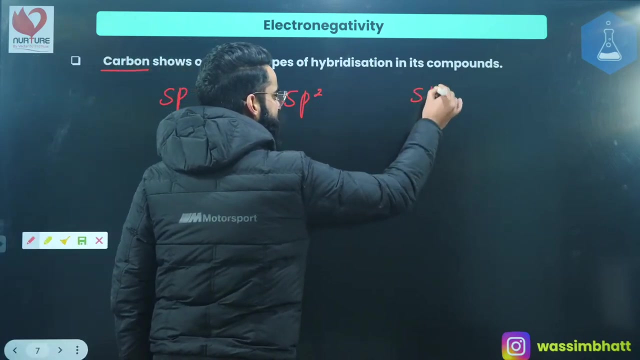 whenever you talk about carbon, whenever you talk about carbon, carbon generally shows three types of hybridization. it only shows three types of hybridizations. carbon only shows three types of hybridizations: sp or sp2 or sp3. these are the three types of hybridizations which carbon shows right. 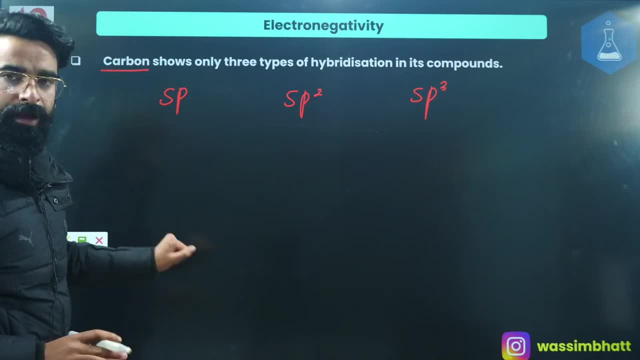 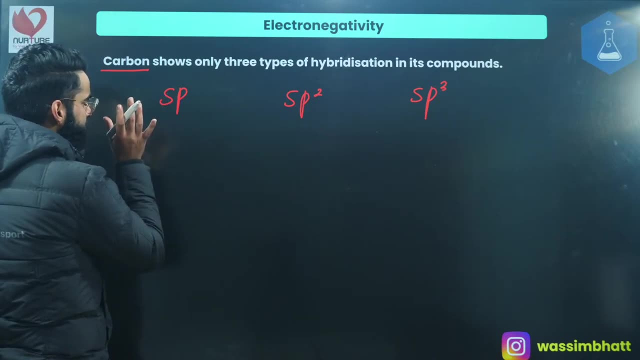 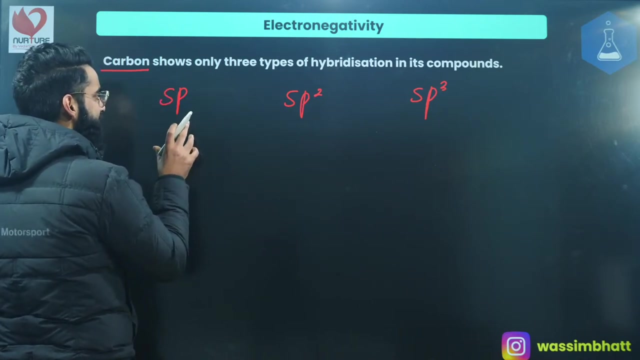 sp, sp2, sp3. right, okay, in case of sp hybridization, what happens? what happens, basically, in case of sp hybridization, one of the s orbital and one of the p orbital in carbon intermixes and leads to the formation of two hybrid orbitals. right, and these are the two hybrid orbitals: one, this is one more, these are: 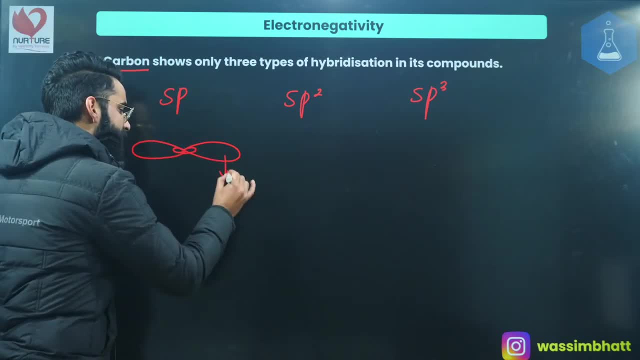 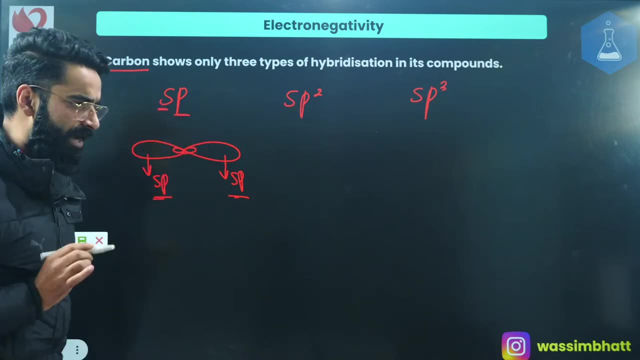 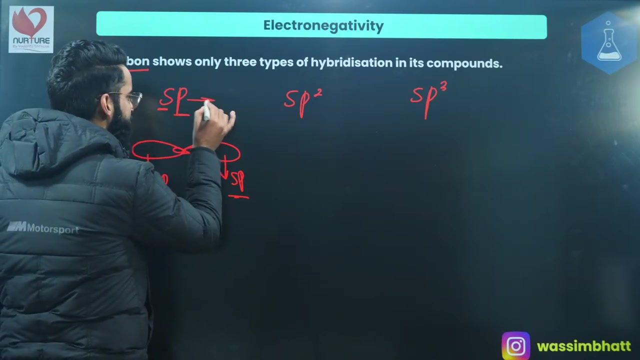 the two hybrid orbitals. right, this is what I call as sp hybrid orbital. this is what I call as sp hybrid orbital. right? number of atomic orbitals mixing is always equal to the number of hybrid orbitals formed. yes, right. first of all, what is going to be the bond angle in case of sp hybridization, if you remember? 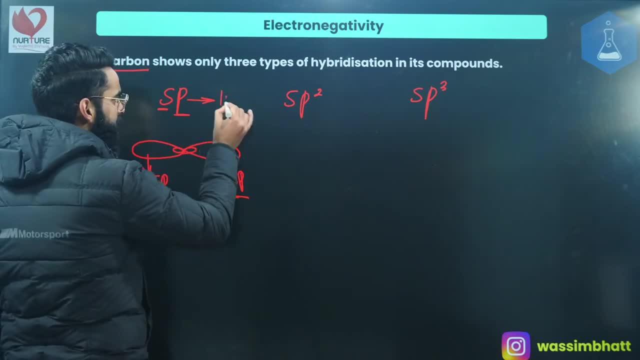 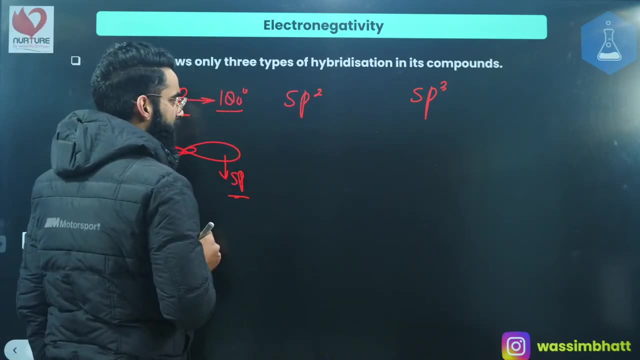 in case of sp hybridization, the bond angle. since it's going to be linear, its bond angle is going to be 180 degree. right, if I talk about sp2 hybridization in carbon, whenever I'll be having the carbon undergoing sp2 hybridization and that means one of the s orbital of carbon. 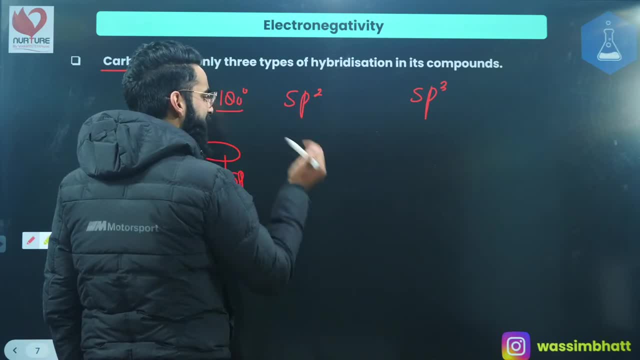 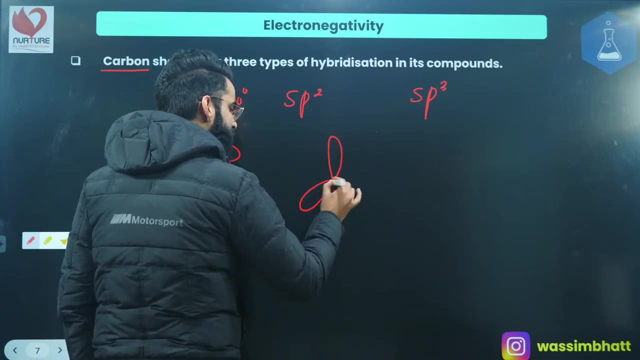 carbon and two of its p orbitals. they have intermixed and they have formed three hybrid orbitals. right, Let me arrange those hybrid orbitals in such a way that there are minimum repulsions between them. These are the three hybrid orbitals which I've arranged right. 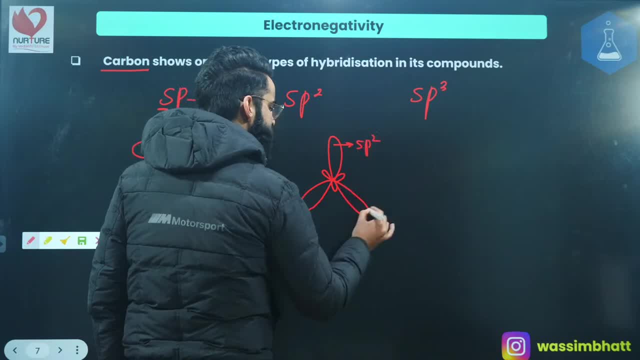 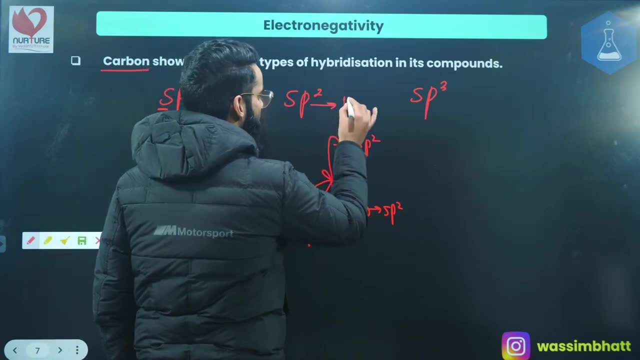 This is what I'll be calling as sp2 hybrid orbital. even this is your sp2 hybrid orbital. even this is your sp2 hybrid orbital, right? What is going to be the angle in case of sp2 hybrid? It's 120 degree, right? This is something which you would have studied as well in chemical. 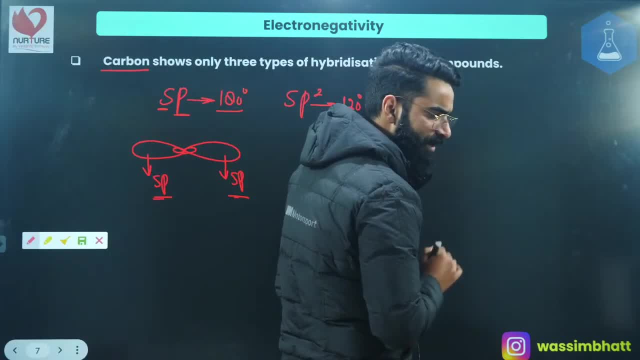 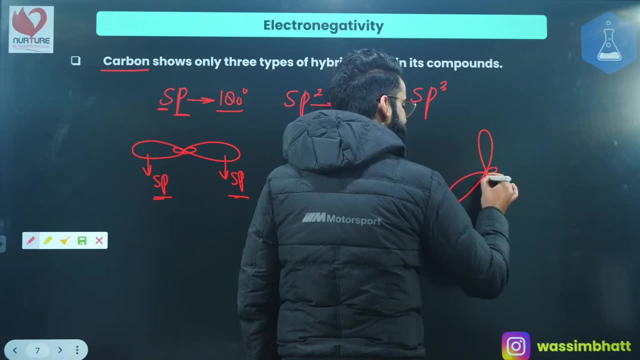 bonding, yeah. Similarly, if you talk about sp3 hybridization, my dear people, in case of sp3 hybridization, we'll be having four. we'll be having four sp3 hybrid orbitals arranged in such a way that there will be minimum repulsions between them. and what is the bond angle in this case? 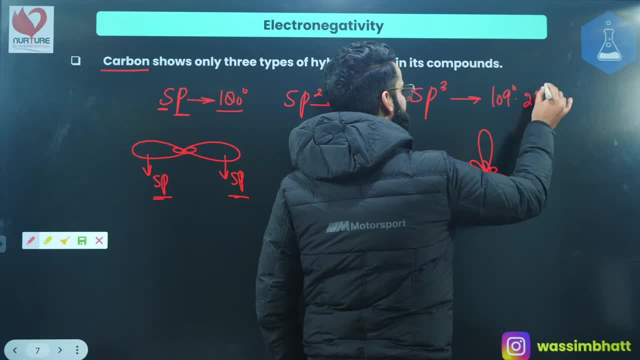 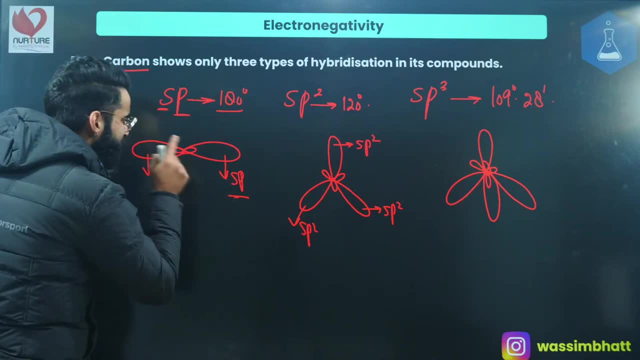 it is 109 degree 28 minutes. Every one of you will be knowing this right. 109 degree, 28 minutes, right. If I ask you, what is the see? this is the hybrid orbital. this is sp2. hybrid orbital, right. So if I ask you, what is the see? this is the hybrid orbital, this is sp2. 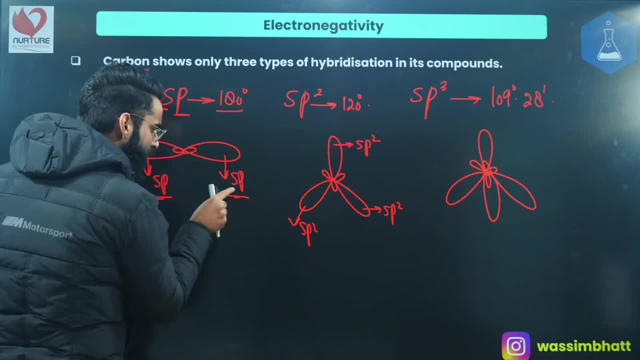 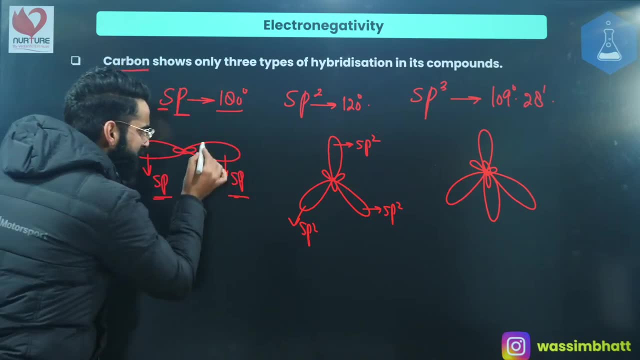 sp hybrid orbital. This hybrid orbital has got formed when one of the s orbital and one of the p orbital, when they have intermixed and formed this hybrid orbital right. So in this hybrid orbital there will be some percentage of s character. there will be some. 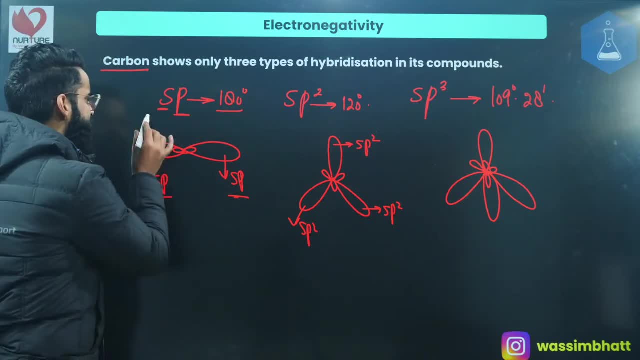 percentage of p character as well. If I ask you, in case of sp hybridization, what is the percentage of s character? What is the percentage of s character? How many s orbitals are involved in in this intermixing? One s orbital is involved. How many total orbitals are involved? 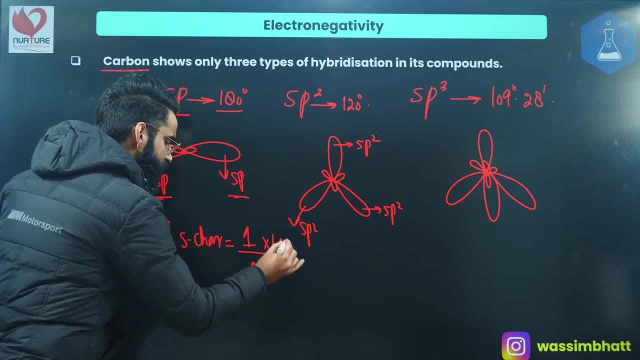 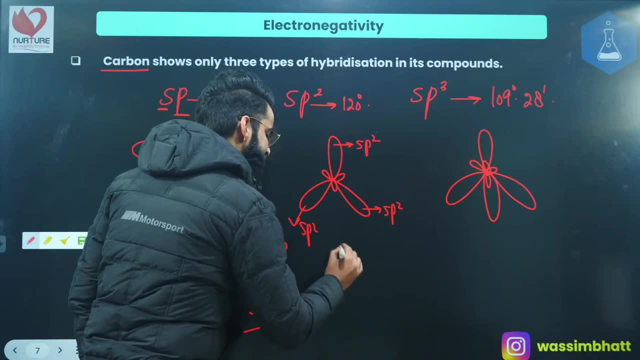 in this intermixing Two orbitals multiplied by 100.. So percentage of s character in case of sp hybridization is going to be 50, right? If I ask you what is going to be the percentage of s character in case of what? In case of sp2 hybridization, How many s orbitals have? 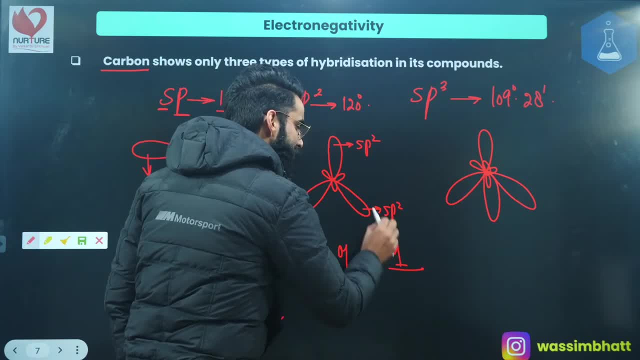 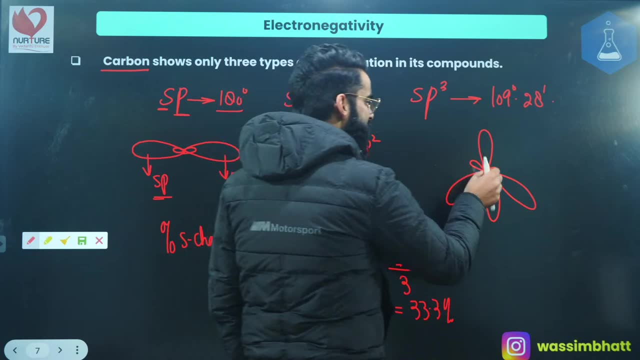 participated in the intermixing One. How many total orbitals have participated? Three multiplied by 100. The value comes out to be 33.33 percent, right? Similarly, if I talk about the percentage of s character over here in sp3 hybridization. 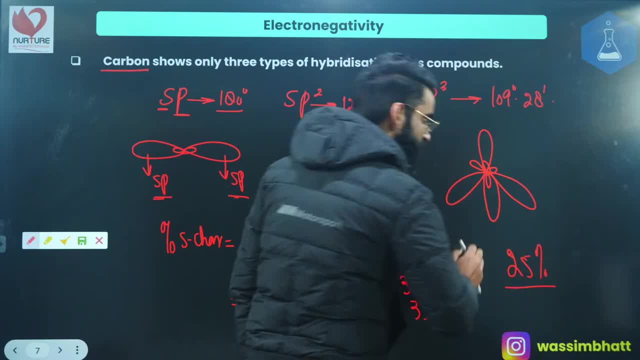 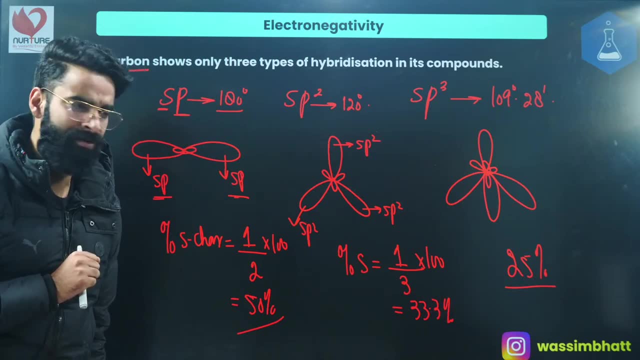 you can calculate it, It will come out to be 25 percent. It will come out to be 25 percent. I told you few minutes back, electronegativity is defined for s orbitals as well, Do you remember? Yes, I mean, electronegativity is defined for orbitals as well. S orbitals have maximum. 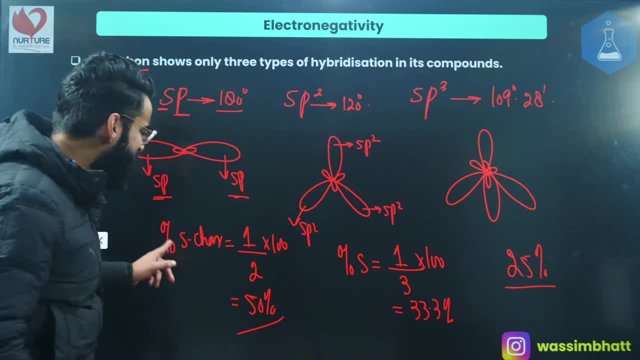 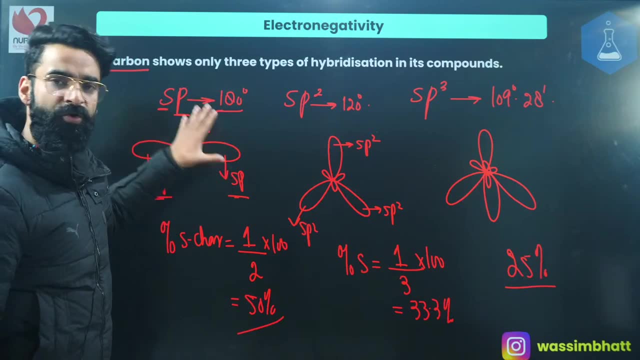 electronegativity, followed by p, followed by d, followed by f. Where is the maximum percentage of s character? In the first one there is a maximum percentage of s character. So can I say: wherever percentage of s character is more, there only electronegativity will. 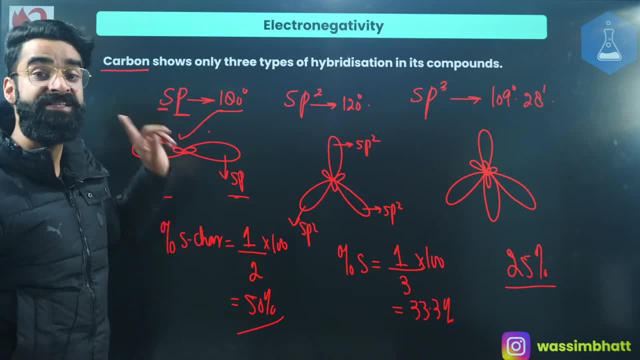 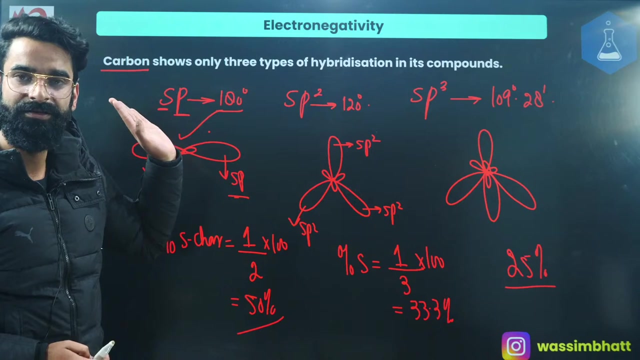 be more. Yes, So can I say electronegativity is defined for hybrid orbitals as well. right, Because of more s character in sp hybrid orbital, its electronegativity will be more than that of sp2,, more than that of sp3, right? Yes, Electronegativity in case of sp is going to. 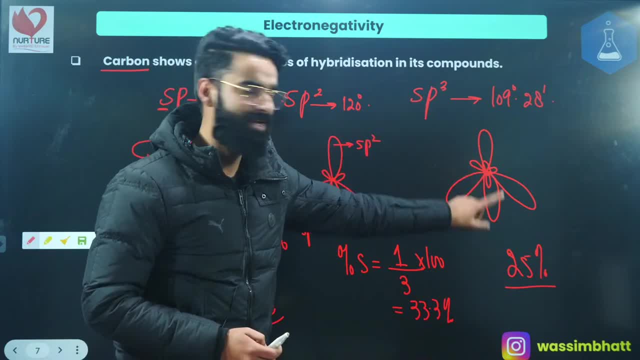 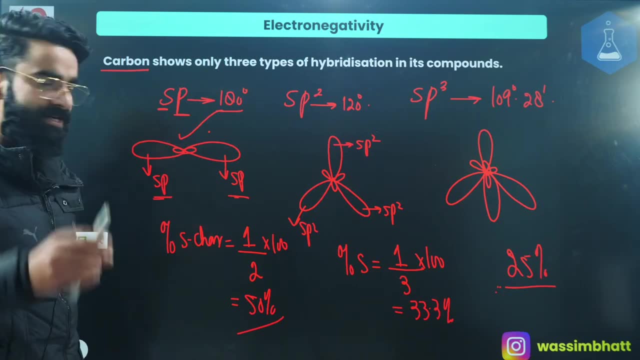 be more than that of sp2, is going to be more than that of sp3, right? Yes, Electronegativity sp3.. This sp3, it has got the least s character. yeah, It has got the least s character, correct. 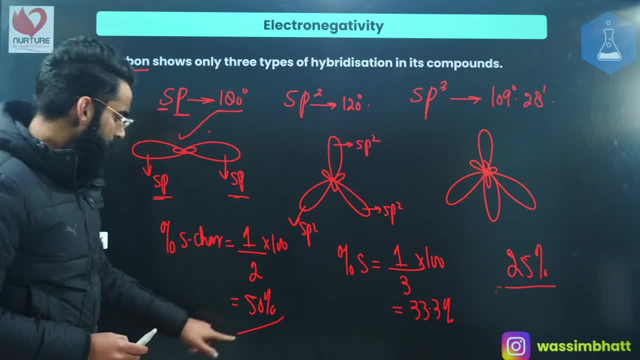 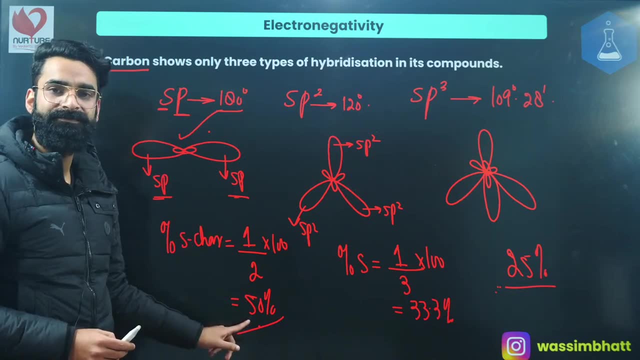 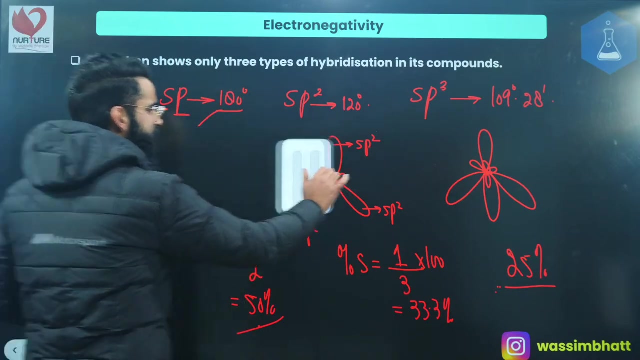 Understand 5 important things. Understand 5 important things. See, percentage s character is maximum over here, right? So electronegativity is maximum. Electronegativity is maximum, right. Yes. So if I ask you, if I say something like this, I'll say something like this first. 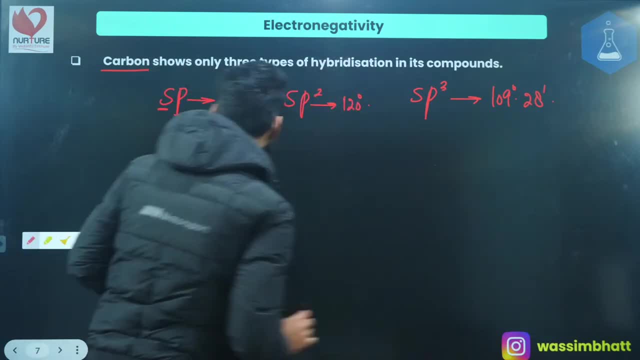 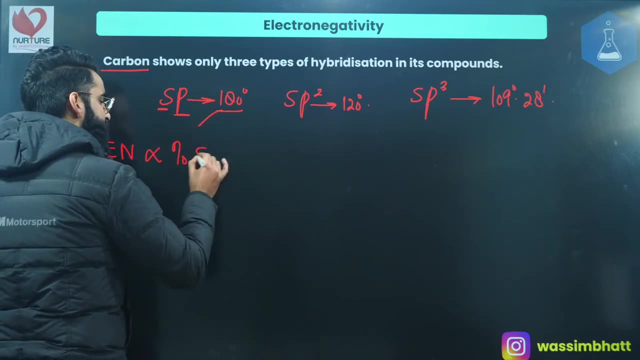 of all, I'm sure you would have taken a note of every single thing till here. right? I'm giving you a simple statement. A statement is electronegativity. it is directly proportional to the percentage of s character. It is directly proportional to the percentage of s character. 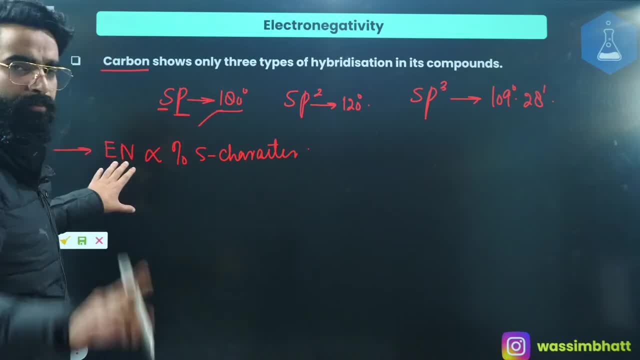 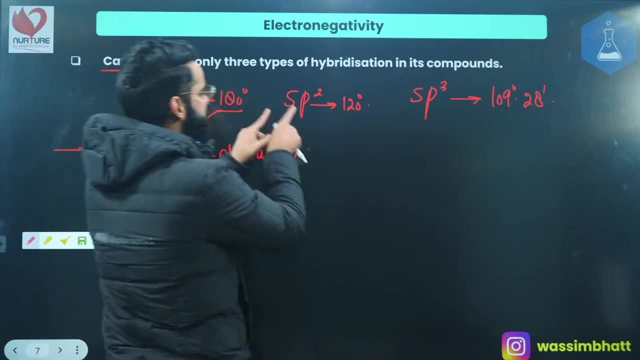 right: More percentage of s character, more the electronegativity. Point number one, Point number two, As I am moving from left to right. have a look, This is sp, As I am moving from sp towards sp2, towards sp3, right, What is happening with the percentage of s character? 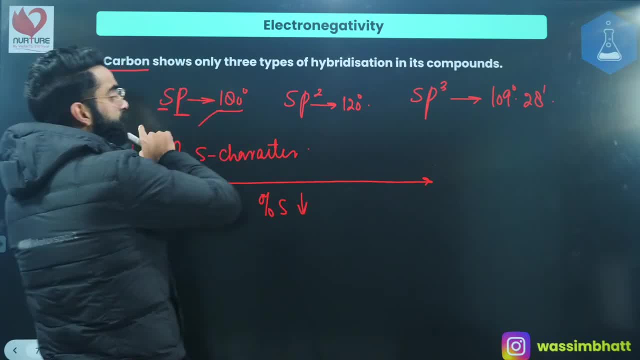 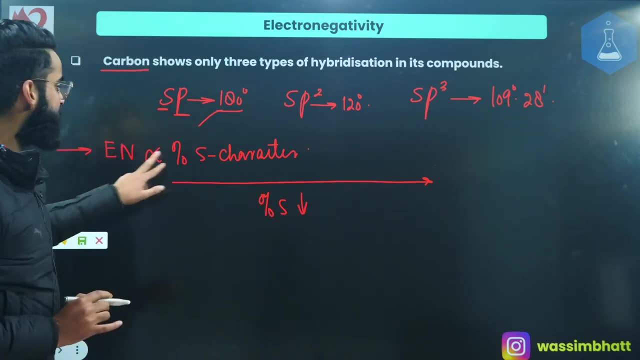 Percentage of s character is decreasing. As I am moving from sp to sp2, I am decreasing. Percentage of s character is decreasing. What is happening to the electronegativity? Both are directly proportional. If percentage of s character is decreasing, I must say electronegativity. 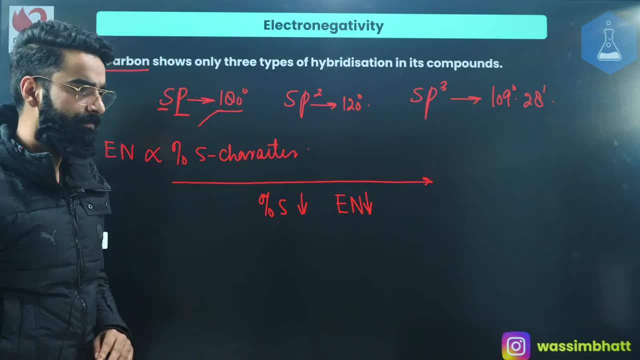 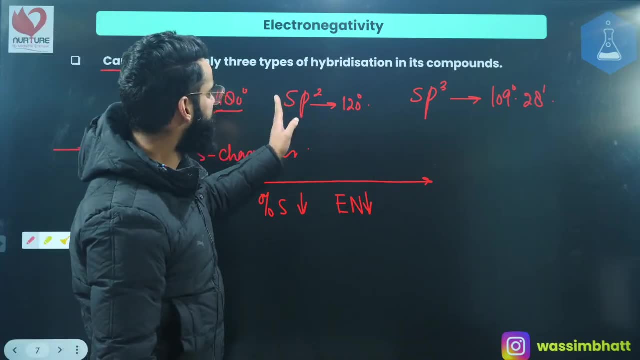 is decreasing right. Electronegativity is decreasing right. Yes, Medico, it's lying At the same time on moving from sp to sp2, right To sp2 to sp3.. What is happening to the bond angle? Is the bond angle increasing or decreasing? 180, 120, 120, 120? What is? 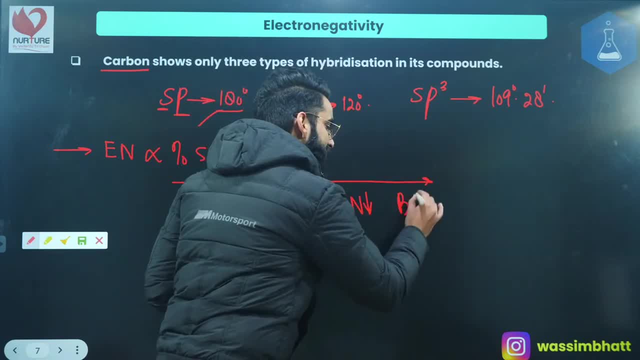 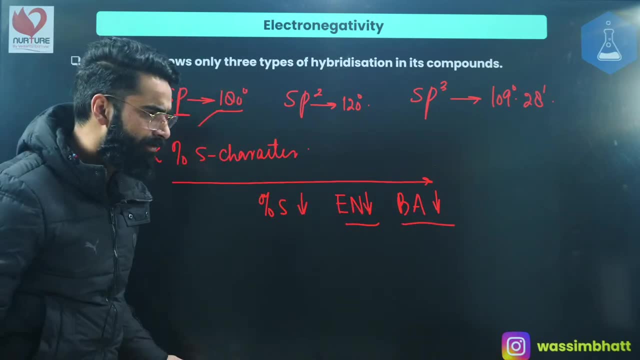 120, 109,. bond angle is decreasing. yes, bond angle is decreasing. So can you make a direct result between electronegativity and bond angle? absolutely, you can make a direct result between electronegativity and the bond angle, right? yes, both are showing. 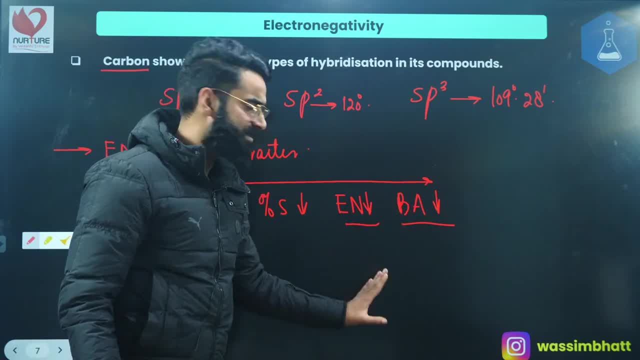 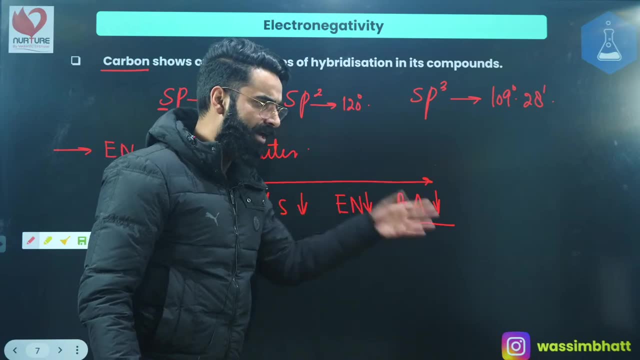 the same variation. both are showing the same variation. can I simply say bond angle is directly proportional to electronegativity. lesser the electronegativity, lesser the bond angle. more the electronegativity, more is going to be the bond angle, right? so this: 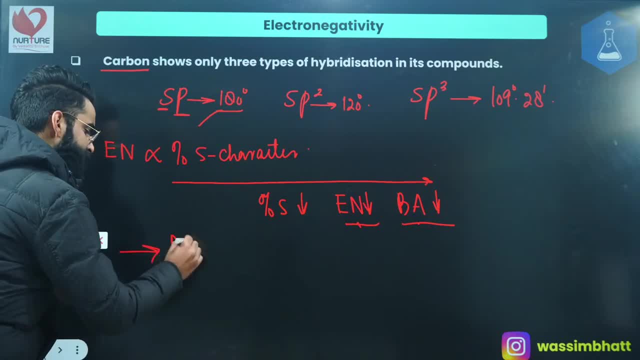 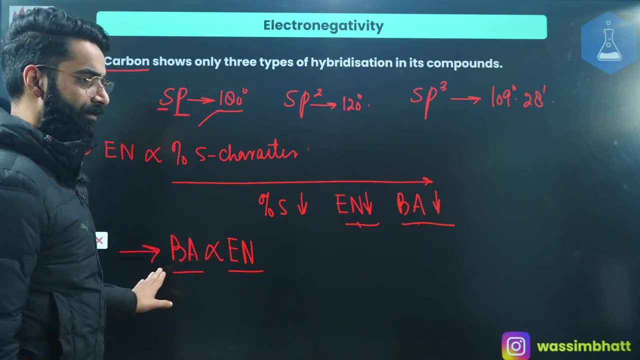 is one important statement which you need to take note of from now onwards, bond angle is directly proportional to electronegativity. more the bond angle, more the electronegativity, more the electronegativity, more the bond angle. yes, they are directly related. I'm 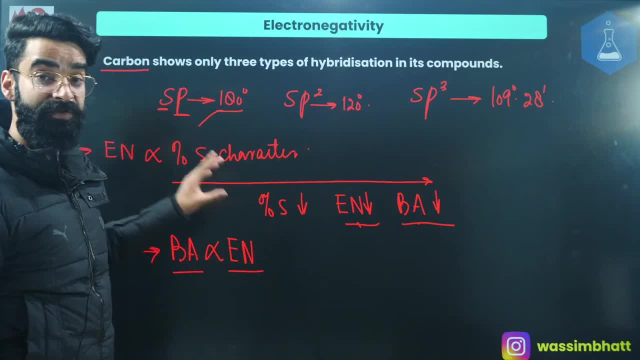 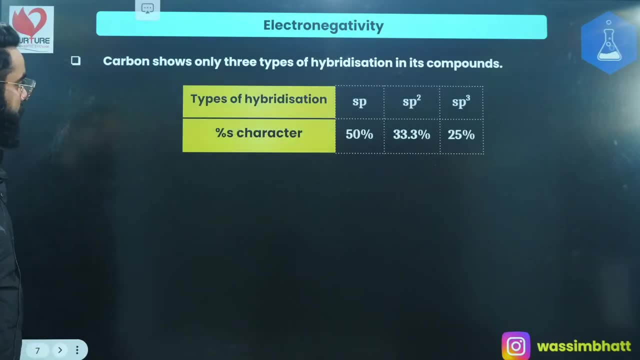 sure this is clear to everyone. yeah, these are important things which you need to take a note of, because I'll be using these things after few minutes. yeah, okay, So this is something which I've taught you. types of hybridization. 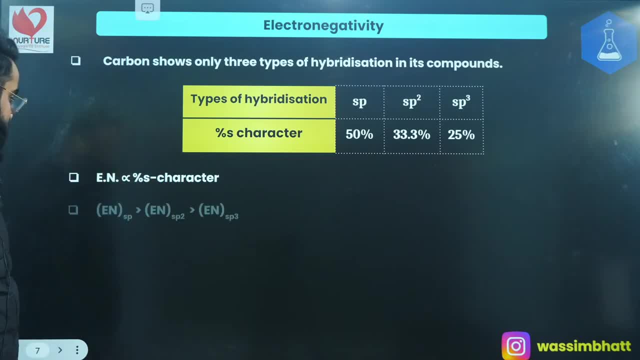 Personalization of S character electronegativity is directly proportional to personalization of S character electronegativity of SP hybrid orbital is more than that of SP2, more than that of SP3, this is something understood right Now. have a look exactly over here. have a look exactly over here. if you look at this, 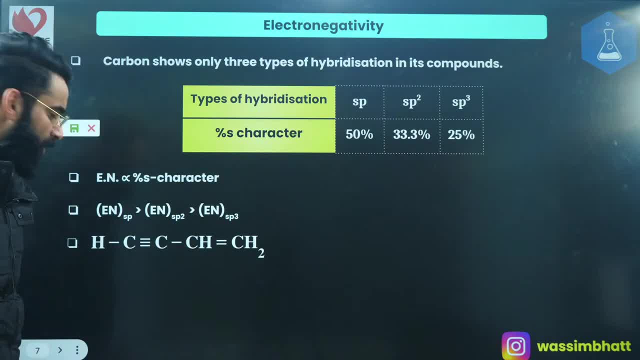 molecule. if you look at this molecule, understand properly, understand properly. if I ask you what about the hybridization of this carbon, You will be counting the number of sigma bonds. it's forming one sigma, two sigma. it's forming two sigma bonds. two sigma bonds means its steric number is two and its hybridization. 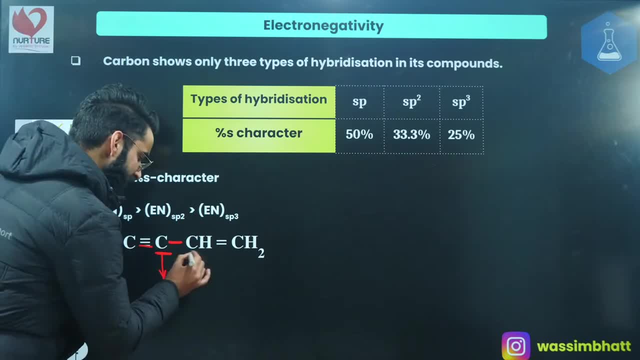 is SP right? If I ask you, what about the hybridization of this carbon? you will clearly count what. You will count the number of sigma bonds: one sigma, two sigma and there is one more sigma which this carbon has made with hydrogen. so three sigma bonds, steric number three: 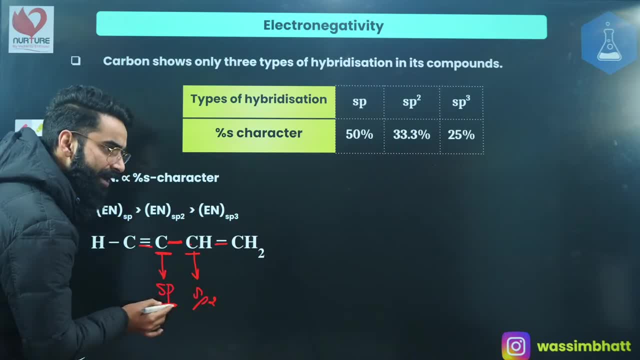 so SP2 hybridization: S character is more over here. S character is more over here. S character is less comparatively over here. More the S character, More the electronegativity. so electronegativity of this carbon is more electronegativity of 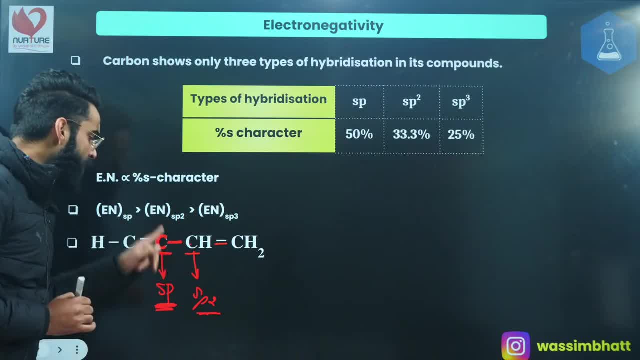 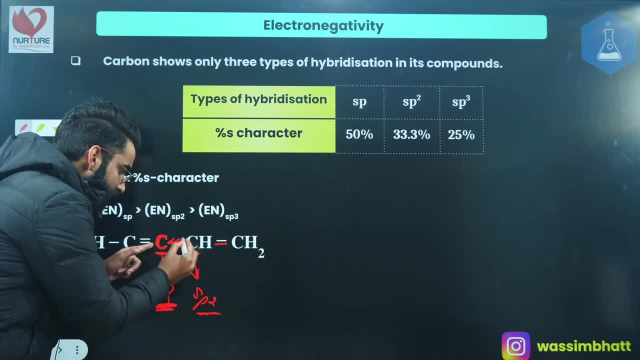 this carbon is more right. If electronegativity of this carbon is more, that means this carbon has got more tendency to attract this bonded pair of electron towards itself. it has got more tendency to attract the bonded pair of electron towards itself, due to which electron density towards this. 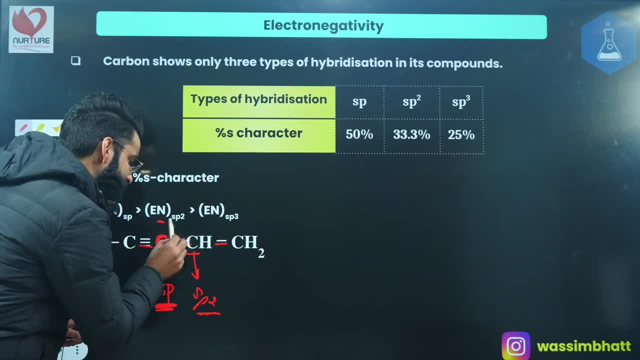 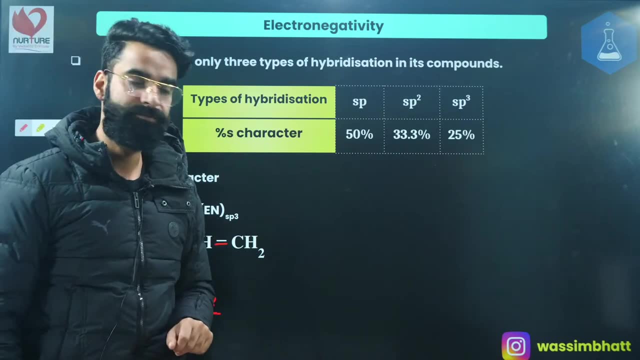 carbon would have got increased, and that increase in the electron density towards this carbon is represented by delta negative, and over here you will be getting delta positive, right. Yes, I am sure this is clear to everyone. very simple and basic thing, correct? 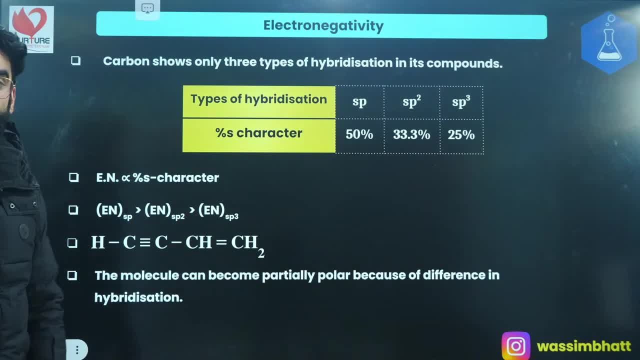 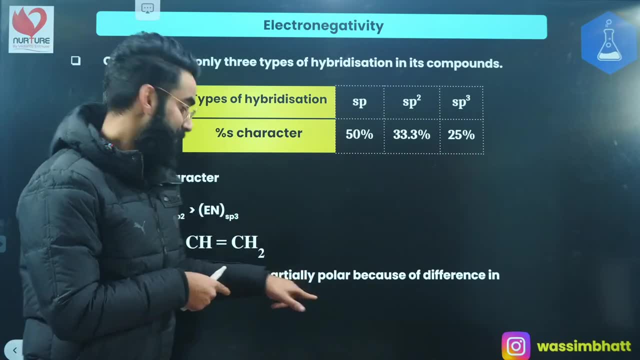 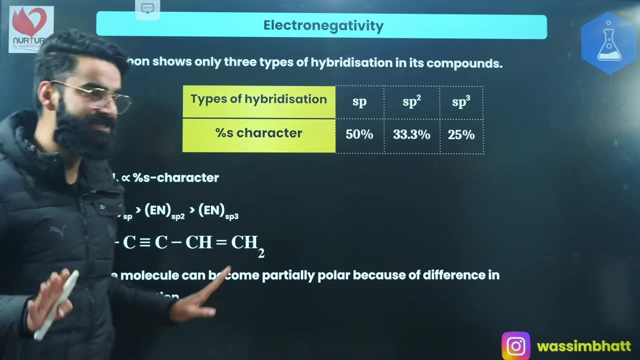 So from here, from here, I can generalize. one more statement. Can I say: the molecule can become partially polar, Like in this case. like in this case, the molecule can become partially polar because of the difference in the hybridization. as simple as that, right. 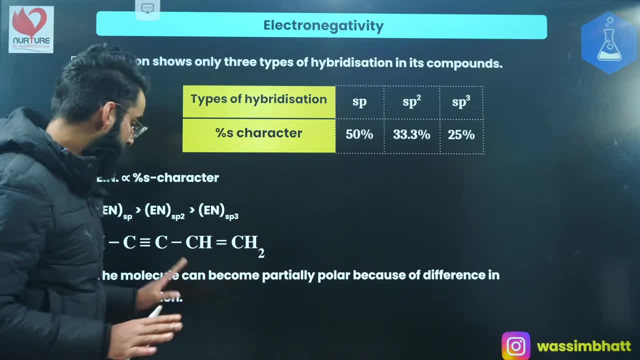 Can I say something like this? Absolutely, I can say, yeah, The molecule can become partially polar because of the difference in the hybridization. as simple as that. right, The molecule can become partially polar. it can become partially polar because of what? 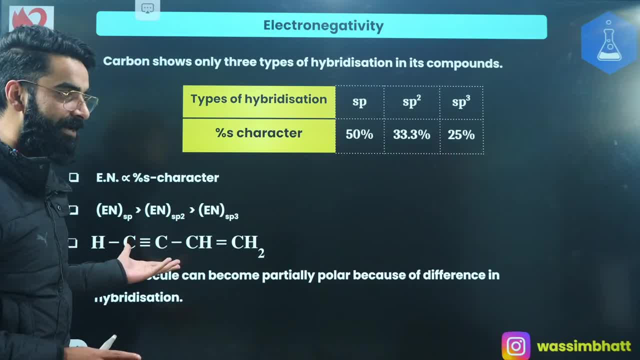 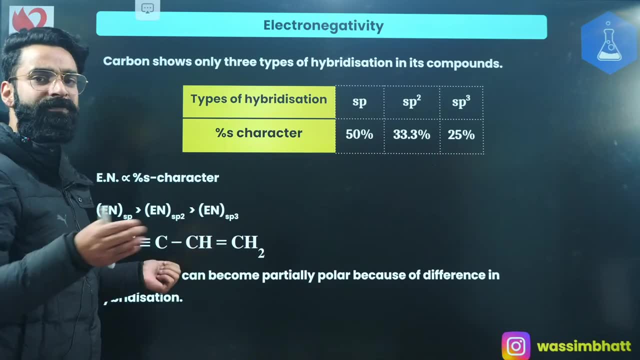 Because of difference in the hybridization, as you saw. as you saw, The molecule became partially polar because of the hybridization, because of the electronegativity difference, because of the shifting of the electron cloud towards more electronegative carbon right. 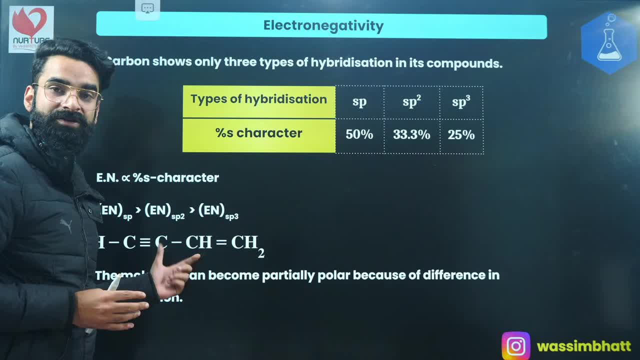 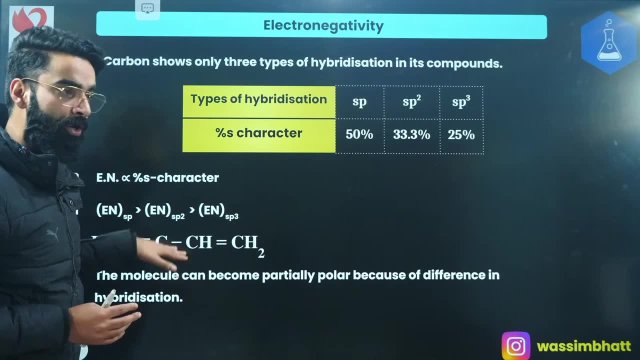 Due to which charges came on these carbon atoms. charges are coming on carbon atoms. that means polarity is getting induced in this molecule, right? So the molecule actually becomes partially polar. Partially polar because of the difference in the hybridization. I'm sure this is clear. 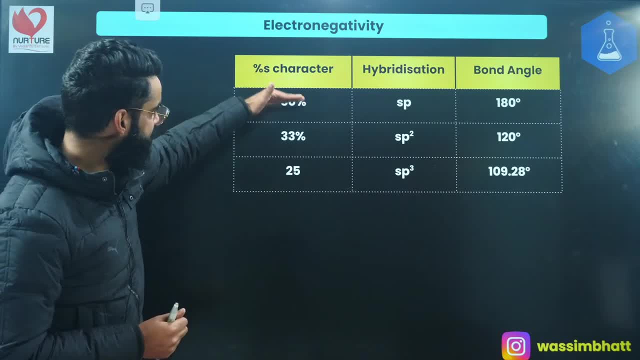 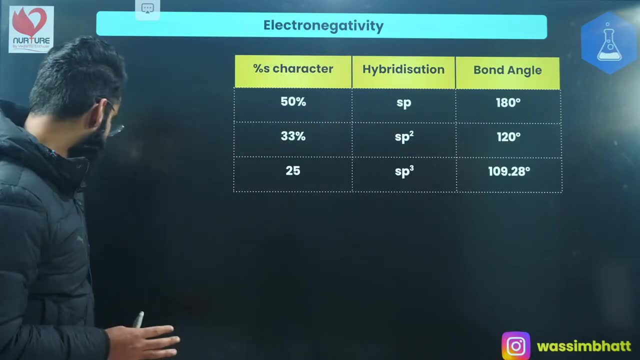 okay, This is something which I've told you. as the percentage S character decreases, what happens to bond angle? Bond angle also decreases. So bond angle and percentage S character- these are directly related. that's something which I've told you few minutes back. 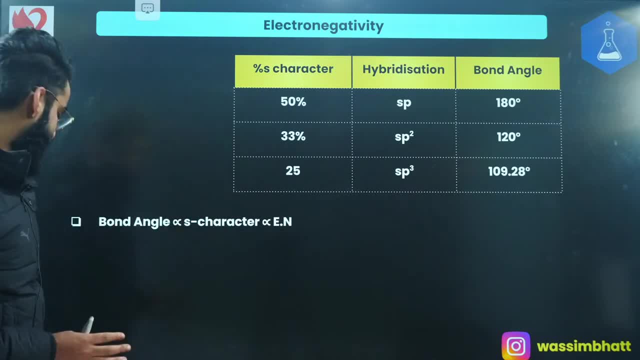 Bond angle is directly proportional to percentage S character, which is directly proportional to electronegativity as well. okay, Yes, there is one more important point: Positive charge on an electronegative element. Positive charge on an electronegative element. 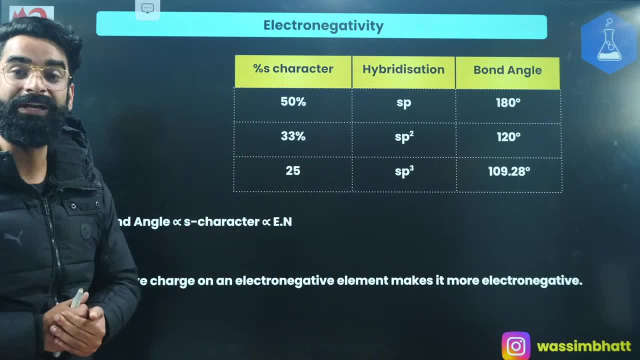 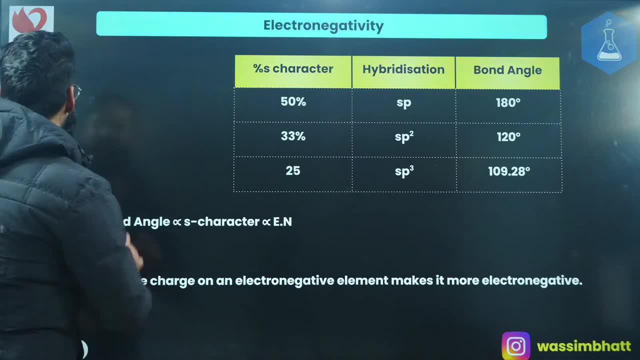 Positive charge on an electronegative element makes it more electronegative. Positive charge on an electronegative element makes it more electronegative. Why is that? Have a look. Let's say I've got the atom A. Let's say I've got the atom A, for example. okay, 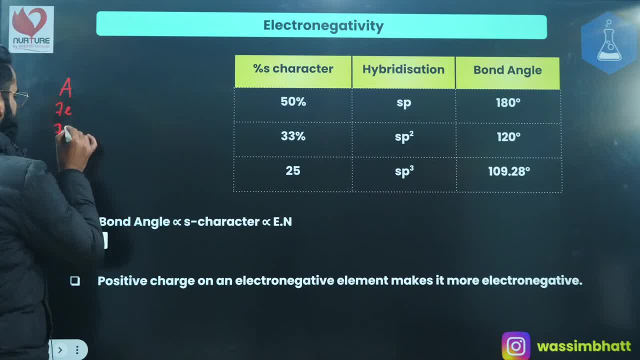 Let's say this atom A has got some seven electrons. it has got some seven protons, correct? Now I'm taking one electron out from this A, so it is getting converted into A positive. So in this A positive, how many electrons will be there? 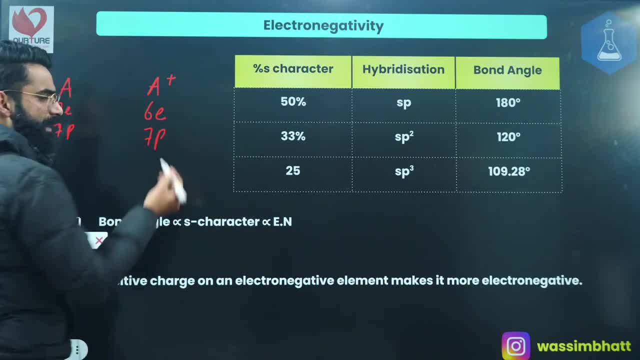 Six electrons, But I've done nothing with the proton. There will be seven protons over here as well. correct? yes, This is parent atom A. This is A positive. This is its ket I. correct, This is its ket I. 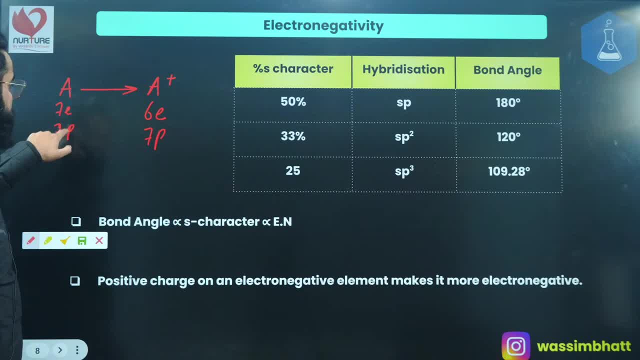 Over here you can see, seven protons were holding seven electrons. Seven protons were holding seven electrons. Over here, these, the same seven protons are only holding six electrons. right, Where do you think is the effective nuclear charge more? 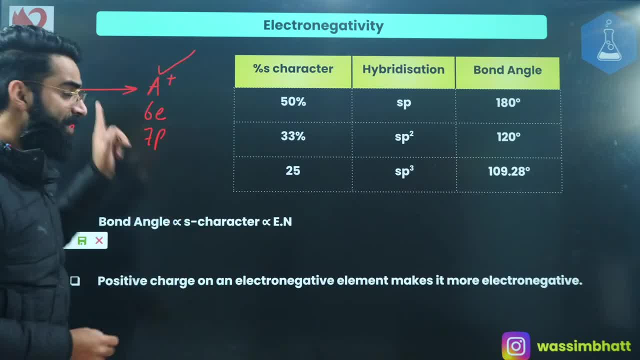 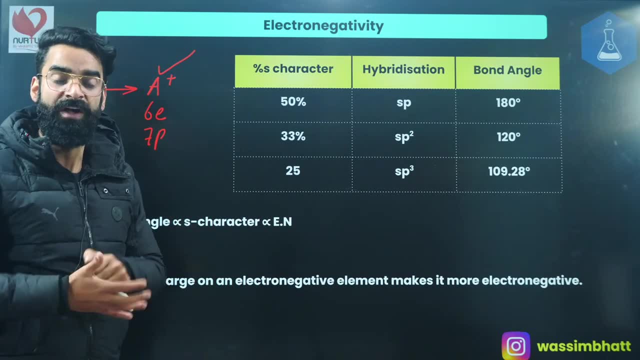 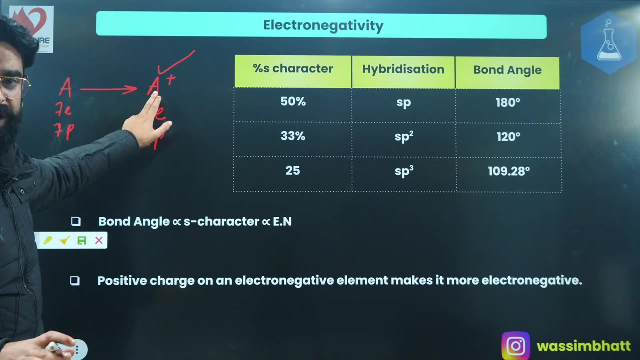 Can I say, effective nuclear charge is more. In this case, wherever effective nuclear charge is more, more is going to be its tendency to attract the bonded pair of electron towards itself. More is going to be its right, In short, in short, in short, can I say, more is going to be its electron negativity. 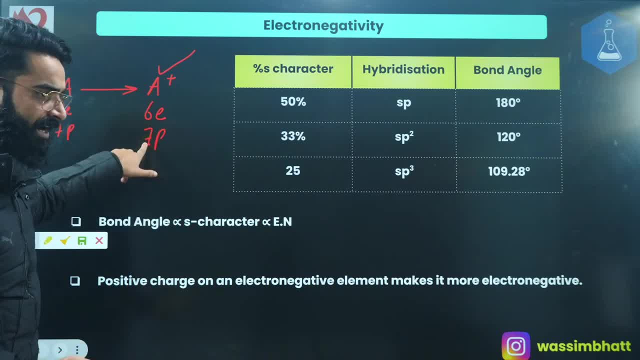 As simple as that. correct, Because only I mean the seven electrons, seven protons. they are holding only six electrons. right Over here, seven protons are holding seven electrons, correct? So effective nuclear charge is more in this case. 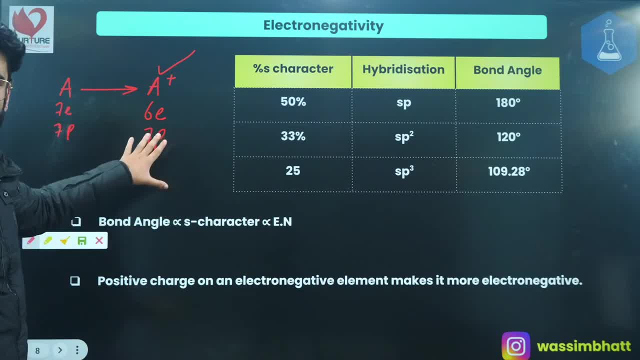 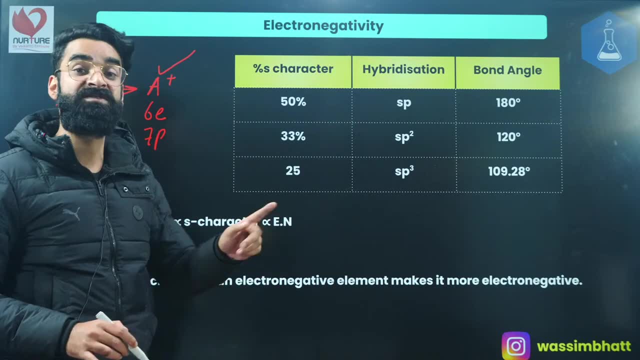 More is going to be its tendency to attract the bonded pair of electrons towards itself Right. In this case, more the effective nuclear charge, more is absolutely going to be its electron negativity correct. So whenever positive charge comes on an electro negative element, it becomes more electro negative. 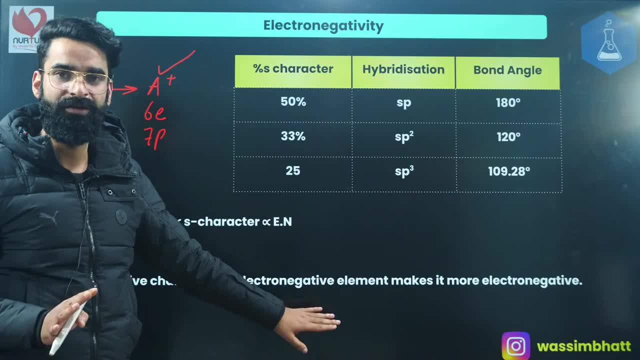 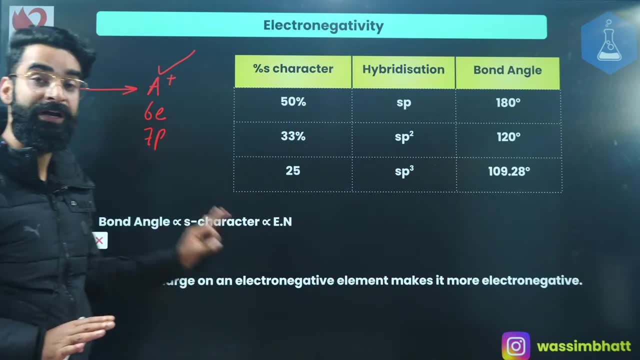 right, There's an exception as well, which I'll be telling you in some time. right, Where this rule gets failed, I'll be showing you that in some time, okay, So do remember: positive charge on an electro negative element makes it more electro negative. 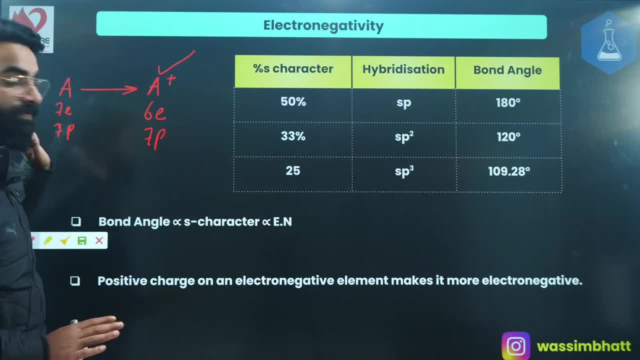 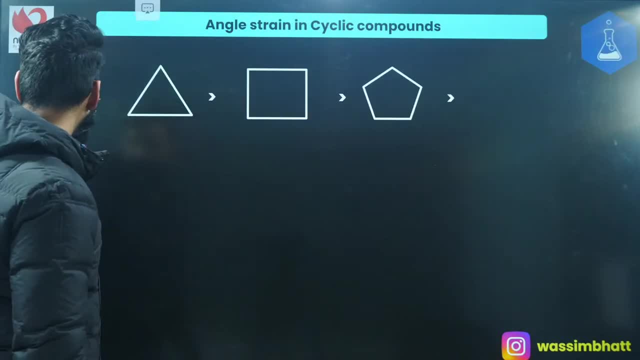 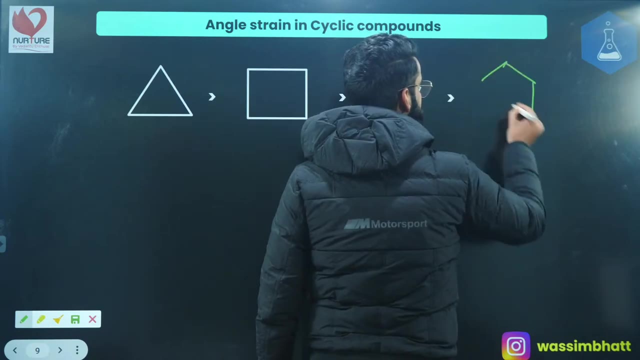 A positive will be definitely more electro negative than that of A. yeah, as simple as that. I'm sure this is clear, Perfect, Perfect. Now comes one more point. Now comes one more point. Have a look exactly what I'm going to talk about. 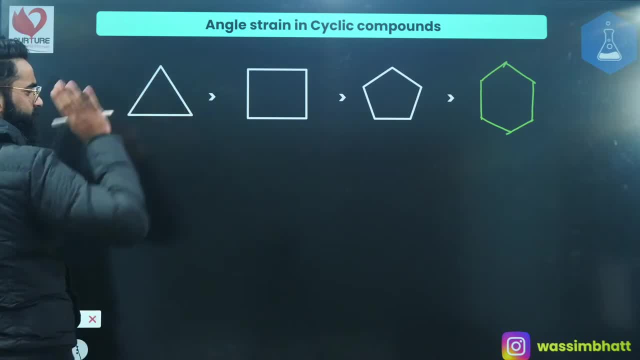 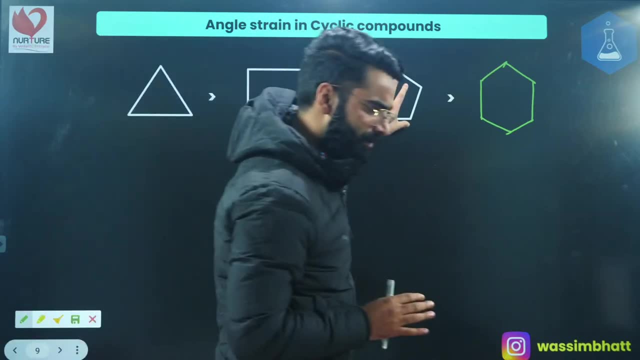 See, guys, this is a simple molecule, which is what we call a cyclopropane. It's cyclopropane right. One, two, three, four. this is cyclobutane. yeah, This is cyclopentane right. 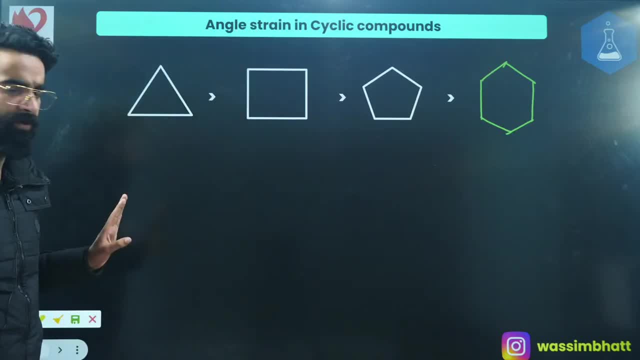 What about this one? This is cyclohexane, Something which every one of you would be knowing, correct? Now have a look exactly. Have a look exactly, guys, If I talk about this carbon atom over here. this is a carbon atom, basically, this is a. 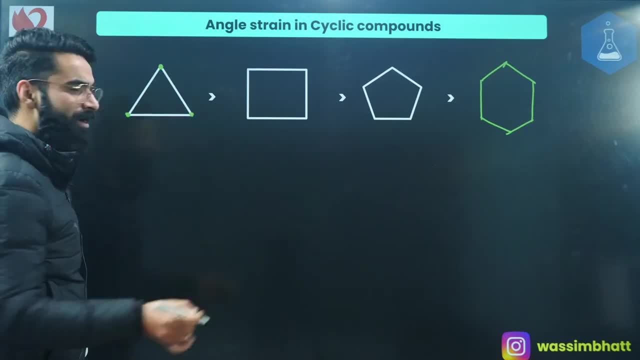 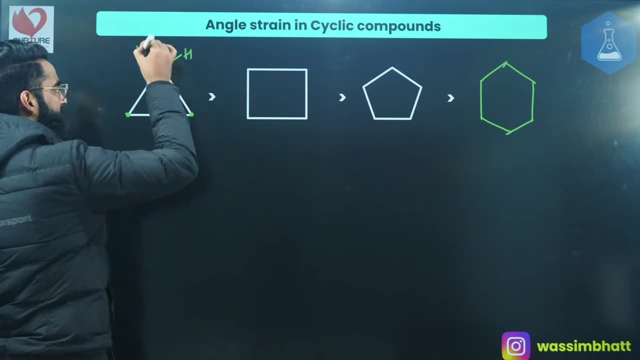 carbon atom. this is a carbon atom right. Carbon forms four bonds. If I talk about this carbon atom in particular, it's forming one. two: there will be one hydrogen on this side. there'll be one hydrogen on this side, correct? 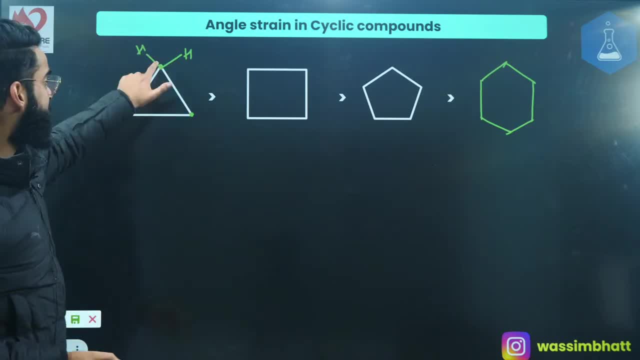 Yes, then only its valence will be satisfied, correct? This carbon is forming four sigma bonds? If it is forming four sigma bonds, what is going to be its hybridization? One, two, three, four. One, two, three, four. 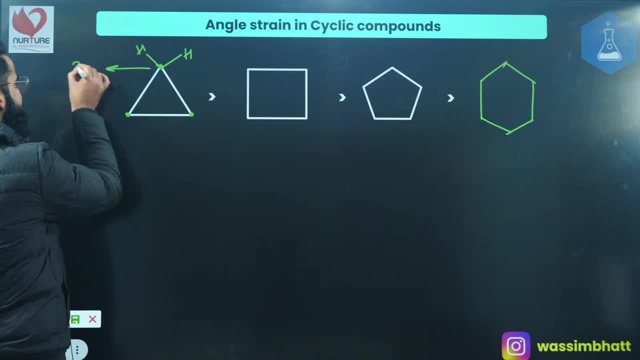 Steric number is four. Its hybridization is sp3.. If its hybridization is sp3, what is going to be the expected bond angle? Isn't it going to be 109 degree 28 minutes? This is expected bond angle over here. 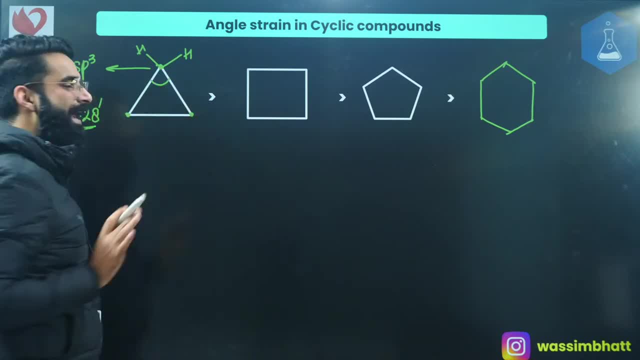 So bond angle over here should have been 109 degree 28 minutes, right, But is the bond angle over here 109 degree 28 minutes? No way, It is just 60.. It is just 60. Do remember Whenever. 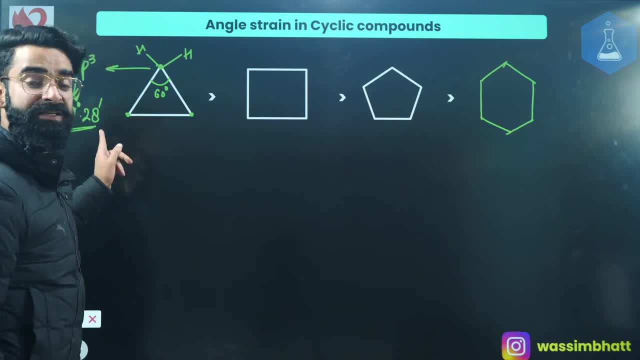 When a molecule expected bond angle, expected bond angle is greater than that of actual bond angle, or whenever in a molecule the actual bond angle is less than the actual bond angle is less than the expected bond angle, We say that molecule is under angular strain. 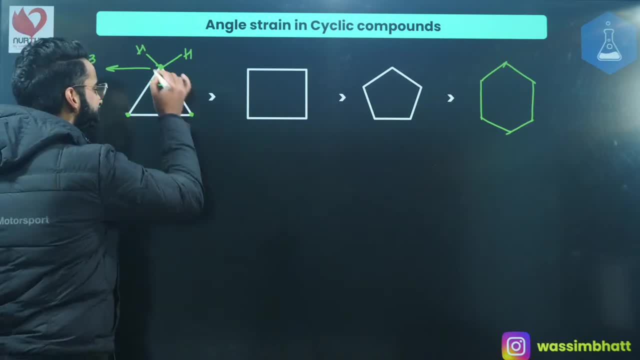 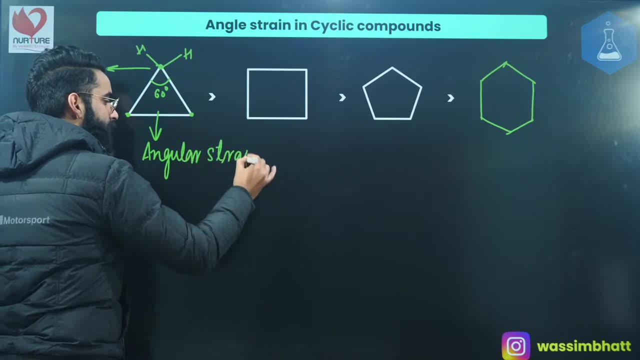 We say the molecule is under angular strain. So this ring, actually it is under angular strain. right, It is under angular strain. These are some basic things which I'm telling you. I will say: this ring is under angular strain and that ring which will be under angular 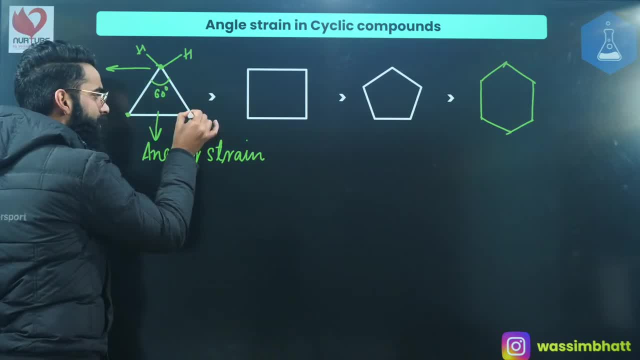 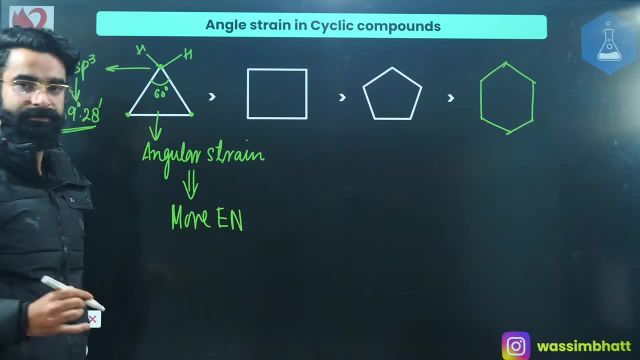 strain, the atoms forming the ring. they are considered to be more electronegative. they are considered to be more electronegative. yes, this molecule over here, which I am considering this, is under angular strain. yes, so the atoms forming the ring, the electronegativity will. 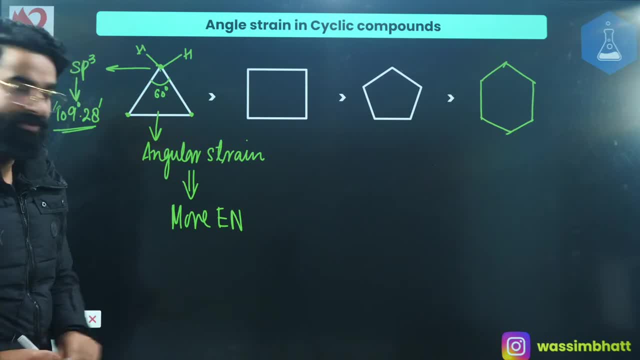 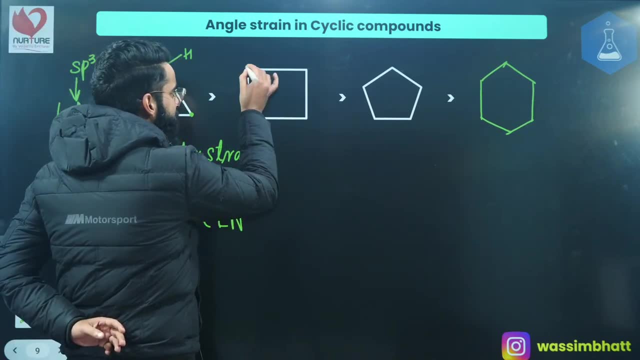 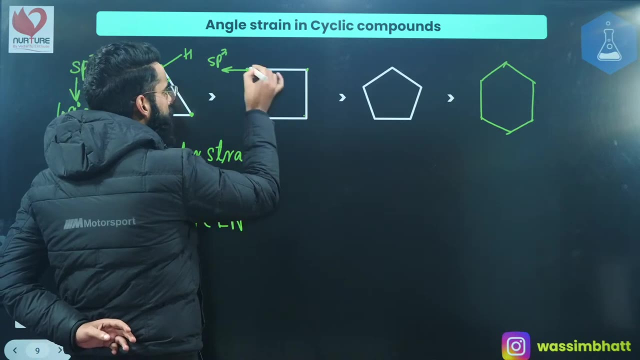 be more, that electronegativity will be more. this molecule is under strain, this molecule is under tension. right, if I talk about this one, this carbon, this carbon, every carbon is sp3 hybridized. every carbon is sp3 hybridized. right, this carbon is forming one, two, there'll. 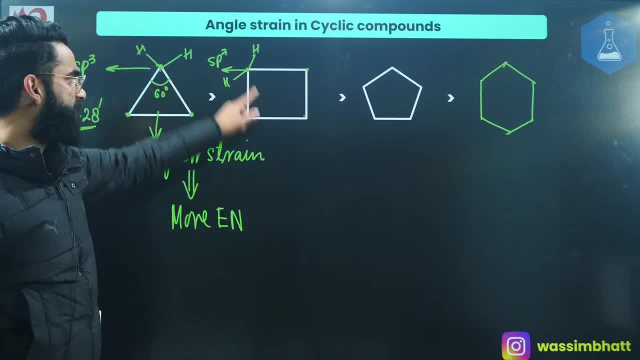 be two hydrogens as well. three and four correct this. sp3 hybridized, what should be the x. what is the expected bond angle? expected is 109 degree 28 minutes. what is the actual one? actual one is actual. one is 100 degree 28 minutes. what is the actual one? actual one is actual. 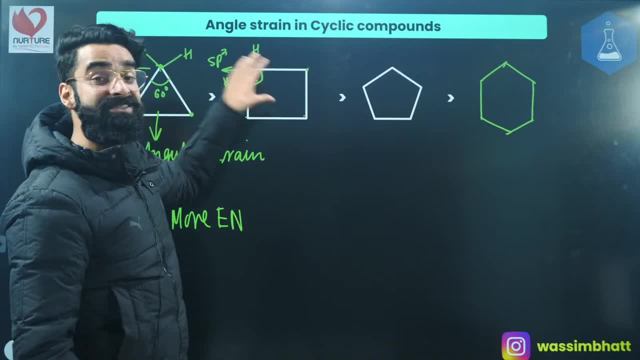 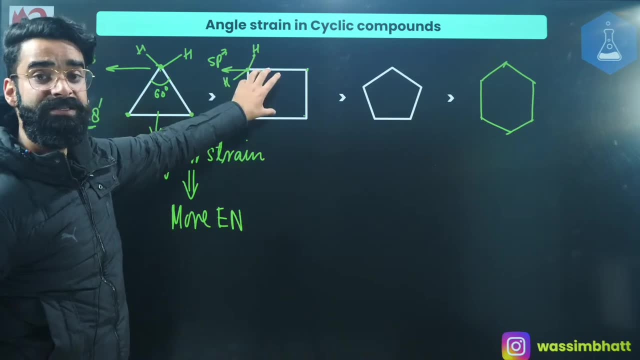 bond angle is less than that of expected, so this molecule is under strain as well. this molecule is under strain as well. yes, this molecule is under strain as well. if this molecule is under angular strain, the atoms forming the ring, their electronegativity, will be more. 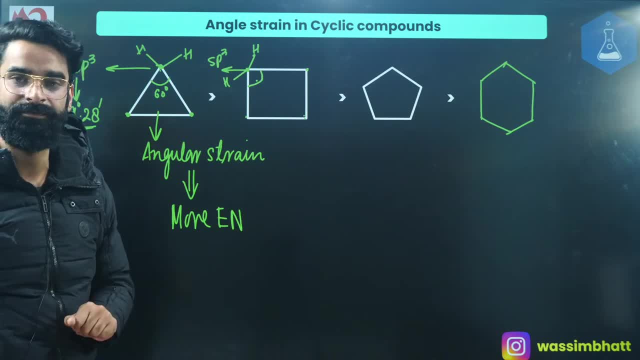 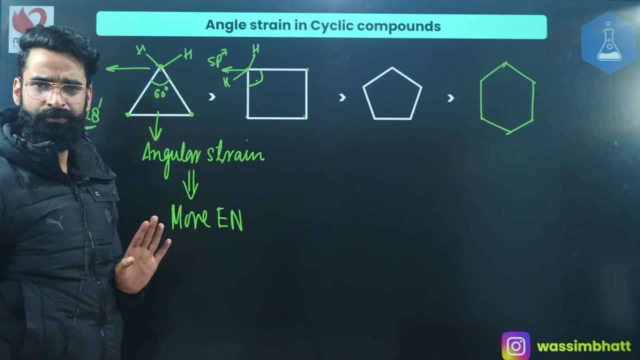 than expected. their electronegativity will be more than expected, right if I? if I want to compare the strain in these two molecules, where is the strain more? where is the stain more? see actual bond angles. is there is a strain in these two molecules? where is the? 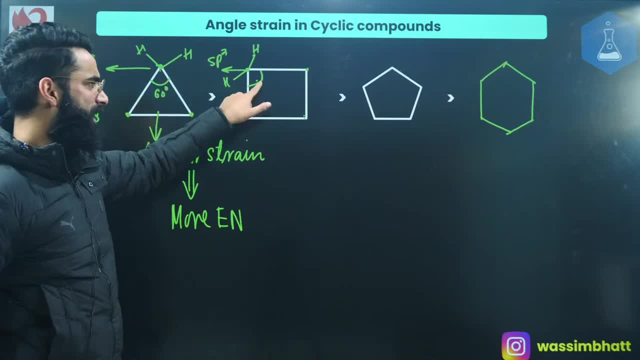 strain more. where is the stain more? see actual bond angles. is there is a strain more where across more gusto sp2, where it is actually in the range of what this molecule is under more tension, is less than that of expected. Over here again, actual bonding is less than that of expected. right, it's 90, correct it's. 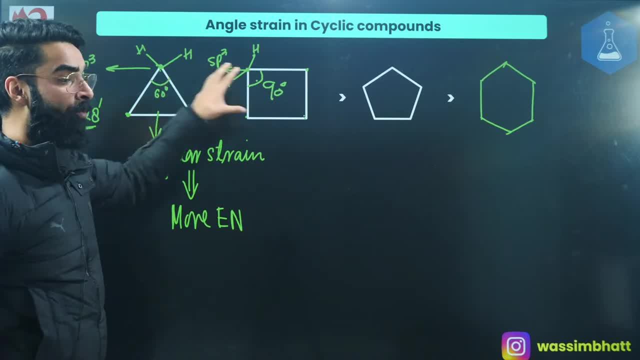 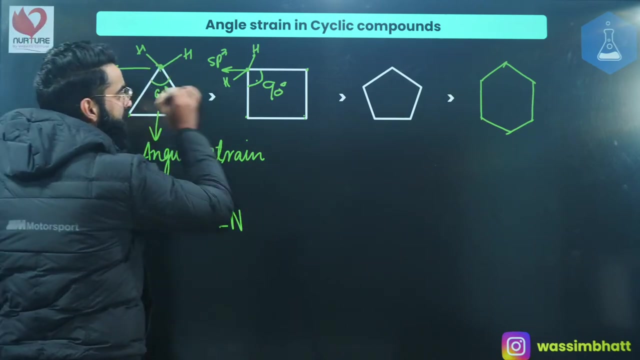 90. okay. so which molecule is under more union? I'll say this molecule is under more tension. this molecule is under more angular strain. if this molecule is under more angular strain, the atoms forming the ring that it through negativities will be more than that of the 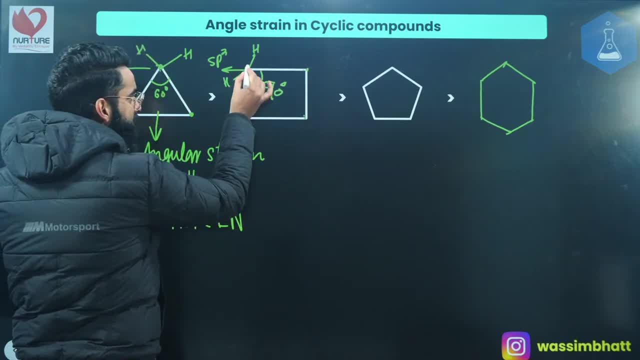 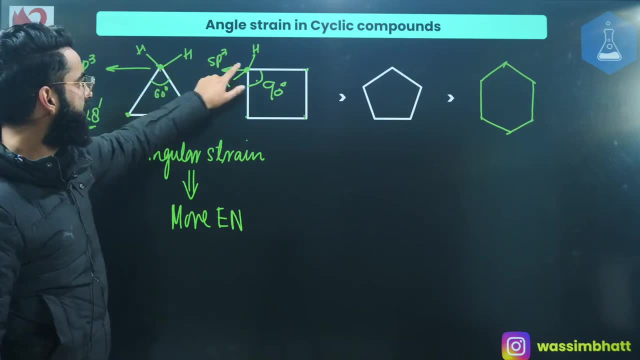 atoms forming this ring right. So if I want to compare atom and this carbon atom, Which carbon atom is going to be more electronegative? I must say this carbon atom is more electronegative than that of this carbon atom. This carbon atom is more. 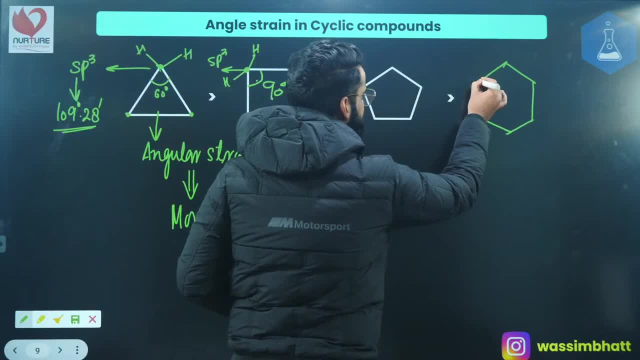 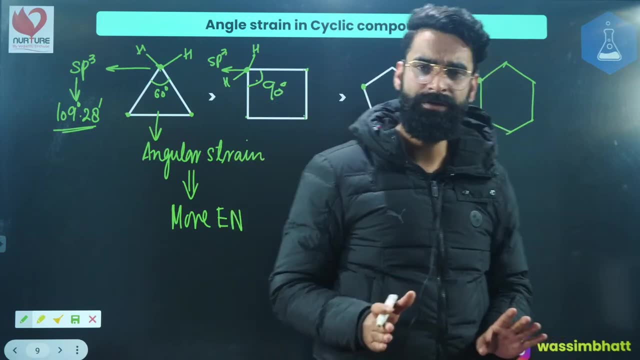 electronegative than that of this carbon atom. This carbon atom is more electronegative than that of this carbon atom. Do remember this thing as well. right, More the angle strain, more the strain in the molecule, right, More is going to be the electronegativity of the atoms. 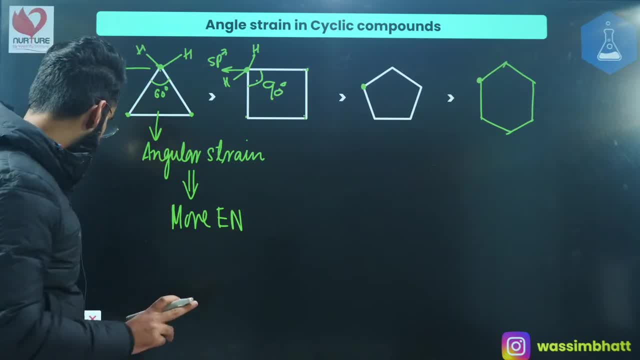 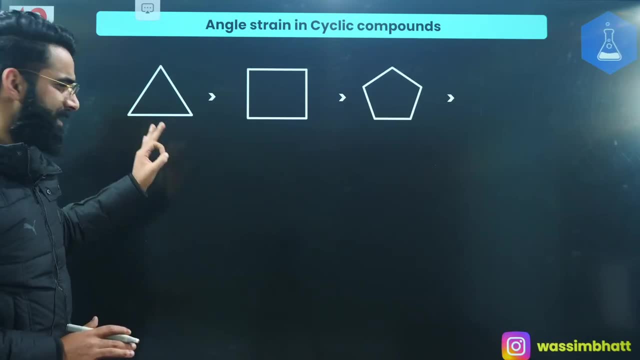 forming the ring. Yes, As simple as that. okay, I'm going to use the same concept in the questions in some time, right? So you need to remember everything. You need to take a note of every single thing which I'll be mentioning over here, correct? Look at this molecule in particular. Look. 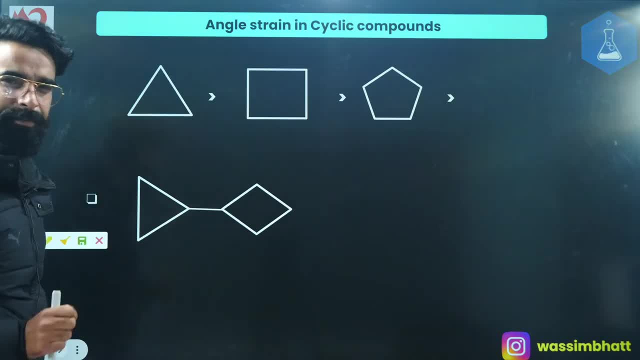 at this molecule in particular. right, Have a look exactly what is happening. Have a look exactly what is happening If I talk about this carbon and this carbon. these are two carbon atoms basically over here. right, These are two carbon atoms. Yes, This is your, basically cyclopropane and this is. 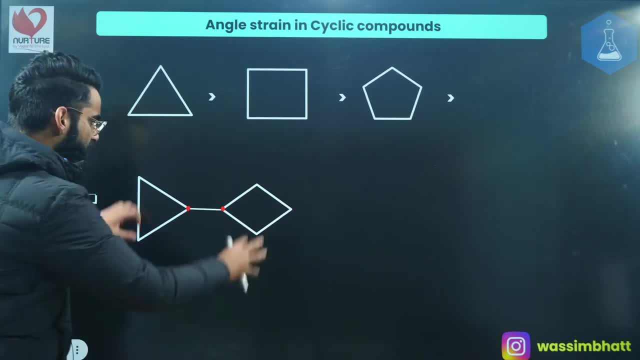 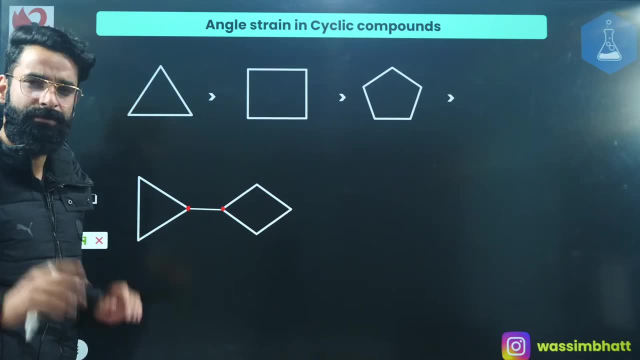 your cyclobutane, and these two are connected. These two are connected. If I ask you which ring among the two, these are two rings basically connected. Which ring among the two is under more angle strain? What do you think? Which ring among? 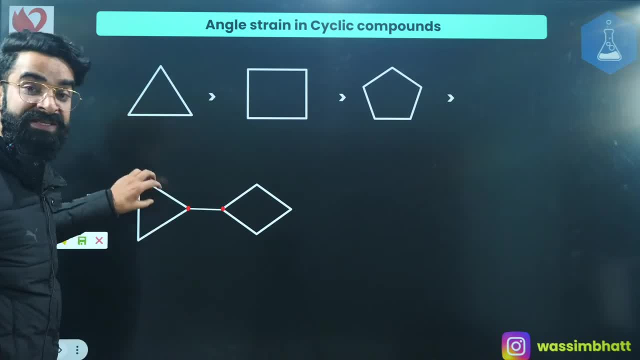 the two is under more angular strain. This ring is more is under more angular strain. If this ring is under more angular strain, so I must say electronegativity of this carbon atom will be more than that of this carbon atom, right, If the electronegativity of this carbon atom is more. 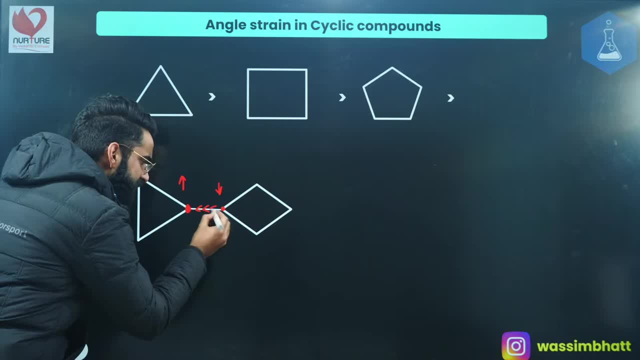 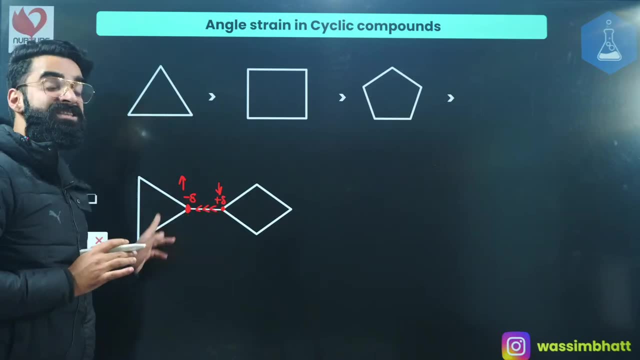 then this carbon atom will have more tendency to attract the bonded pair of electron towards itself, due to which this carbon gets delta negative. this carbon gets delta positive, right. So, due to the different angle strains, due to the different electronegativities, what is happening? 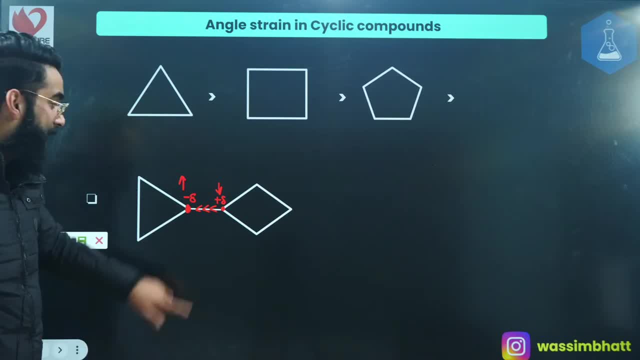 over here. What is happening over here? Can I say again, the partial polarity is getting developed. Partial polarity is again getting developed over here due to the difference in the electronegativities. and why is the difference in the electronegativities? Because of the difference in their angular strain. 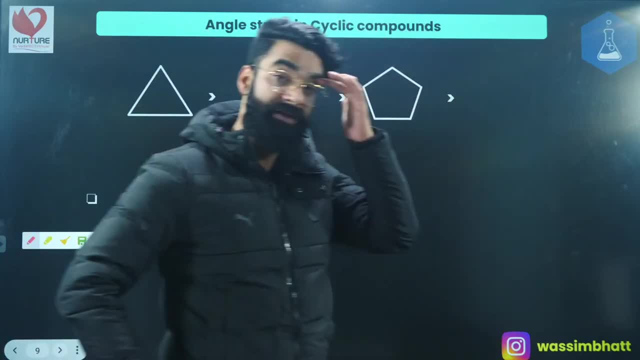 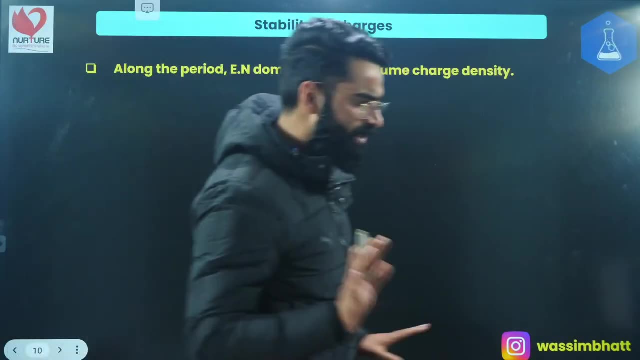 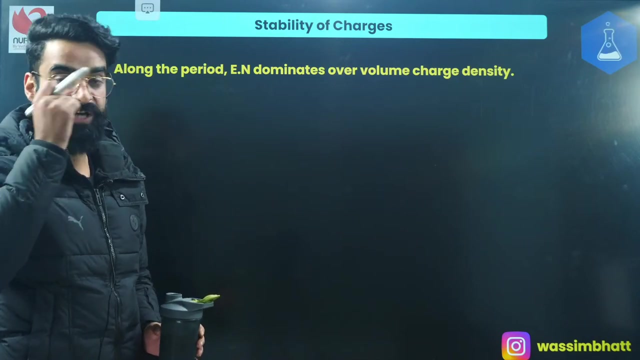 So right, Yes, as simple as that. okay, Right, people, I'm sure this is also clear to you. Okay, now comes the actual stuff. Whatever I told you till now, let's try to apply all this in the equations. But before the equations, let's have a look on certain important rules which I 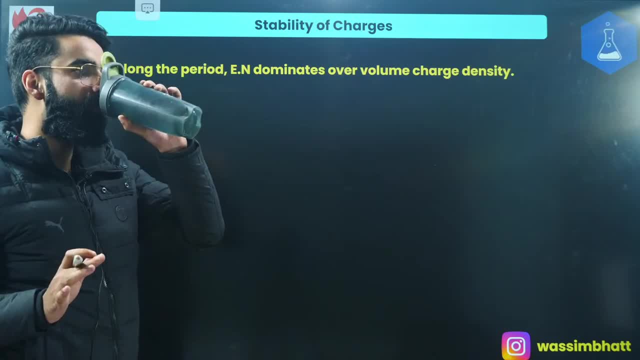 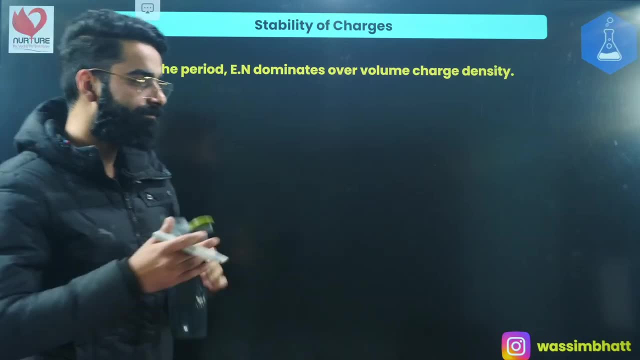 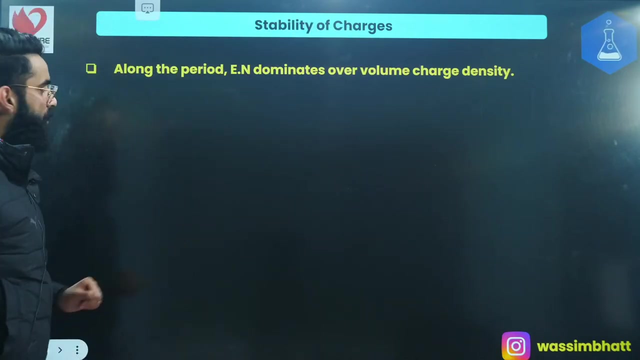 want all of you to take a note of correct. Till then, you guys can let me know in the charts if it is clear. till here, right, Okay, Do remember whenever you need to compare, whenever you need to compare the stability. 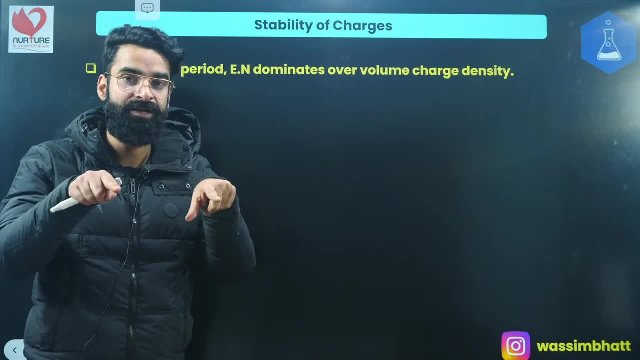 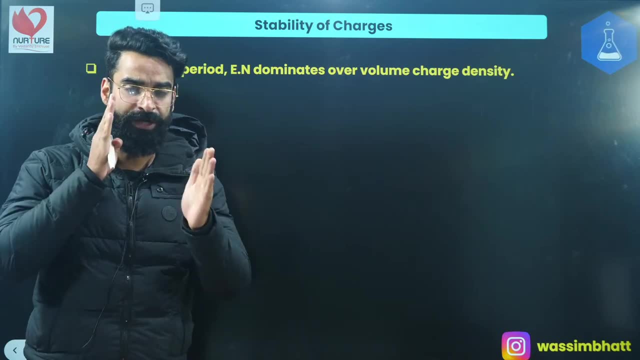 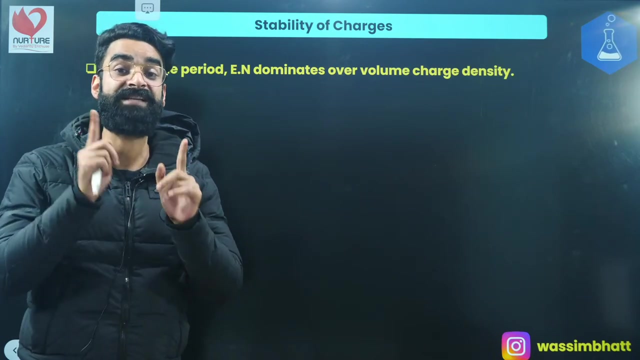 of the charges on two elements, on two elements which belong to same period, which belong to same period. whenever you need to compare the stability of the charges on two elements which belong to same period, you will be comparing the stability of the charges on the basis. 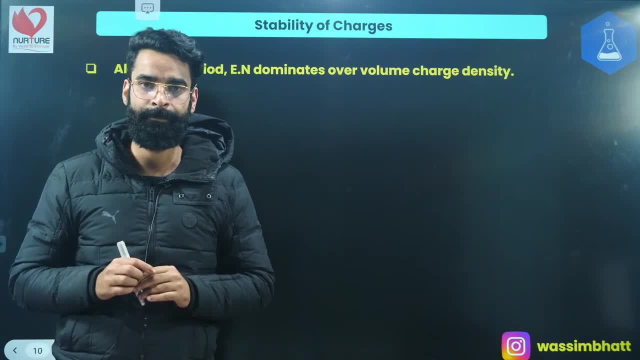 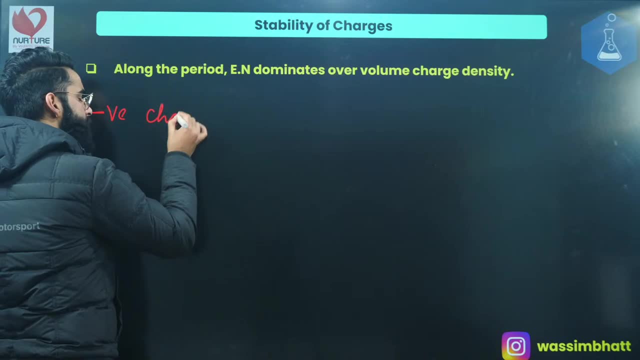 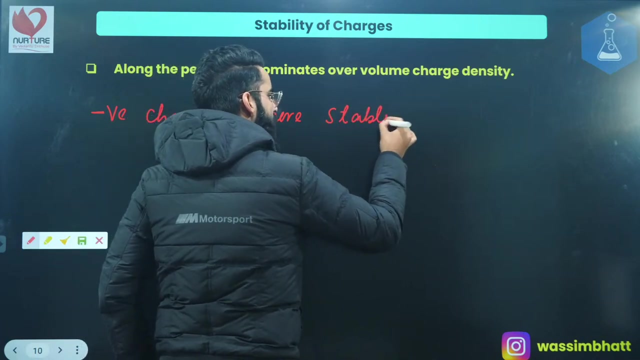 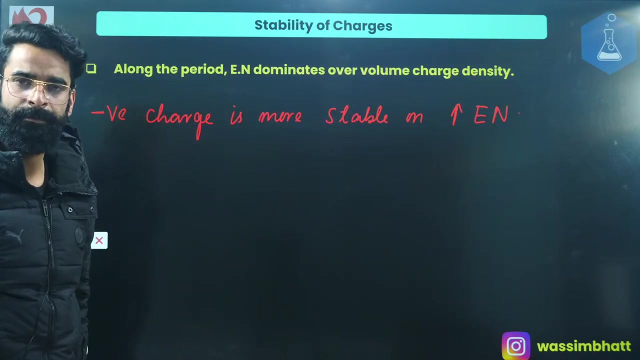 of electronegativity. on the basis of electronegativity, Do remember negative charge. do remember negative charge is more stable, is more stable on more electronegative element. Negative charge is more stable on more electronegative element. Do remember positive charge is more. 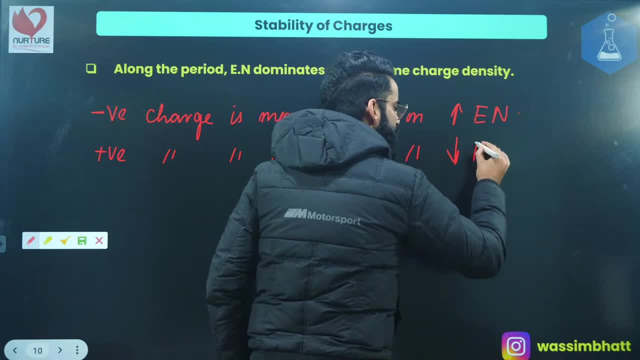 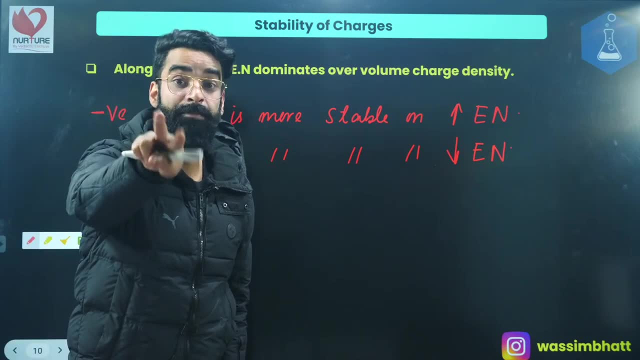 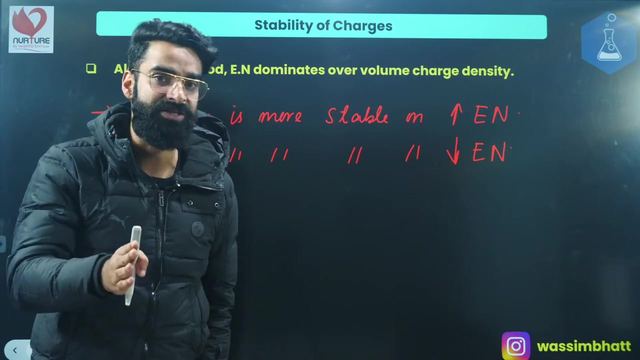 stable. Positive charge is more stable on less electronegative element. Just do remember these two things First of all. whenever I need to compare the stability of the charges present on two elements which belong to the same period, I'll be comparing the stabilities of the charges on the elements. 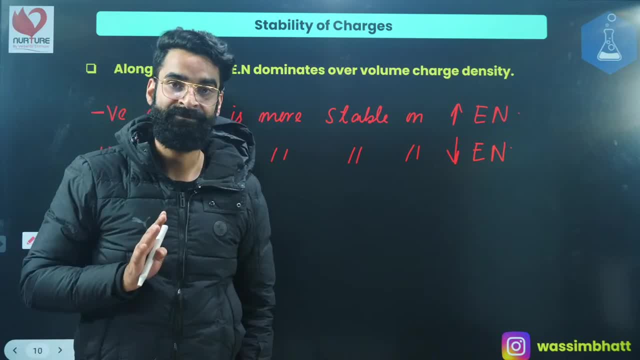 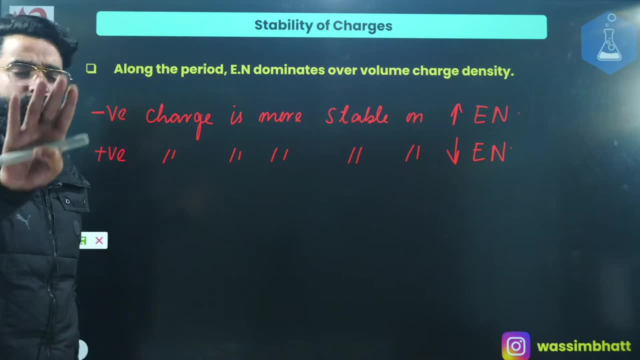 which belong to the same period. by means of electronegativity. Negative charge is more stable on more electronegative element. Positive charge is more stable on less electronegative element. These are the two things which you need to take note of. 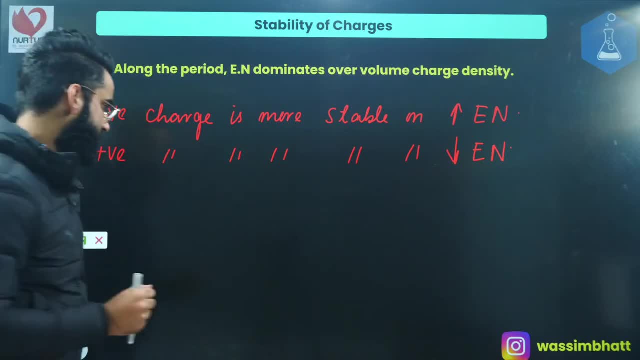 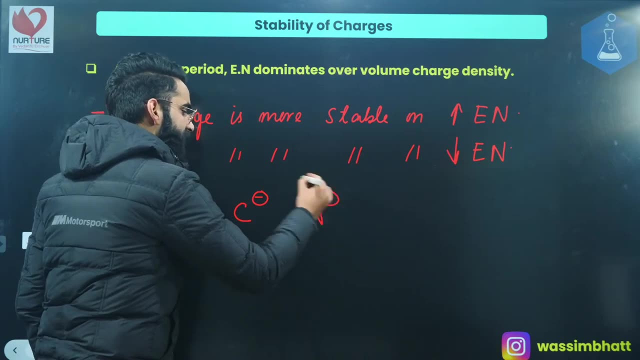 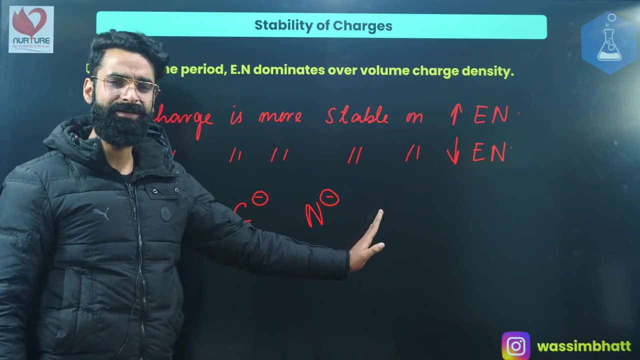 Right, For example. for example, Let's say I've got carbon carrying the negative charge. Let's say I've got nitrogen carrying the negative charge. carbon and nitrogen do they belong to same period? absolutely they belong to same period, right? I need to compare the. 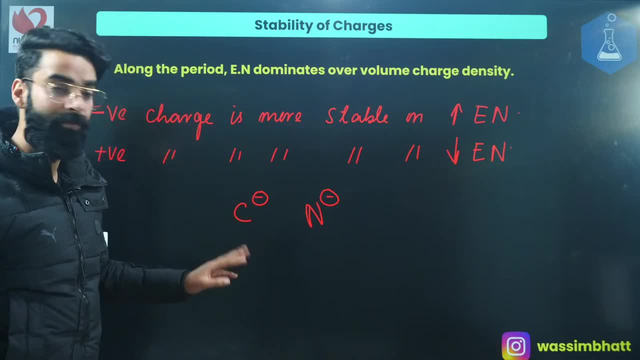 stability of the charges. Where is the negative charge more stable? Whenever I'll be comparing the stability of the charges on two elements which belongs to the same period, I'll be comparing it on the basis of electronegativity. Right Negative charge is more stable on two. 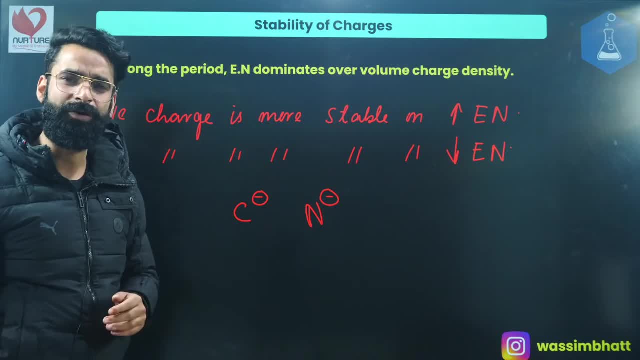 elements which belong to the same period. right: Negative charge is more stable on more electronegative element. When I反이� attach esto to this, this analogous drugs and this analogous charge is more stable on more electronegative element. negative charge is more stable on more. 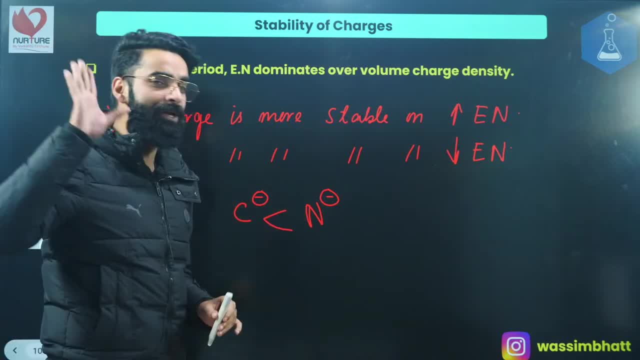 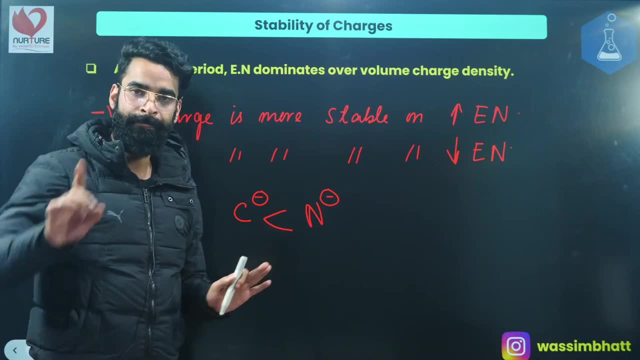 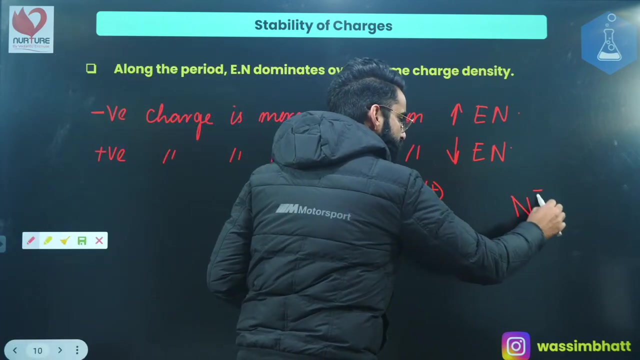 electronegative element. right, so negative charge of nitrogen is definitely going to be more stable on nitrogen as compared to that of carbon. yeah, as simple as that. okay, similarly, have a look. let's say: i've got carbon carrying the positive charge, i've got nitrogen carrying the positive charge. 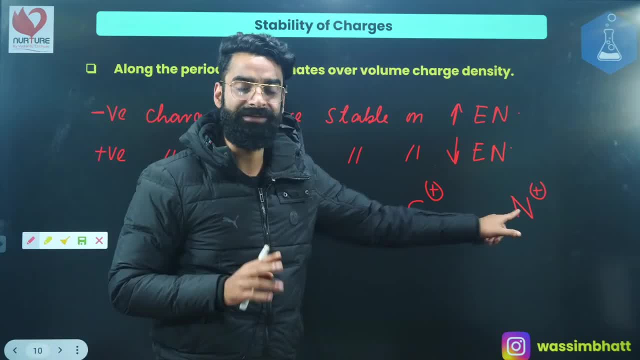 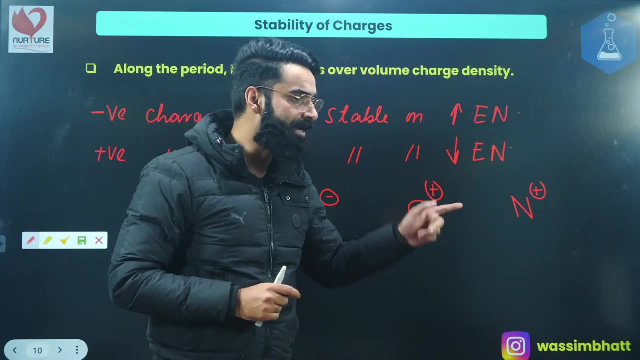 again, if you see over here, carbon and nitrogen, these are the two elements which belong to the same period. right, these are the two elements which belong to the same period. i need to compare the stability of the charges on these elements. i need to compare the stability of the charges. 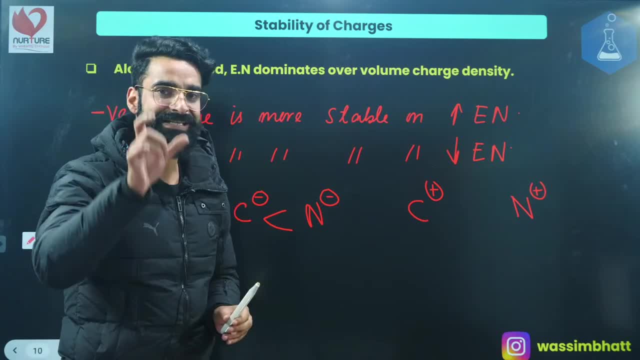 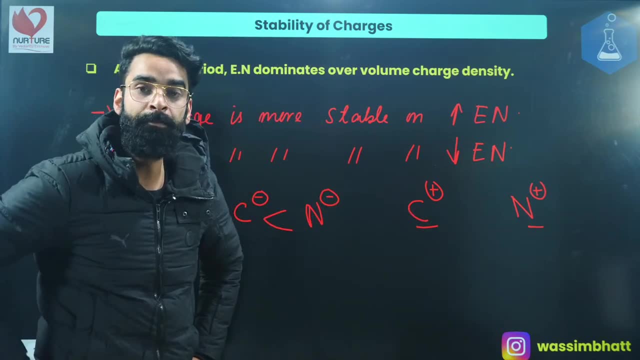 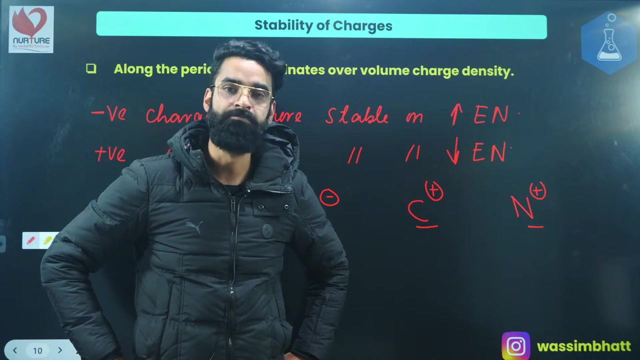 on these elements right. whenever you need to compare the stability of the charges on two elements which belong to same period, at that point of time we'll be comparing the stabilities on the basis of electronegativity. as i told you five minutes back, positive charge is more stable on. 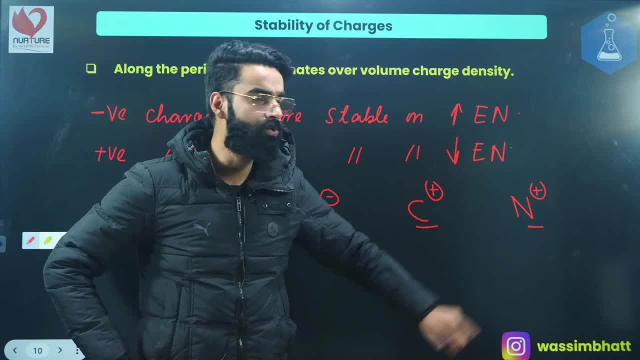 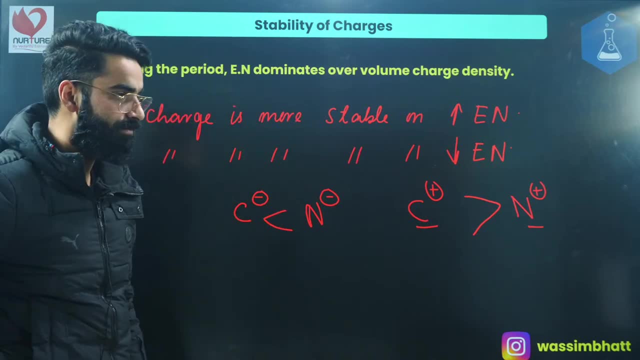 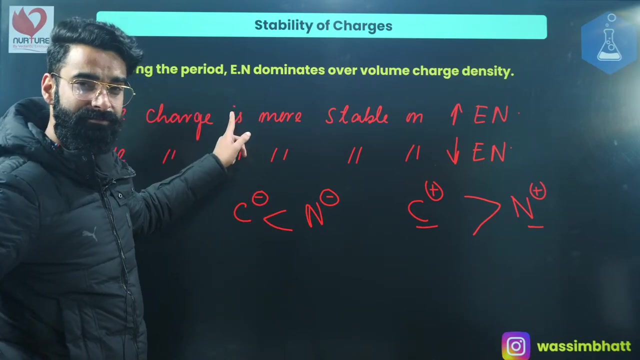 less electronegative element? which element among the two is less electronegative? isn't it carbon? absolutely so positive charges will be more stable on carbon as compared to that of nitrogen. yeah, simple, right. so this is a very, very valid and important point. i'll be using this point everywhere in your organic chemistry. 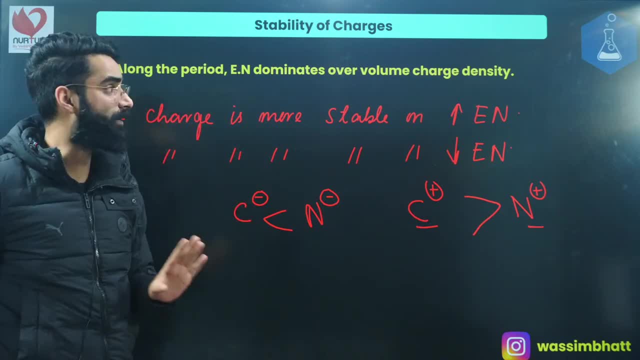 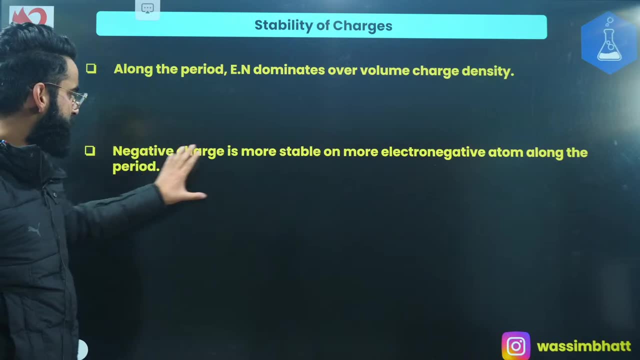 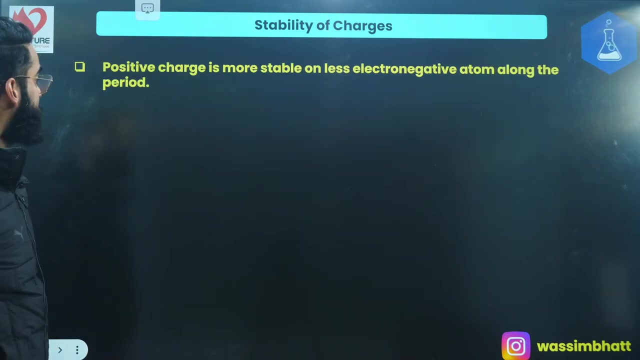 do you remember the things which i told you till now, correct? yes, right now comes one more point. there's something which i told you: positive charge is more stable on more electronegative element whenever you are comparing the stability of the charges on elements which belong to the same period. right, there's something which i told. 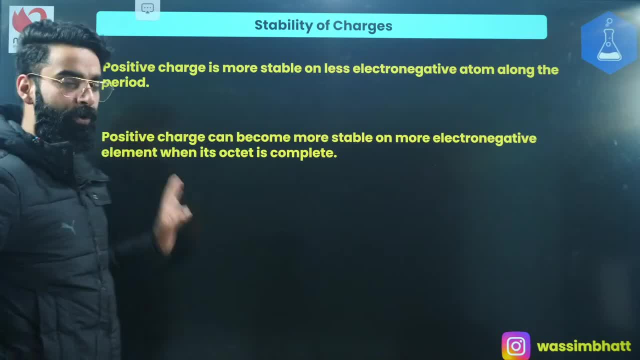 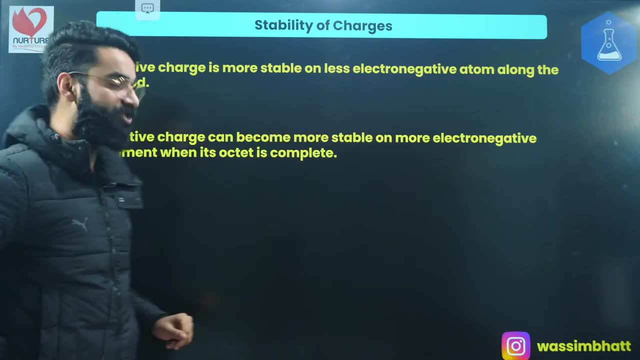 you too correct? this is one more point. positive charge can become more stable. it can become more stable on more electronegative element, but there is a condition: when its octet will be complete. when its octet will be complete, what is meant by this term? you'll get this idea in some time. 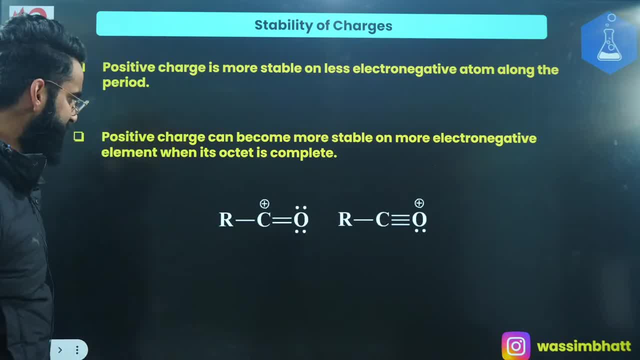 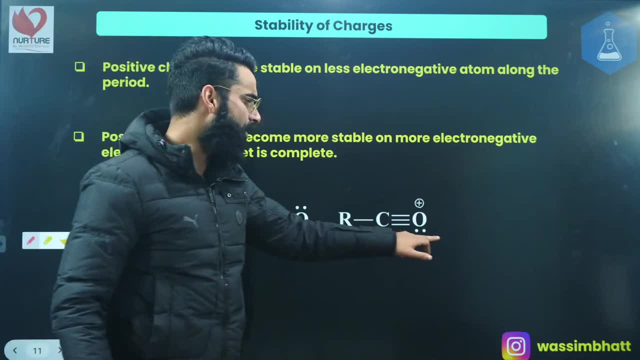 or let's have a look over here, only, let's have a look over here, only say: guys say exactly, in these two molecules, if you talk about this carbon, this carbon is having the positive charge right over here, this oxygen is having the positive charge. carbon and oxygen do they belong to same? 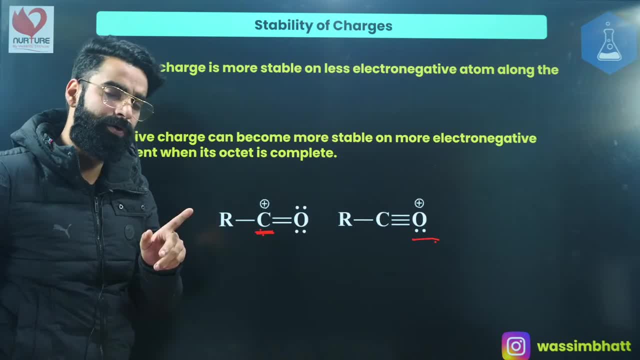 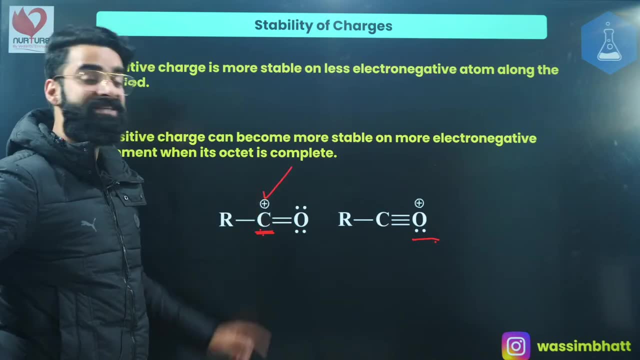 period? absolutely, they belong to same period. few minutes back, i told you positive charge is more stable on less electronegative element, so positive charge should be more stable on this carbon. right, positive charge should be more stable on this carbon. but let me tell you positive. 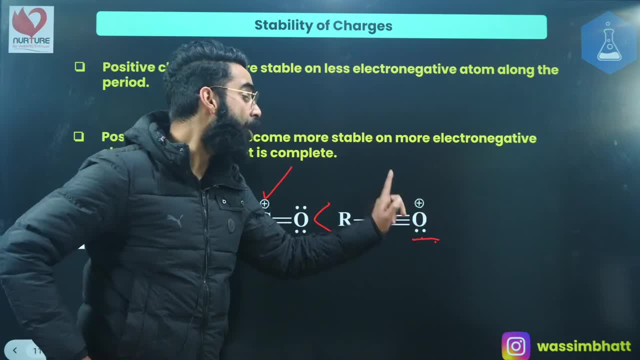 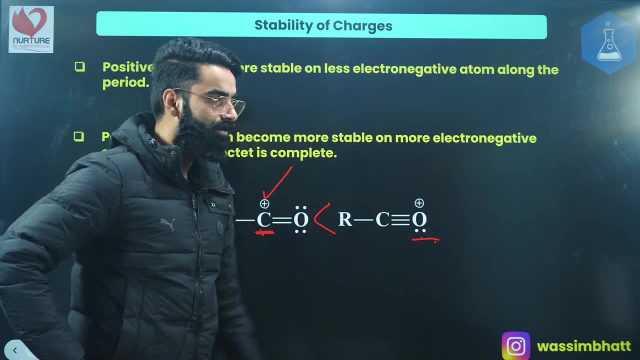 charge in this case is more stable on this oxygen because the octet of this oxygen is complete: two, four, six and lone pair, eight. right r refers to alkyl. group. alkyl it can be ch3, it can be c2h5, whatever, i've got nothing to do with that right now. 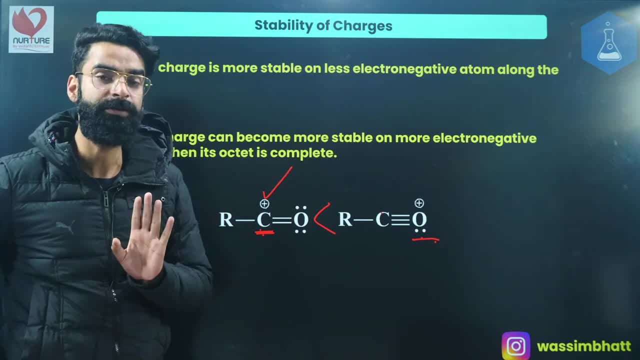 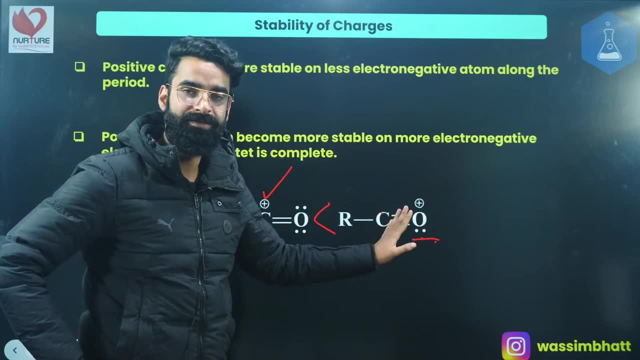 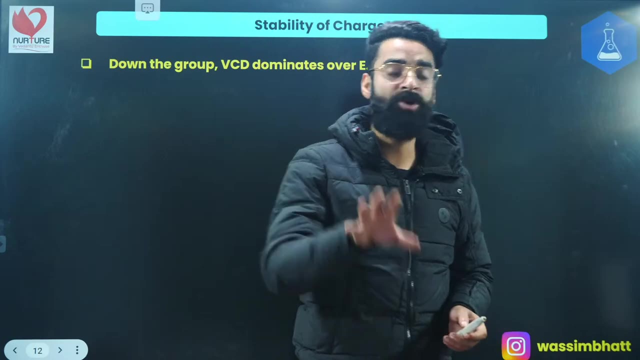 yes, do remember, positive charge can become more stable on more electronic element when the octet of the more electronic element is complete right, as in this case. yes, i'm sure this also clear to you, perfect. now comes a point. this was all about the comparison of the stabilities of the charges on. 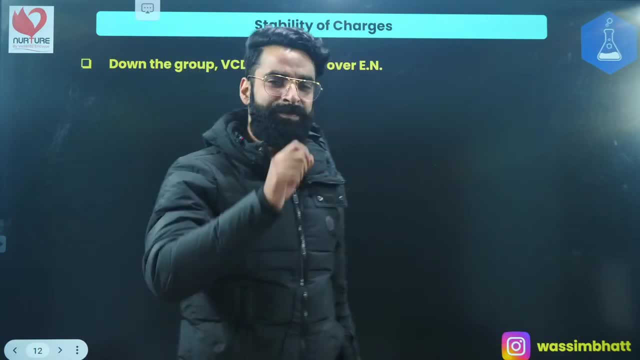 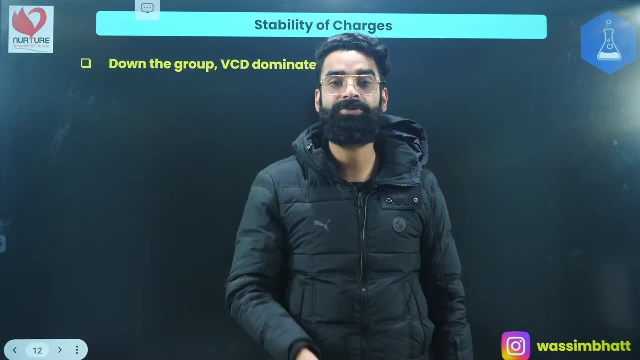 the elements which belong to the same period, right. but, people, if you'll be having two elements which do not belong to the same period, which belong to the same group, which belongs to the same group, right, i'll be having two elements. for example, they are belonging to the same group. yes, both. 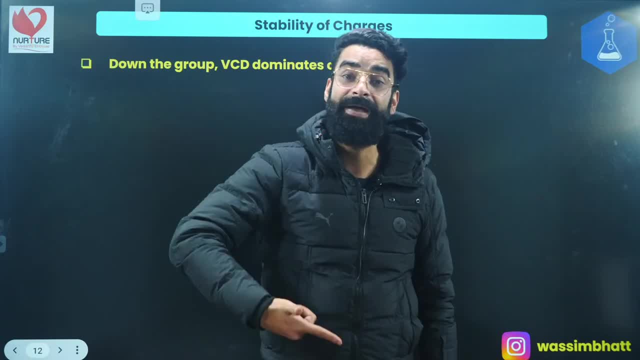 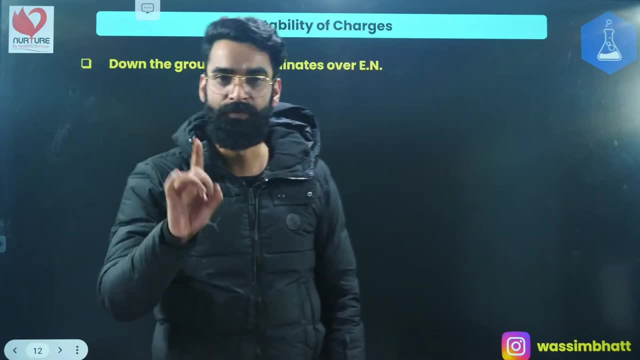 the elements have got some charge on them and you are supposed to compare the stabilities of the charges on those elements which belong to the same group. at that point of time you won't be comparing the stabilities of the charges on the base of electronegativity. you will be comparing. 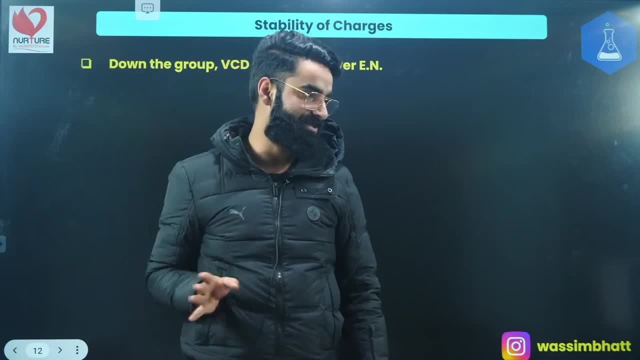 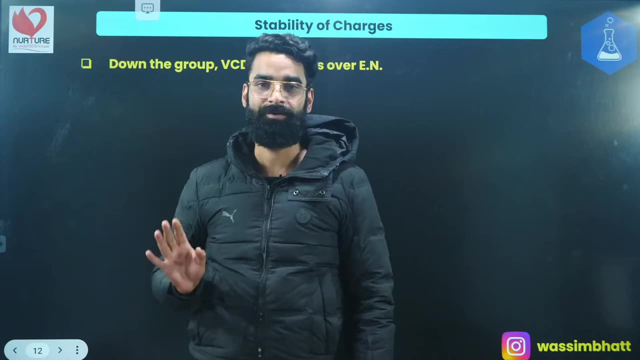 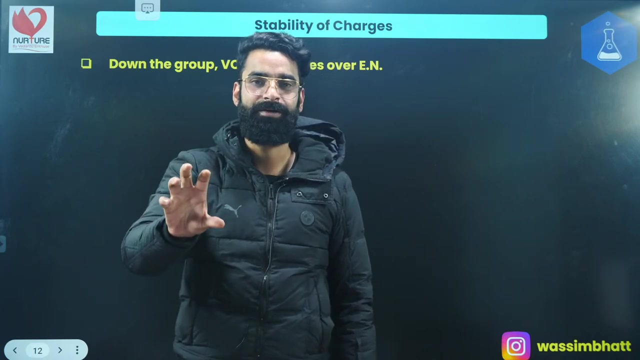 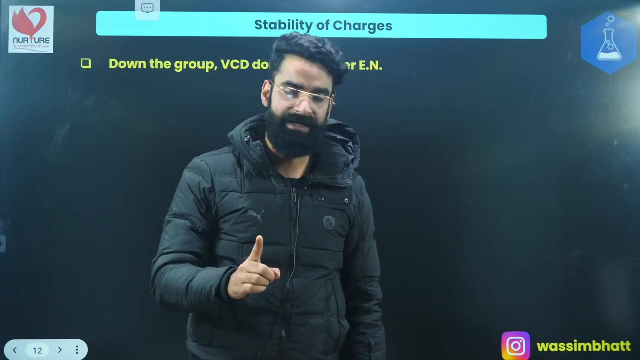 the stability of the charges on the basis of volume charge density. along the period, electronegativity dominates down the group, volume charge density dominates. as i told you earlier, volume charge density is inversely proportional. stability- more volume charge density- less stability, less volume charge density- more stability. right, that's something which i told you earlier, correct? 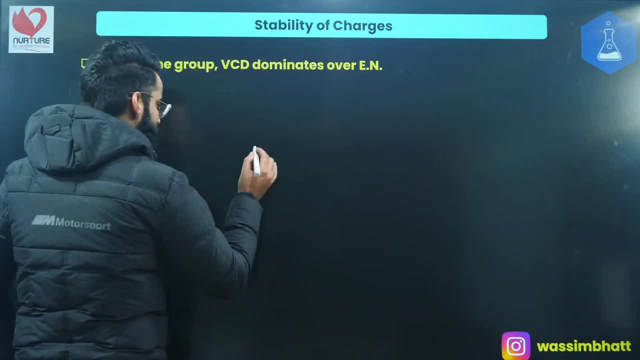 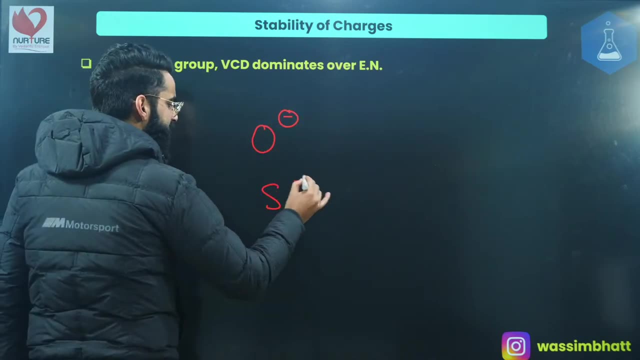 yes, for example, have a look, let's say, let's say i've got, for example, oxygen carrying the negative charge. right, let's say i've got sulfur carrying the negative charge. these are the two elements carrying the negative charge, right? i need to see where is the negative charge more stable? 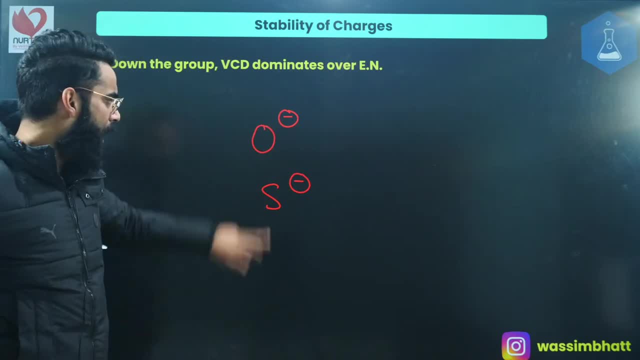 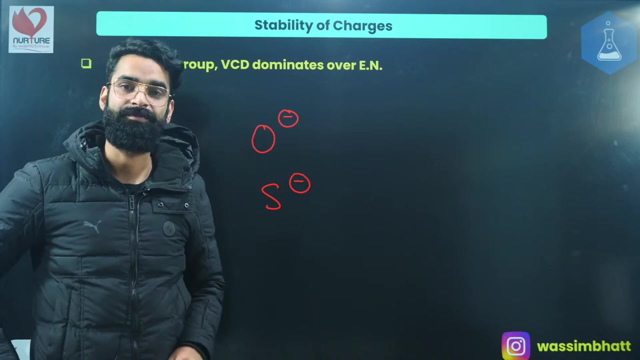 i need to see exactly where is the negative charge more stable. have a look exactly. oxygen and sulfur, first of all identify. do they belong to same period? absolutely they belong to same period. right and whenever. i'll be having two elements belonging to the same period and i need to compare the stability of the charges. volume, charge density comes into. play. you're right, and we know. volume charge density is directly proportional to charge on the specie, inversely proportional to size of the specie. right, and we have discussed volume charge density is inversely proportional to stability as well. right, have a look. the amount of charge on both the elements is same. amount of charge is same but size is different. 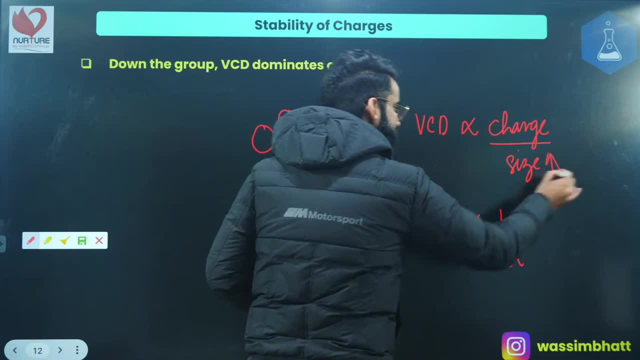 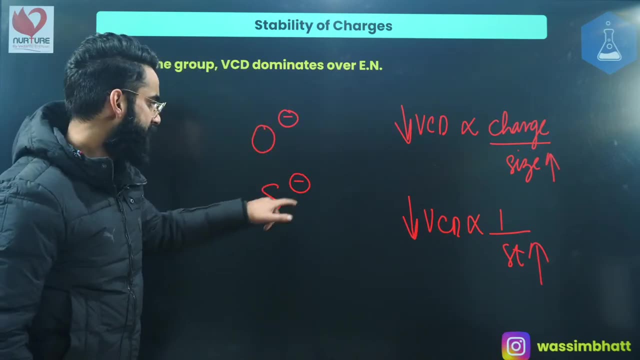 sulfur has got more size. sulfur has got more size. more size means less volume charge density. less volume charge density means more stability. so where is the negative charge more stable among the two? negative charge is more stable on sulfur as compared to that of oxygen. yes, correct two. 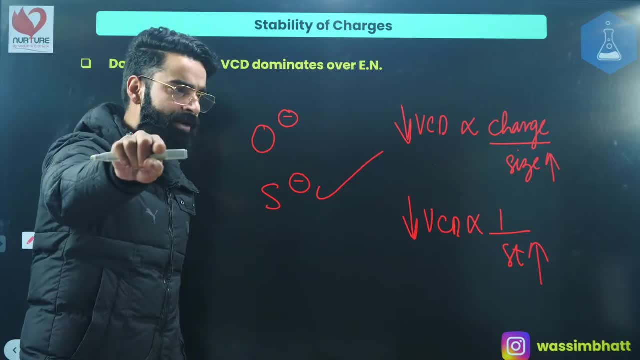 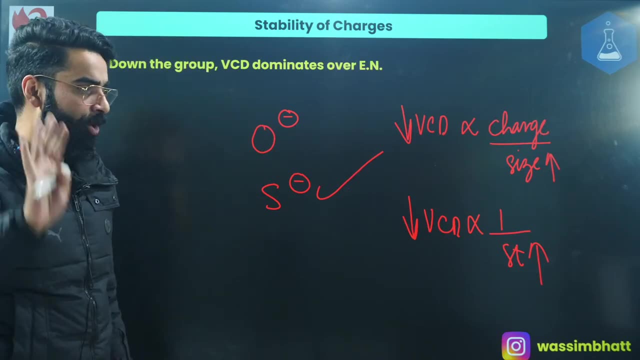 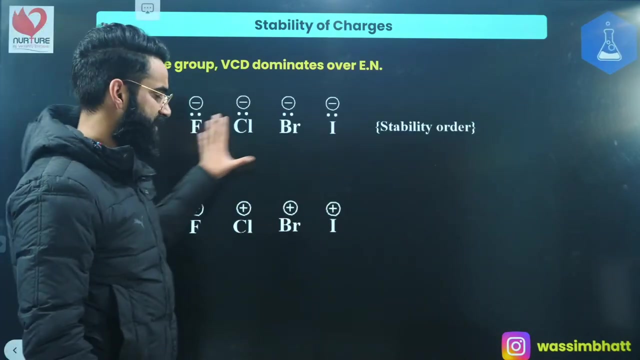 things. in the periodmontan, electric negativity dominates over volume charge density. in the intra田, volume charge density dominates over the electro negativity. right, I'll be using this concept. I'll be doing a lot of questions on this concept, for example. for example. these are first two. 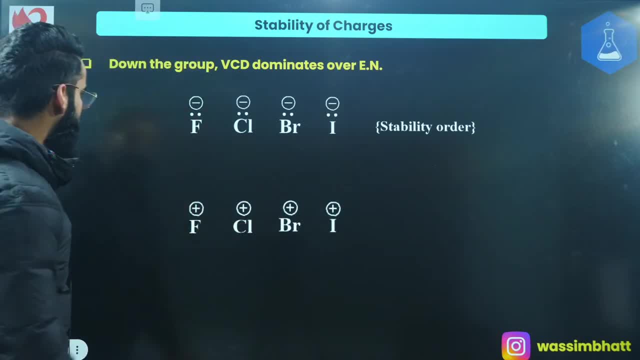 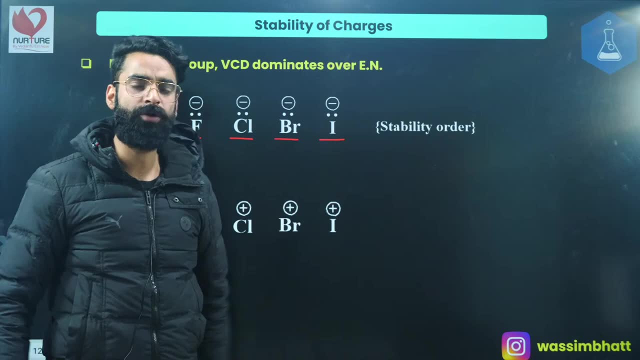 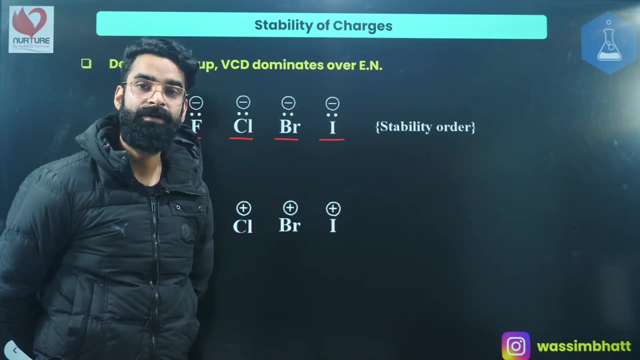 questions. these are first two questions. have a look: fluorine having negative charge, chlorine negative charge, bromine negative charge, iodine negative charge. first of all, identify: do these elements, do they belong to same period? no way they belong to same group, right? so I'll be considering volume charge, density, volume charges in worst episode. size: iodine has maximum size. so minimum volume charge, density. minimum volume charge density means maximum stability, so negate your charge is more stable on iodine than that of bromine, then they're of chlorine, then they're of flooring right. similar. similarly fluorine, chlorine, bromine, iodine- same group volume charge. density plays a role right balling charge. gen Z is inverse. the purpose of the size are: yeah, more size of iodine means volume charge density is least over here. if volume charge density is least, stability of positive charge on iodine will be maximum. so this is the stability of the stability order of the charges on these. 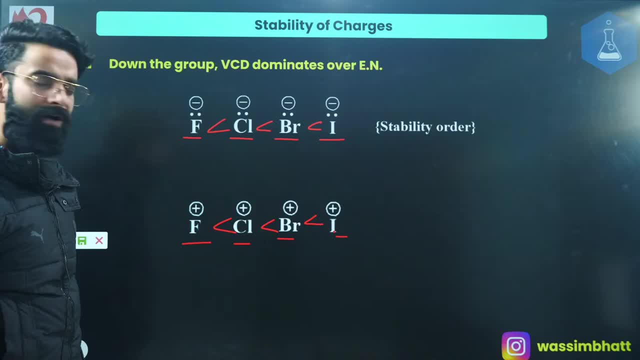 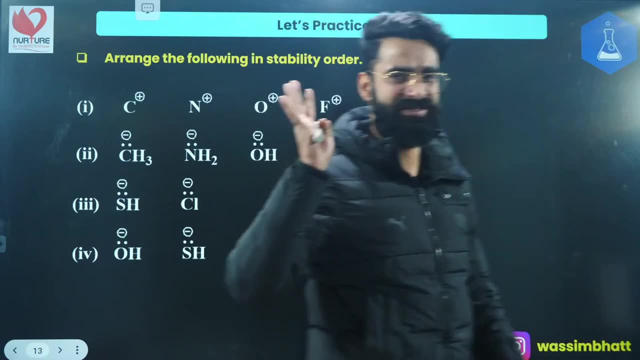 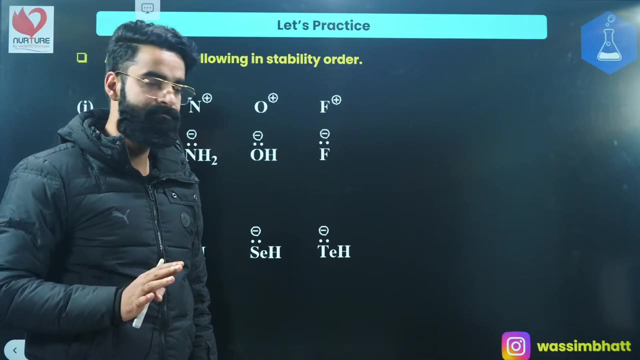 elements. isn't it simple, my dear people? isn't it simple? absolutely just two things you need to remember, that's all. let's try to do some questions and let's try to master this concept. this is a single concept which you'll be using everywhere. trust me on that. yes, have a look. arrange the following in: 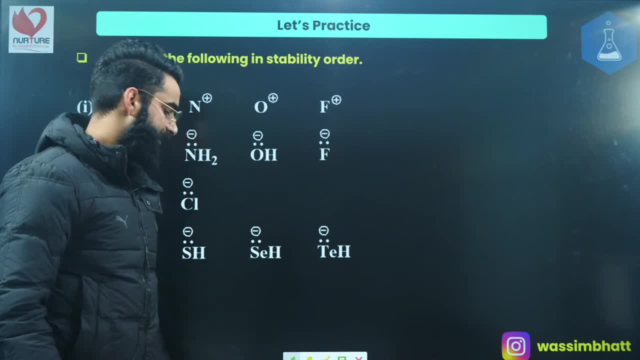 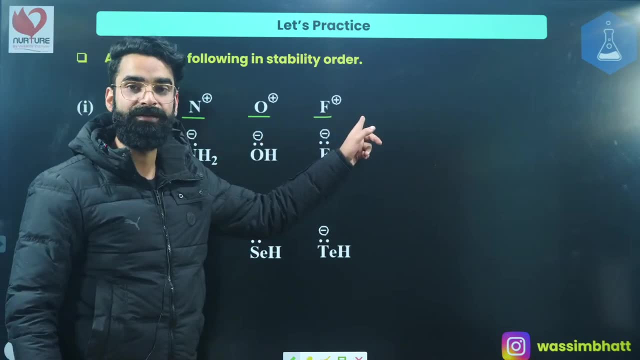 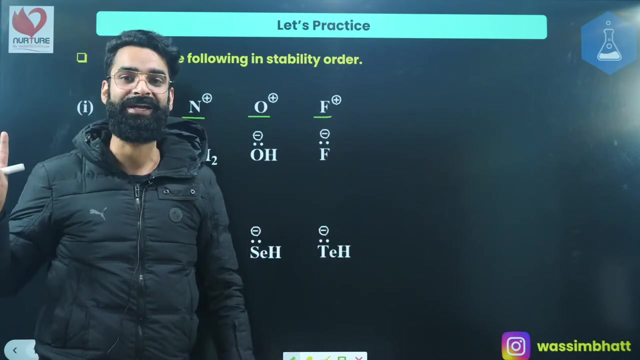 the stability order. you need to arrange the following on the base of the stability order. how about over here carbon having positive nitrogen positive oxygen positive fluorine positive? these elements belong to same period. electronegativity plays a role. positive charge is more stable on less electronegative element. positive charge is more stable on less. 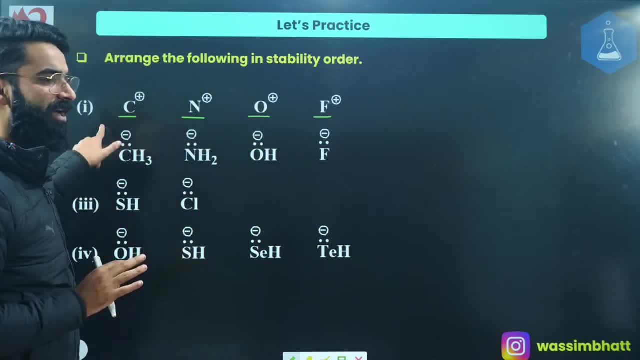 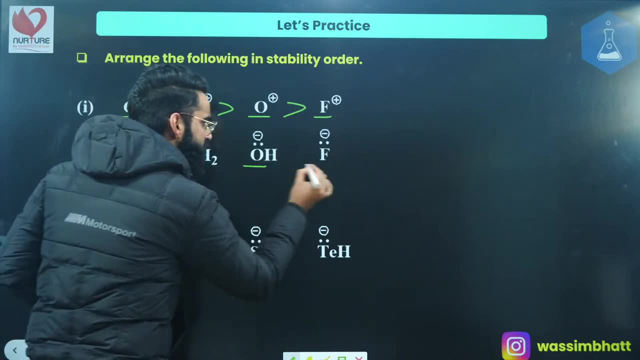 electronegative element, which is is the least electro-negative among the following: carbon. So positive charge will be most stable over here. As simple as that. okay, carbon having negative, nitrogen negative, oxygen negative, fluorine negative, All these elements- carbon, nitrogen, oxygen, fluorine. 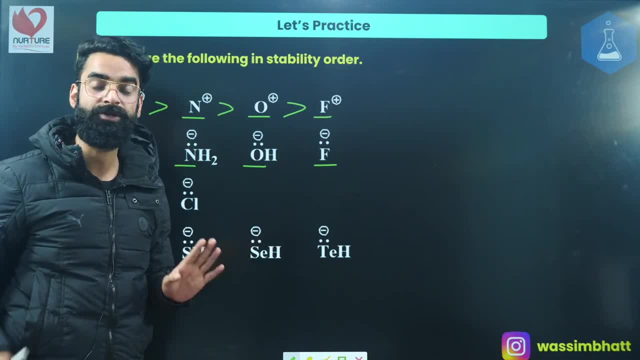 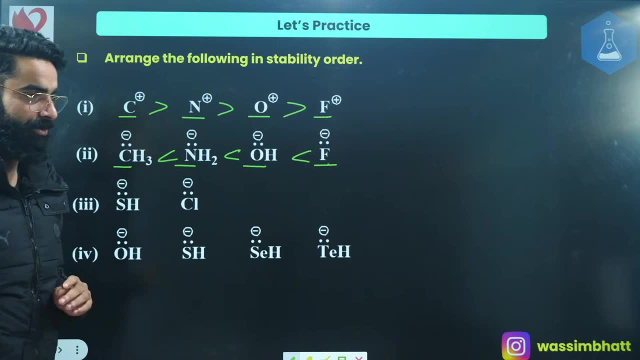 again, they belong the same period. right Again, they belong to same period. Electronegativity- again. Negativity charge is more stable and more electro negative element. Negative charge is more stable and more electro negative element. This is the order, yeah. 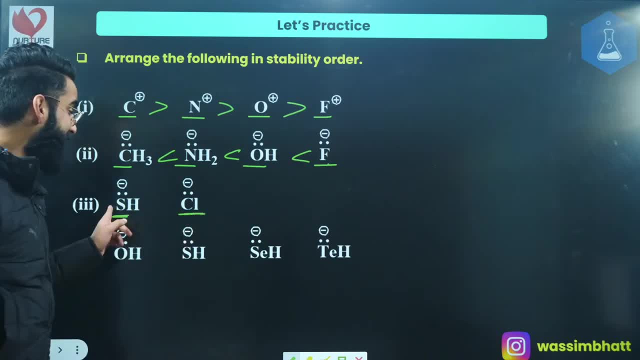 Sulfur carrying negative charge. chlorine carrying negative charge- Again, same period elements. Same period elements. Correct, Yes Again, electronegativity: Which one is more electronegative? Chlorine is absolutely more electronegative than that of sulfur. 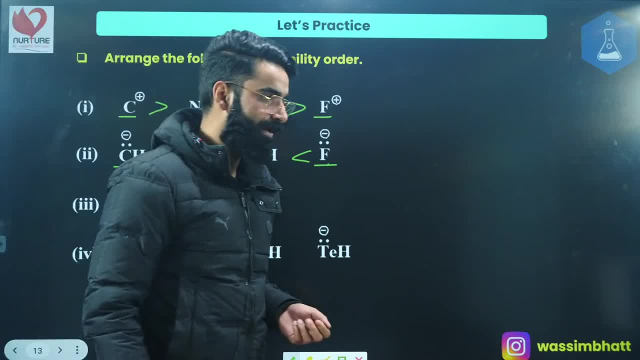 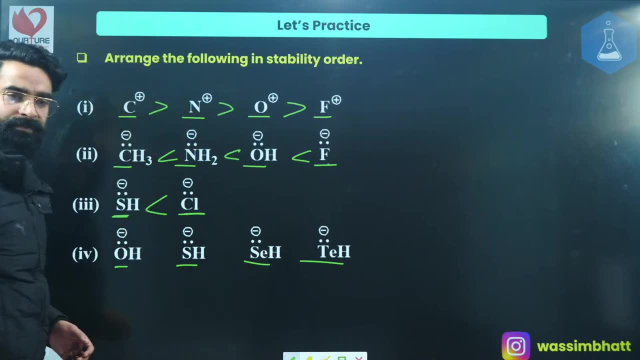 And negative charge is more stable on more electronegative element. As simple as that, Right? Yes, If you talk about the last one, Oxygen, Sulfur, Silurium Tellurium- Right O S. 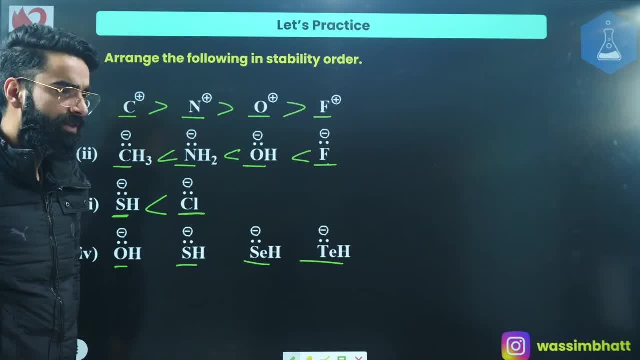 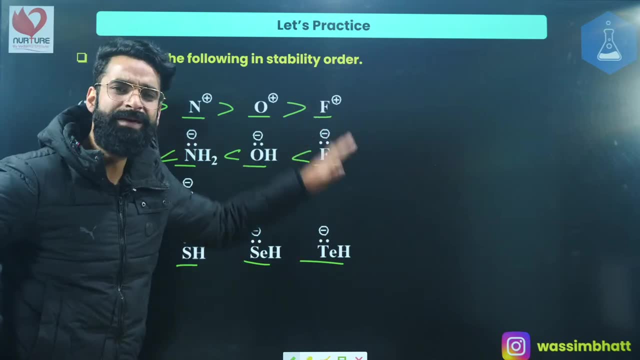 SE T. Do they belong to? Do they belong to Same period or same group? I must say they belong to same group, Right, They are same group elements. Volume charge density comes into play. Volume charge density is inversely proportional to size. 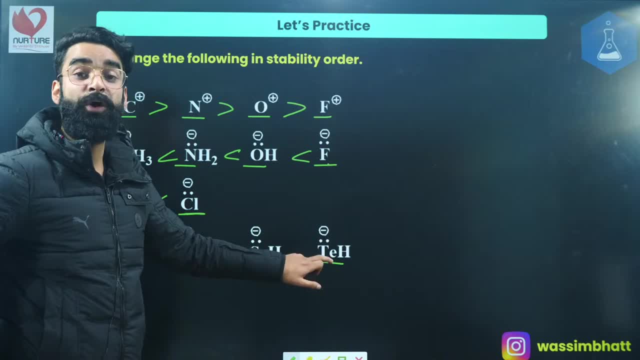 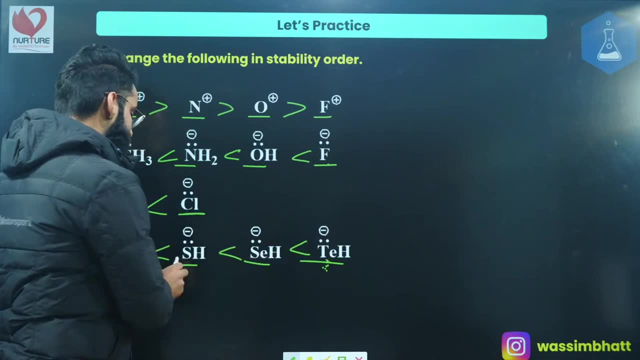 Where is the size maximum? This has got the maximum size, So its volume charge density will be the least. If its volume charge density is least, stability of negative charge will be maximum over here. Right, This is the stability of the negative charge. 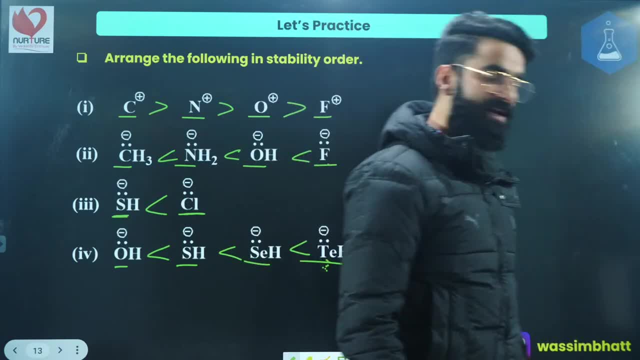 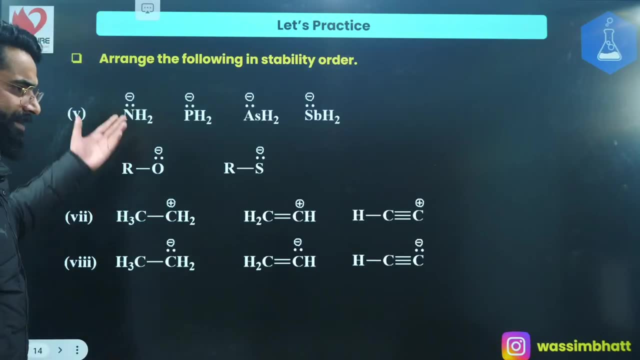 As simple as that. Right, Right, my dear people, Yes, I am sure every single thing is clear Till here. Let's talk about these cases as well. Let's talk about these cases as well. Have a look, Have a look, guys. 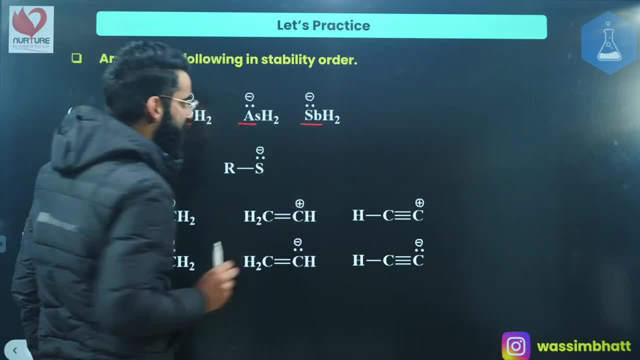 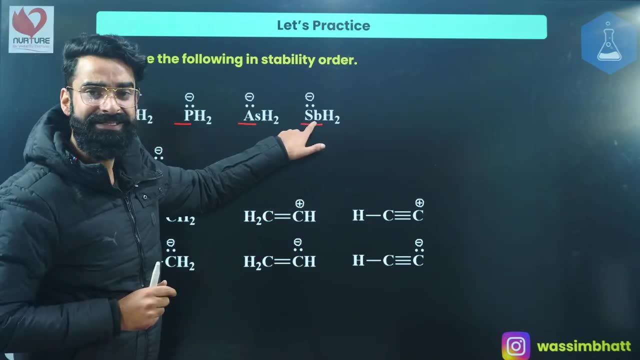 Nitrogen with negative charge, Phosphorus with negative, Arsenic with negative, Antimony with negative. Same group elements. Volume charge density comes into play. More size, More size, because down the group size increases. More size, Less volume charge density. 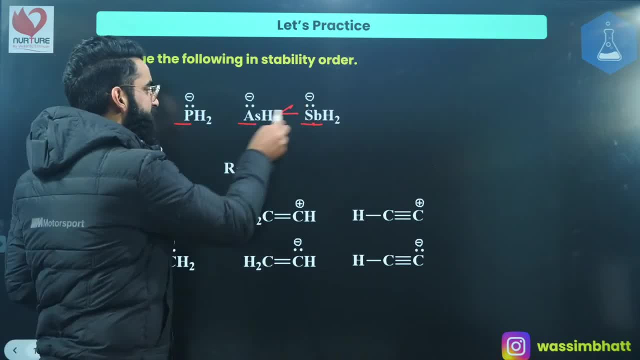 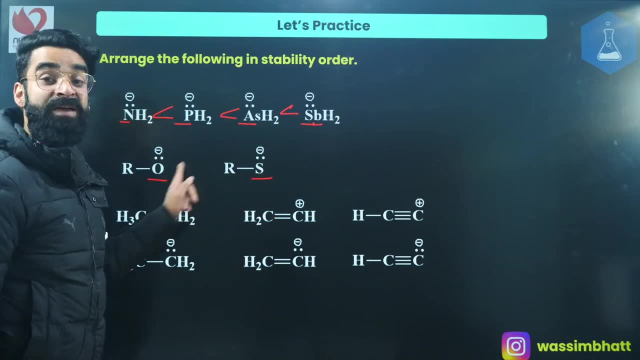 Less volume, charge density, More stability. So negative charge is more stable, More stable over here. followed by this, followed by this. As simple as that. Negative charge on oxygen. negative charge on Sulphur. Same group, Oxygen and Sulphur. they belong to same group. 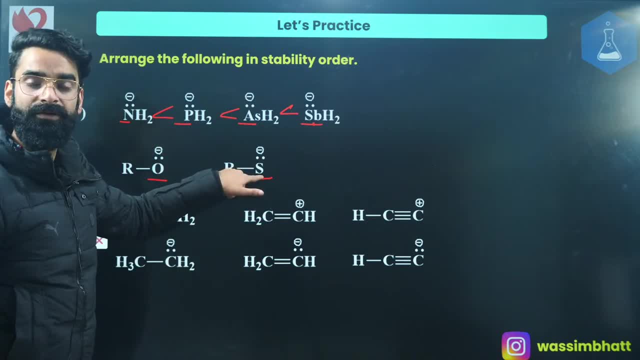 Right Volume charge density, More size of Sulphur, Less volume charge density, More stability. So negative charge is more stable over here, Right, Yes. Similarly, if you talk about the last one, if you talk about this one, see, guys, one thing I would like to share with you. 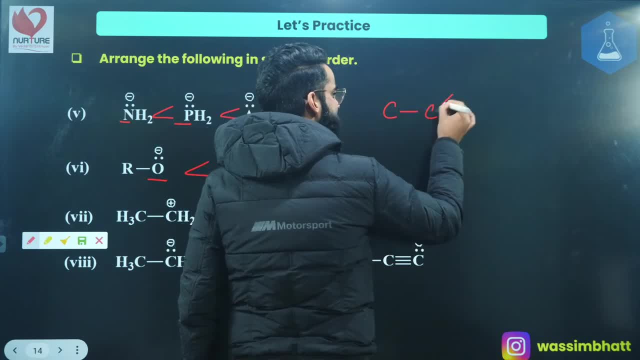 One thing I would like to share with you. Let's say: this is carbon, This is single bond, And this carbon is forming three bonds with hydrogen. Even this carbon is forming three bonds with hydrogen, right, Let's say there's a double bond, right? 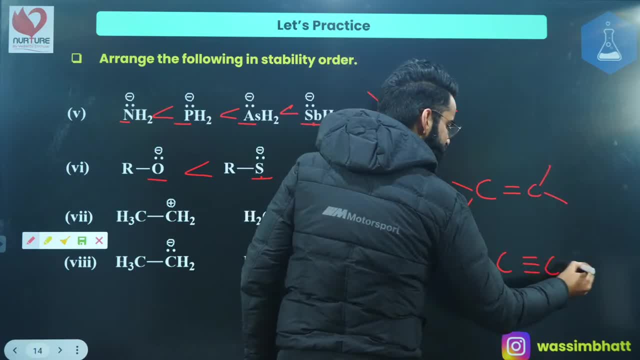 This is forming two bonds, two bonds with hydrogen. There's a triple bond. This is forming one bond with hydrogen, one bond with hydrogen. If I ask you what about the hybridization of this carbon, You'll say it's forming four sigma bonds. 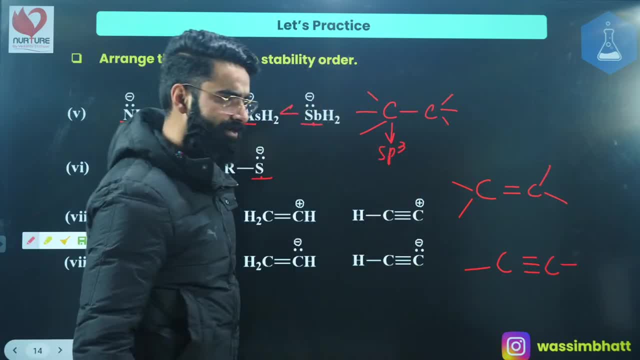 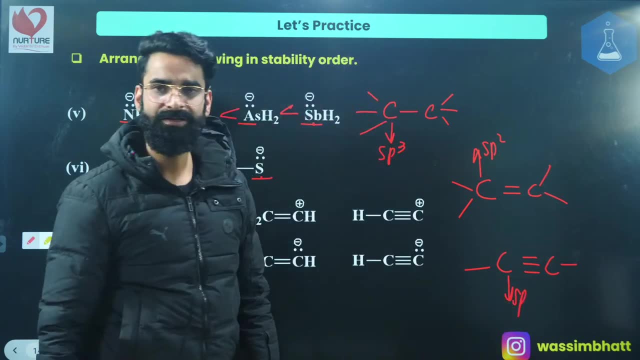 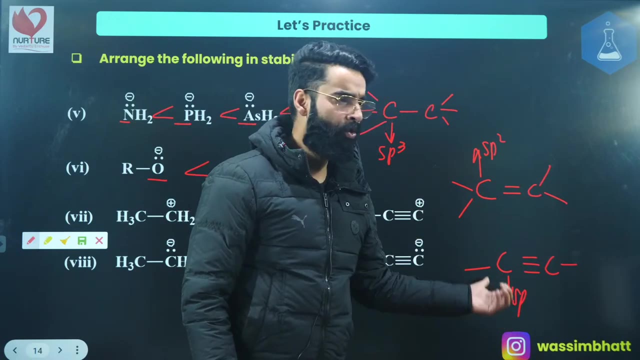 So its hybridization is sp3.. Yes, Right, This is forming three sigma bonds, sp2.. Two sigma bonds, sp. Right, There's something which every one of you knows: Where in the electronegativity is more sp, more s-character, right? 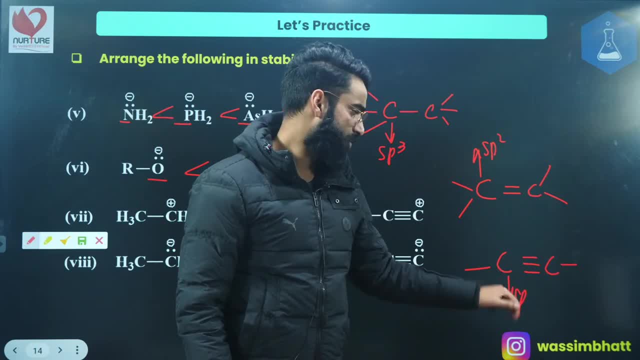 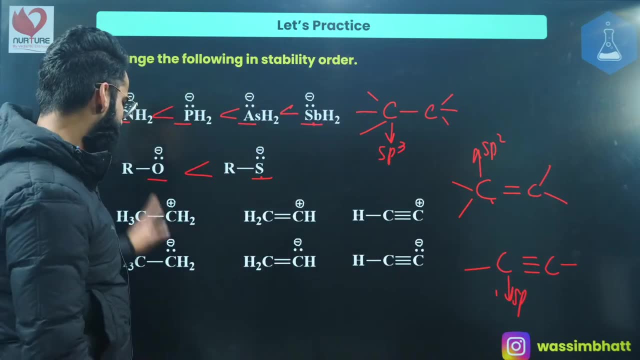 More s-character, more electronegativity. So triple bonded carbon has got more electronegativity than that of double bonded carbon, than that of single bonded carbon. As simple as that. Now compare it: Single bonded carbon, double bonded carbon, triple bonded carbon- right. 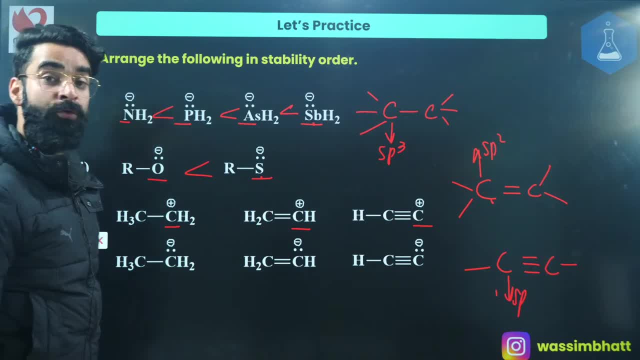 Yes, Positive charge is more stable on less electronegative element. Which carbon is the least, The least electronegative among all? This carbon, this carbon or this carbon? This is single bonded carbon. Its electronegativity will be less. 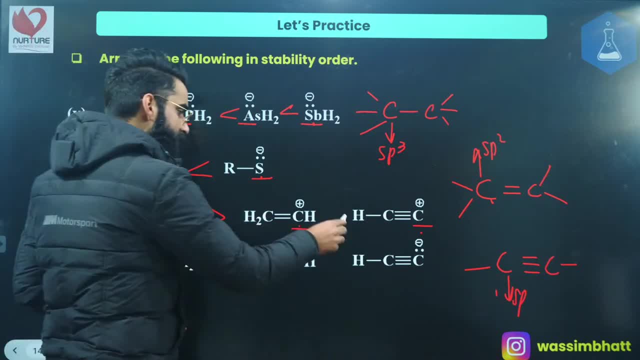 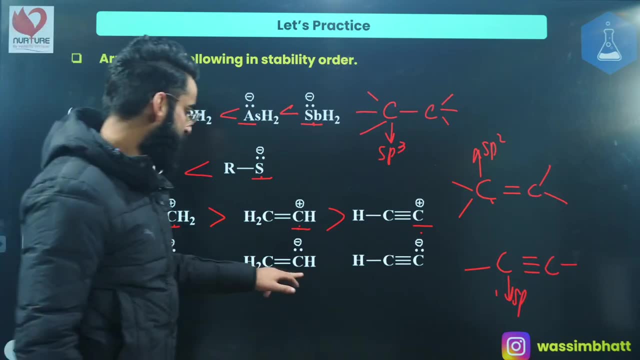 And negative. positive charge is more stable on less electronegative element. Okay, So this is going to be the stability order of the positive charges: Yes Carbon carrying negative. Single bonded carbon carrying negative. Double bonded carbon carrying negative. Triple bonded carbon carrying negative. 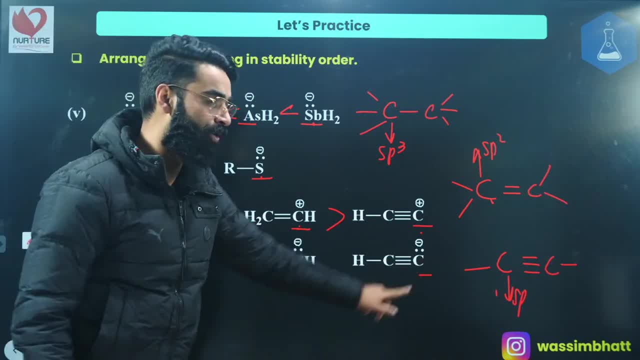 Negative charge is more stable on more electronegative element And triple bonded carbon is more electronegative. So this is the stability order of the negative charges, Right? I'm sure this is clear. I'm sure this is clear. 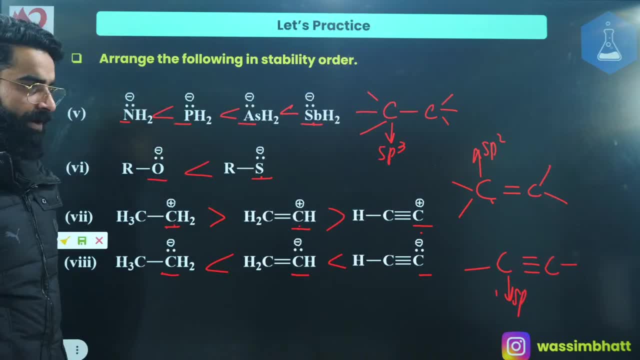 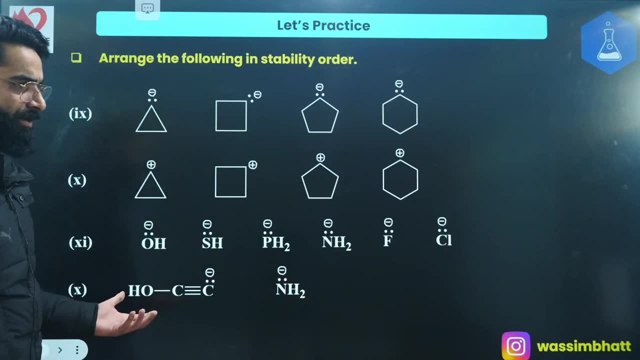 I'm sure this is clear to everyone. Yeah, Right, my dear people, Okay, Let's try to do certain more equations. Right, Let's try to do certain more equations. Okay, These are two more equations which I'm giving you. 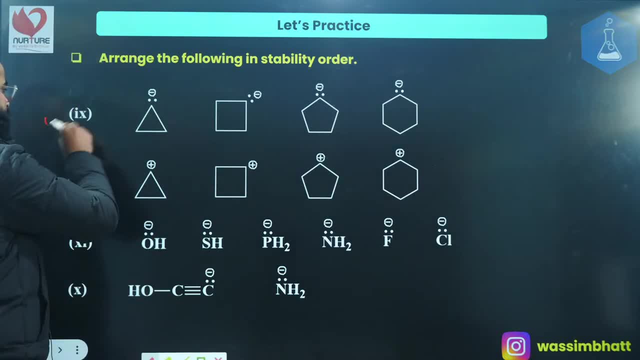 And I will be just showing you this one and this one. These two are going to be your homework, Right? And if you could answer the equations properly, Right? Do write the answer in the comment section If you were not able to answer these two questions. 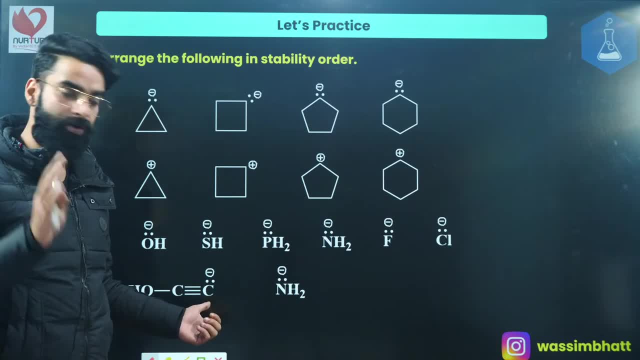 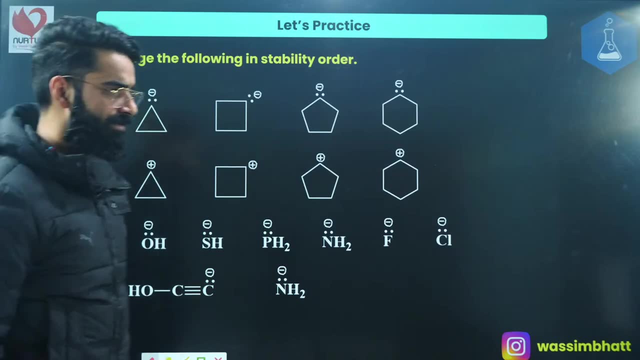 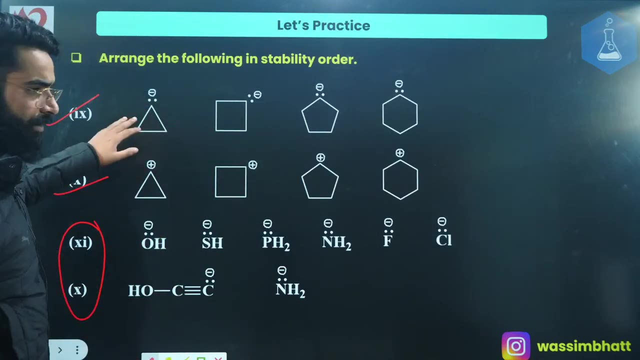 Do let me know in the comment section itself that we could not solve these two questions. Then I'll be starting the next session from these two sessions only. Yeah, Right, Right, people Now have a look. Exactly, Sir, does new batch started for neat repeaters? 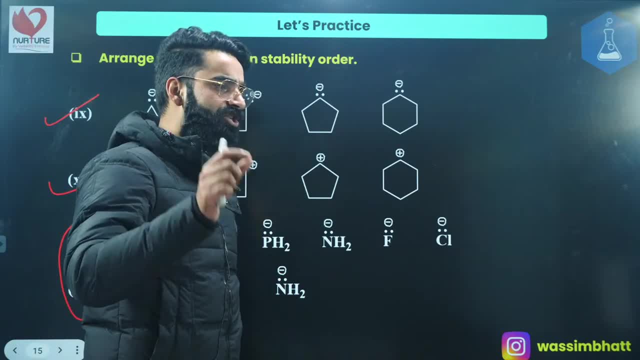 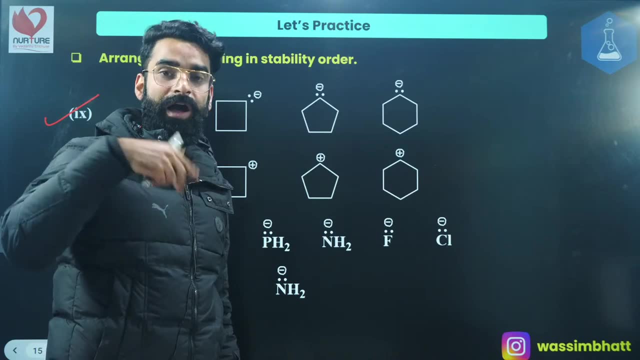 Yes, yes, New batch is starting. I've already shared a video on Neat Elite Channel tonight. only Right, Do check that video. You'll get to know how to get enrolled in that new batch which has started on the actual Vedanta platform. 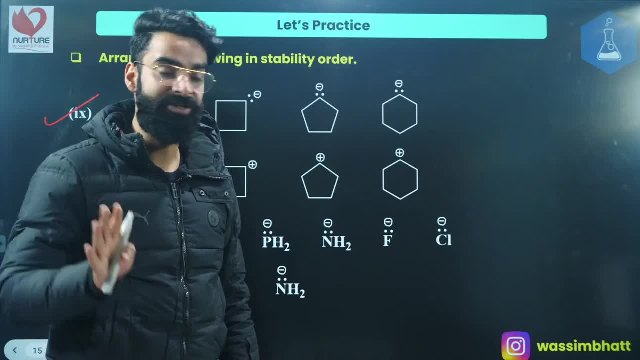 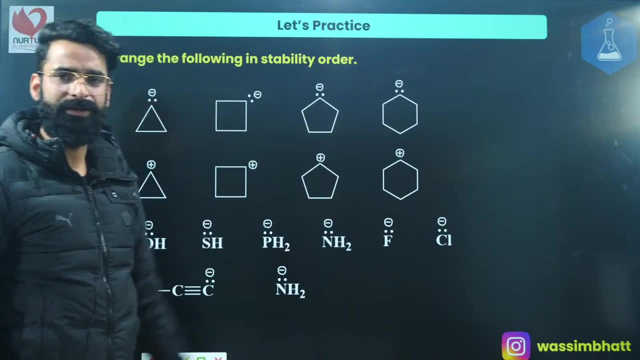 Tonight only, I've shared a video on Neat Elite English Channel. Do check that out, Right, Okay, Now guys have a look. I need to see where is the negative charge more stable. You guys can tell me easily where is the negative charge more stable? 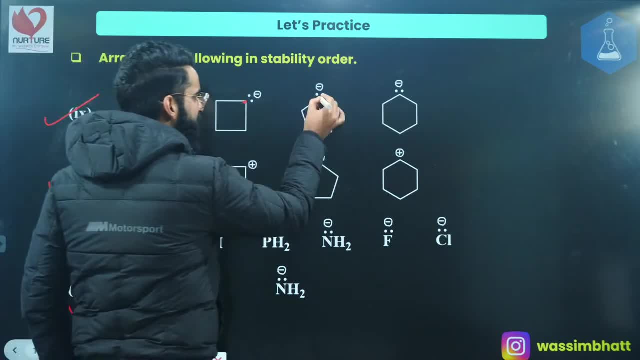 See, For example, if I talk about this carbon, if I talk about this one, if I talk about this one, if I talk about this one, Which carbon is more electronegative? First of all, this carbon is more electronegative. 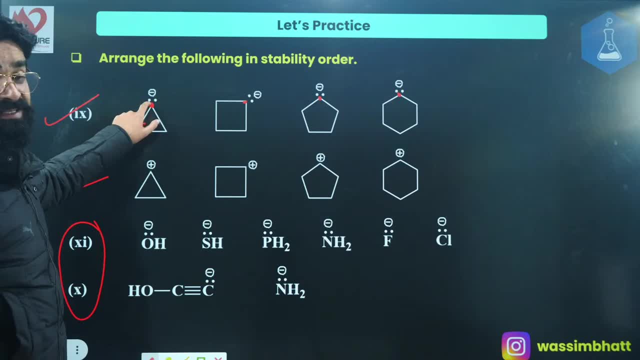 This carbon is more electronegative- Right, And we have seen the reason as well. This is under this ring- is under more angular strain, Right. Yes, This carbon is more electronegative as compared to this Right. 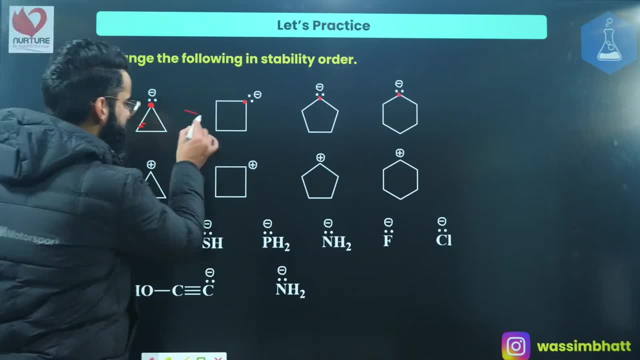 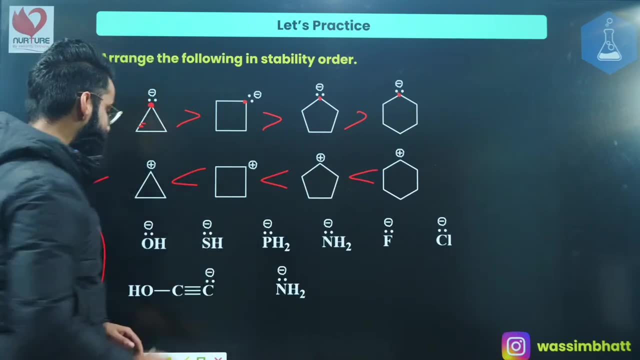 Negative charge is more stable on more electronegative element. That's something which I've told you a few minutes back. So this is the stability order. Positive charge is more stable on less electronegative element element. so this is the order right. these two are absolutely going to be your. 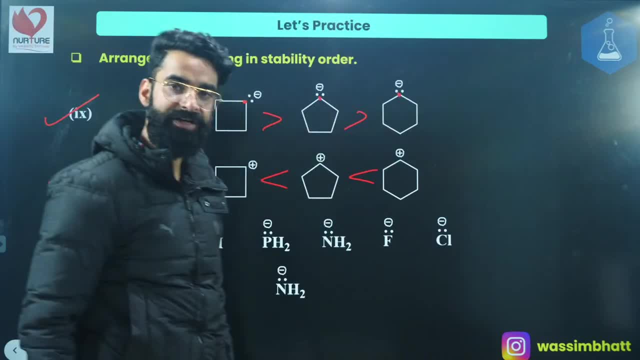 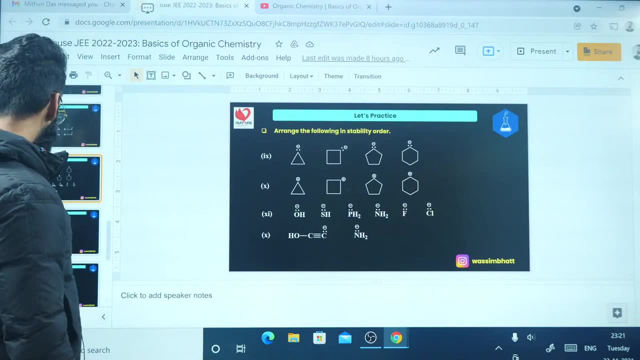 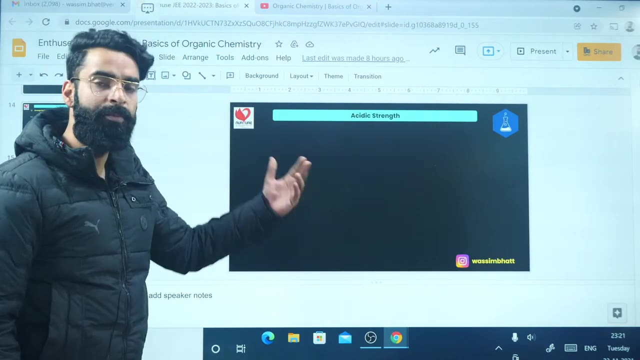 homework questions. do let me know their answers in the comment section. right? so, people, I think this much is enough for the first session of your go see right. in the next session we will be talking about the acidic strength. we will be comparing the acidic strengths. right, but a car, you can just drag the video a. 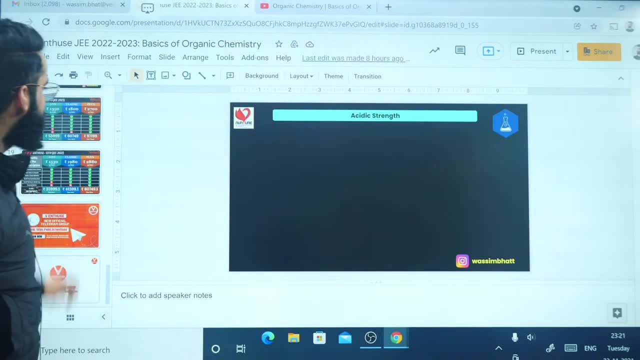 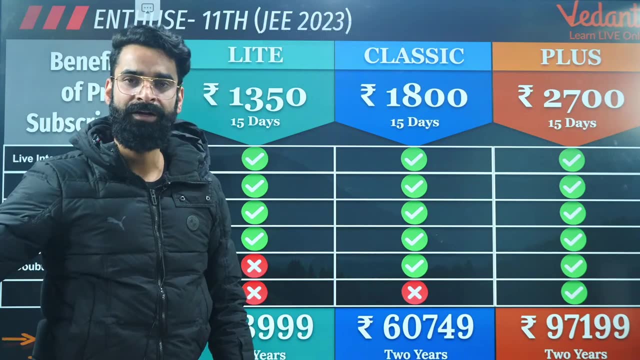 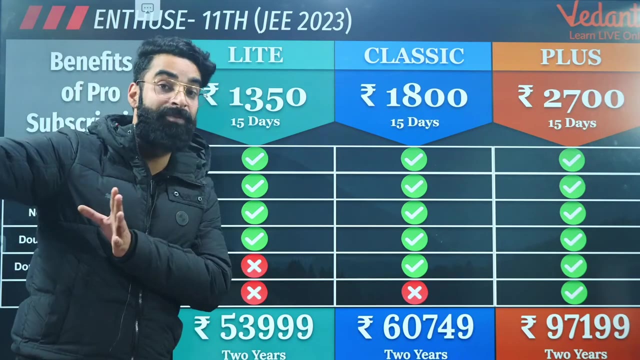 little back. it'll be replay for you, okay, and the ones who have not joined into the actual Vedantu platform, into the actual long-term batch taken by us, taken by the masteries of Vedantu, you can still take it right. well, how to get enrolled into the actual batch which is there on the actual, with on the platform? 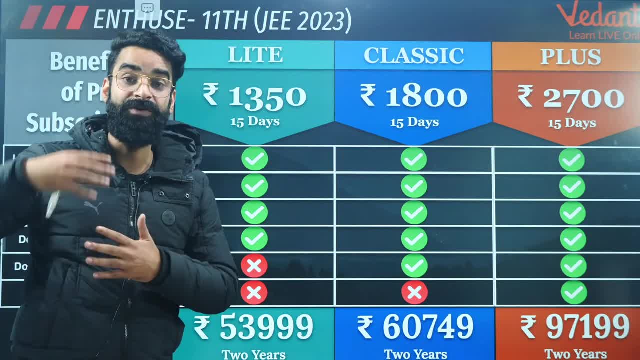 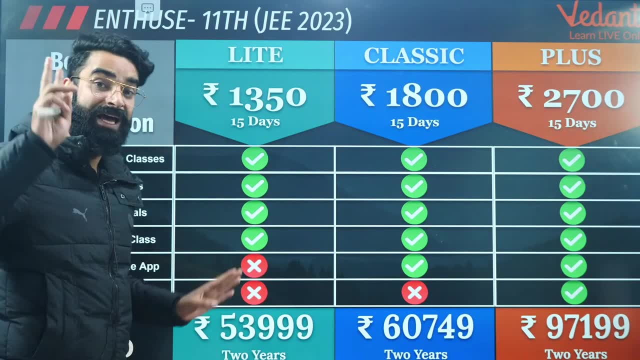 right, in which tests are happening continuously, in which you get the study material right, which is one of the finest study material across the country. right, you need to. you need to get enrolled into that batch which is there on the actual with on the platform right by taking 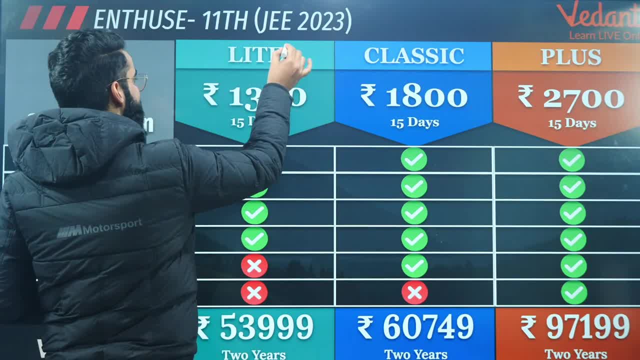 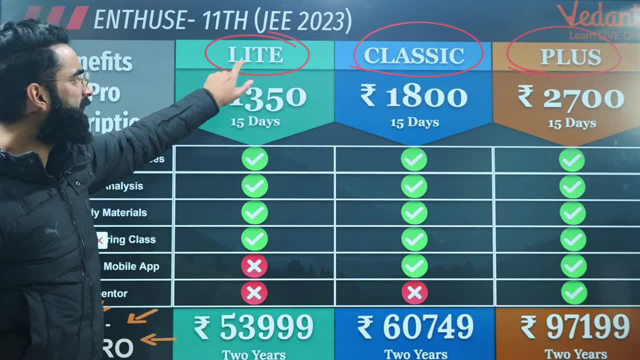 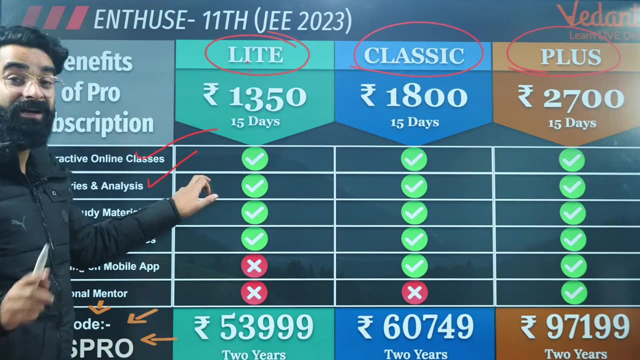 and any of these plans? yes, biting, any of these plans. and what are these plans all about? let me give the quick description of these plans. if you talk about the light plan, if you are taking the light plan, you'll be getting the live online interactive classes. test cities will be conducted regularly. notes and study. 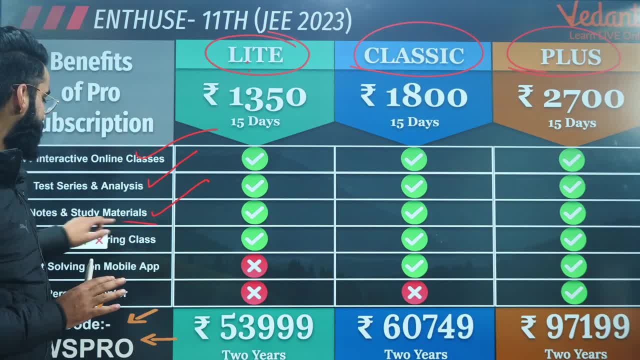 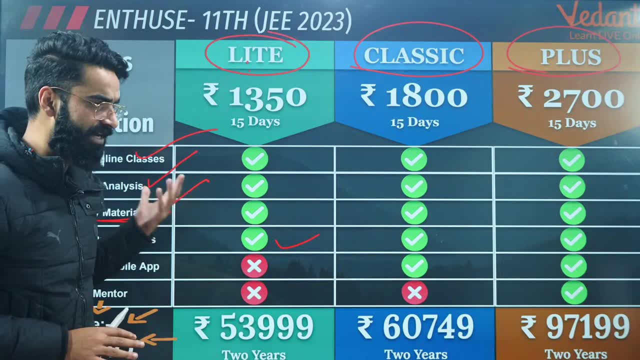 material will be giving, given to you. this is the best thing: study material, that will material, one of the best materials which you can find across the country: doubt solving during the classes. these are the features you, which you guys, will be getting if you are getting enrolled in the actual batch, which is a 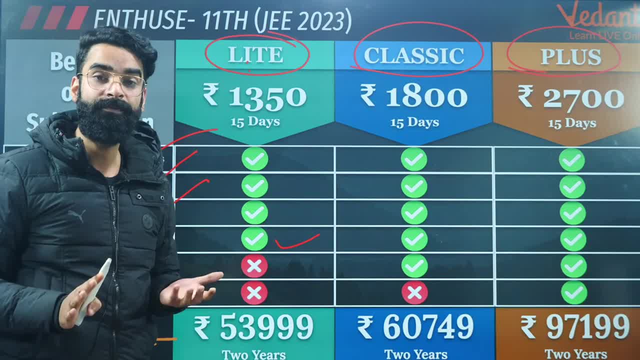 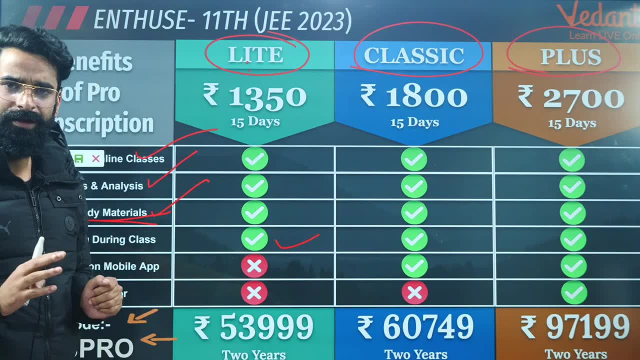 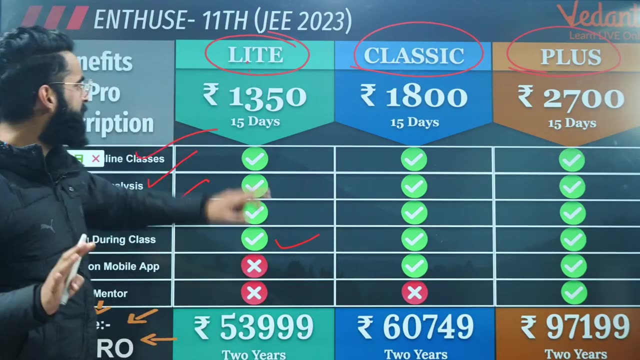 digital version of a crypto platform. so we are going to talk about this: how to get enrolled into the actual with an the platform. if you are getting enrolled into the actual batch- the ones which are preparing for J 2023- right? if you are new to it, up to you have no idea how the actual with on the platform looks like. 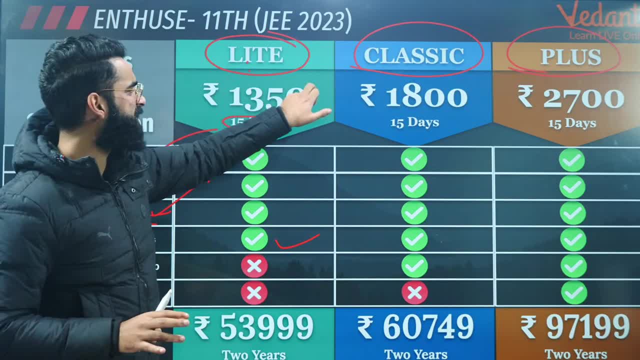 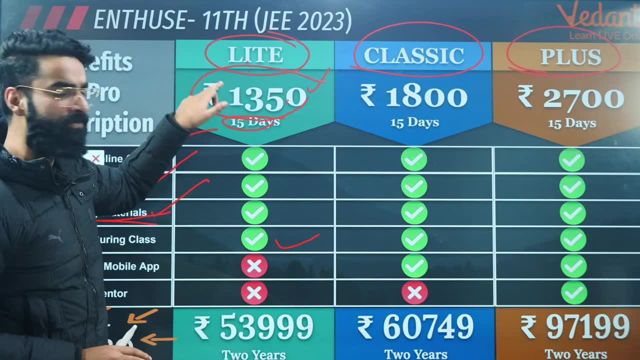 how the actual class are taken on the actual on the platform. you can take this plan for 15 days as well, and only this much amount. you need to pay for 15 days, not even this much amount. if you are using the code WSP RO. you did, you'll be. 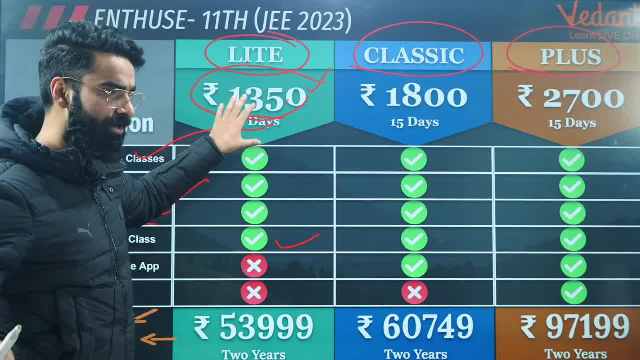 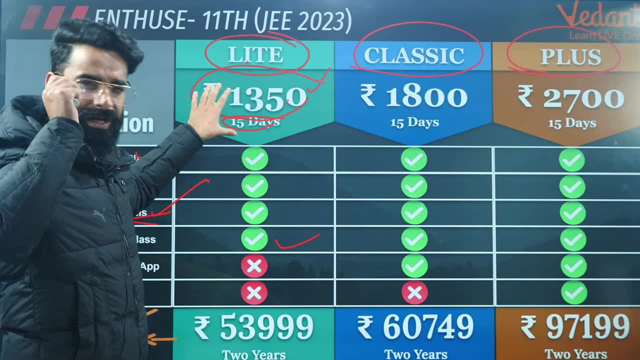 If you want to see it, if you want to see the actual classes on actual within the platform, right, You can take the subscription. You can take the slide program for 15 days, right, Definitely, you guys are going to love it. 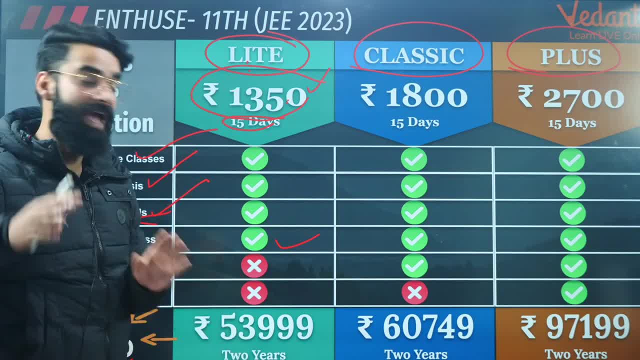 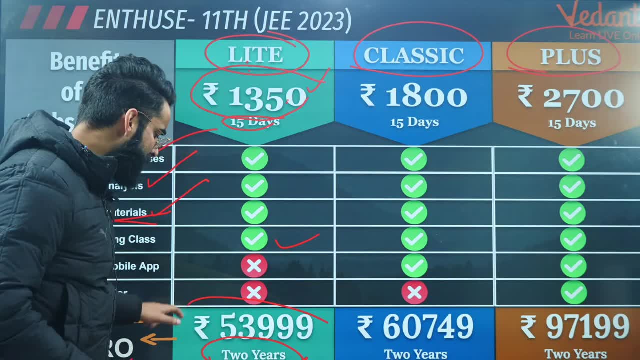 Trust me on that- And automatically you can enroll yourself into the actual batch, And this batch is particularly a two-year classroom program, which I'm talking about, right- And even this much of amount, which is a complete package for two years. 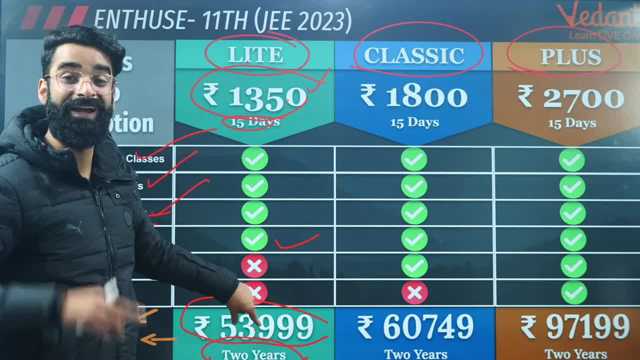 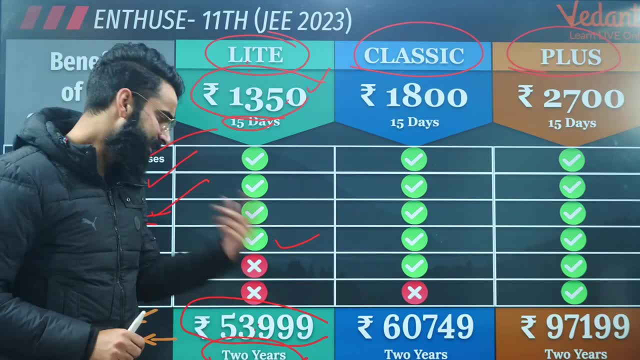 you need not to pay this much of amount in one go. If you are later on, if you are later on going for that batch for two years, right. You need not to pay this much amount in one go. Vedantu has kept an EMI option for this as well, right? 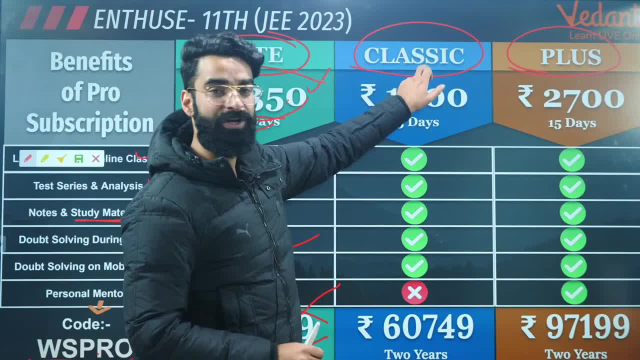 So monthly you can pay the fee. Same is the case for Classic. What all features, what all extra features you get in Classic? In Classic, the extra feature which you'll be getting, that is, doubt solving in the mobile app. 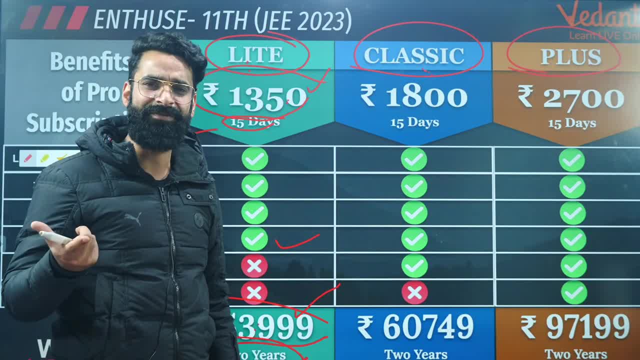 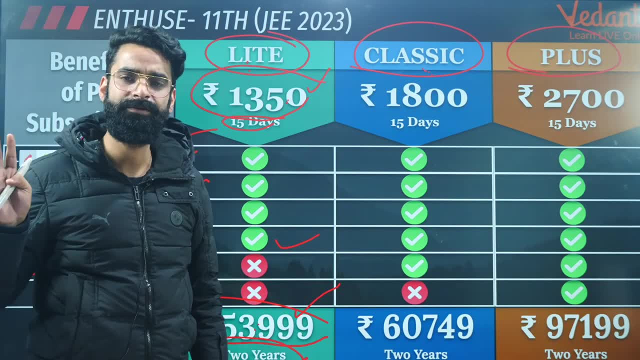 You'll be getting an app Whenever after the class you'll be having any sort of doubt. you just need to put that question, your doubt on the app. You'll be automatically cleared. You'll be cleared without doubt, right? Yes? 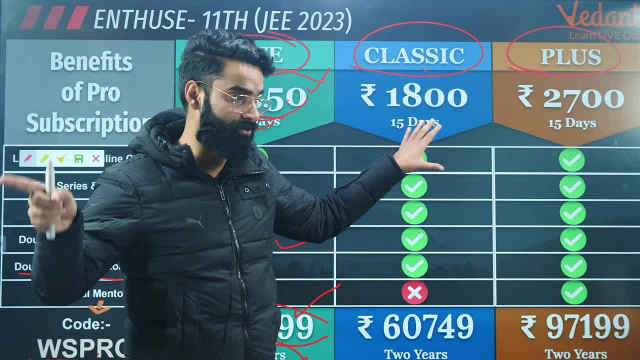 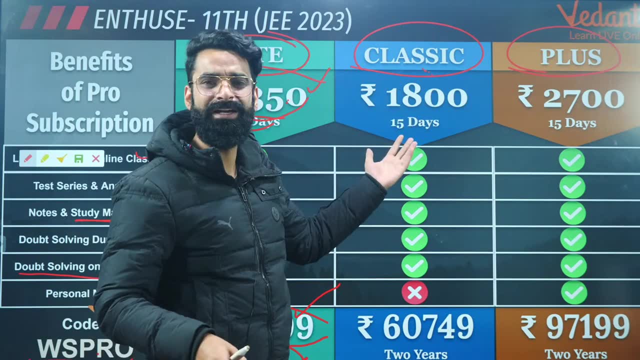 Even this course, if you are getting enrolled in the batch which is then on the actual within the platform, through this program, through this Classic program, right Even, you can give it a try for 15 days as well, Just see if it is working for you. 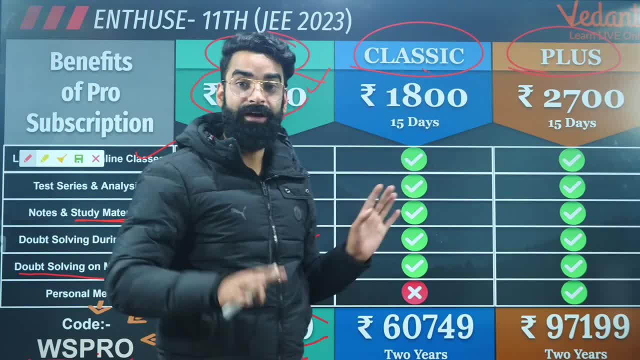 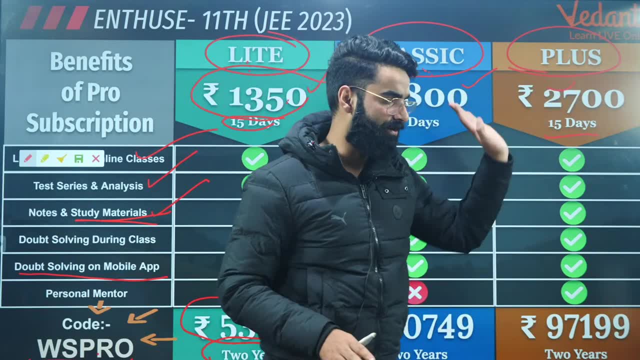 Trust me, you're going to love it. Yes, Similarly, you can enroll into the batch through this program as well. You can take again this for 15 days first of all. Just this much of amount you need to pay. That's all right. 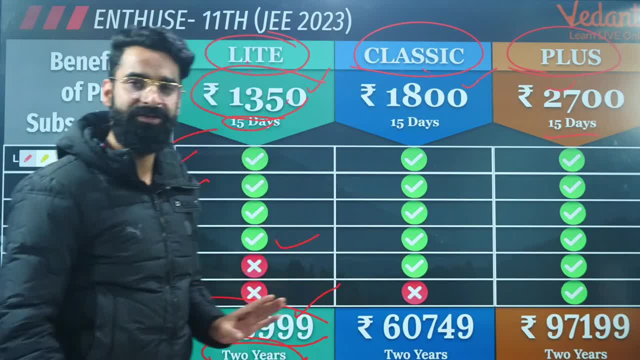 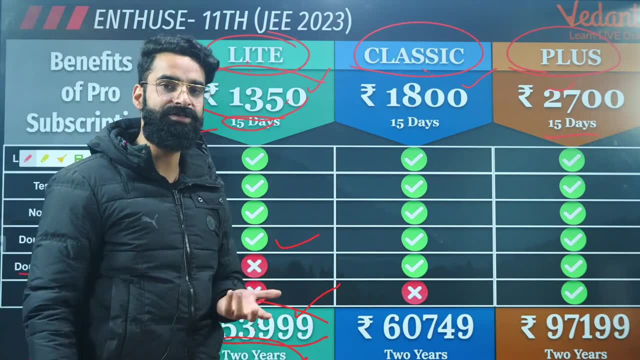 So take any one of these plans, Absolutely. trust me, You guys are going to love it. Okay, And majority of the advanced selections. you would have seen the advanced selections this year, Some 1570 selections came directly from our long-term batches. right, 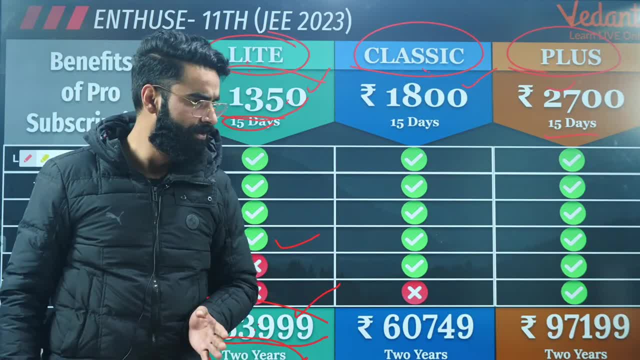 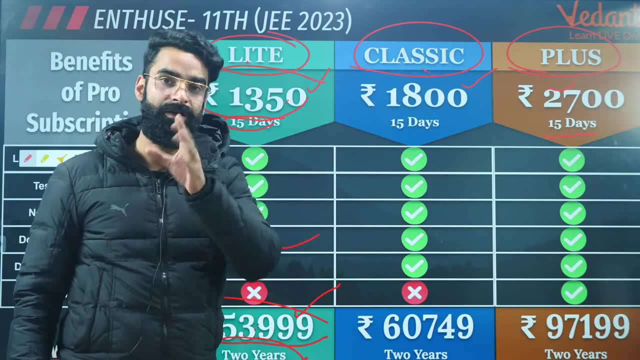 Okay, So do get enrolled as soon as possible. if you are new to Vedantu, So do give it a try, at least for 15 days. Enroll yourself for 15 days in any of these through any of these courses in the actual Vedantu batch, okay. 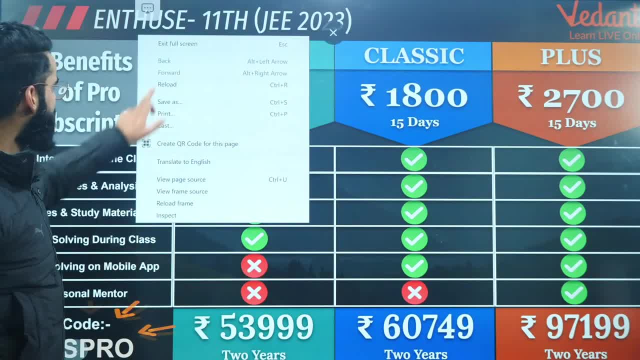 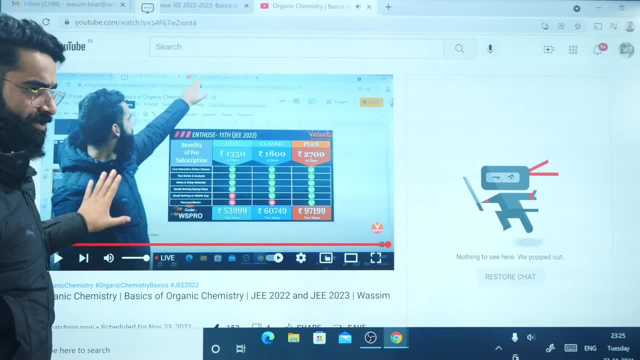 And let me show you exactly how to get enrolled into this batch. Let me show you exactly. See, this is the video which you guys are currently watching, right? Yes, sir, This is the video which you guys are currently watching, yeah. 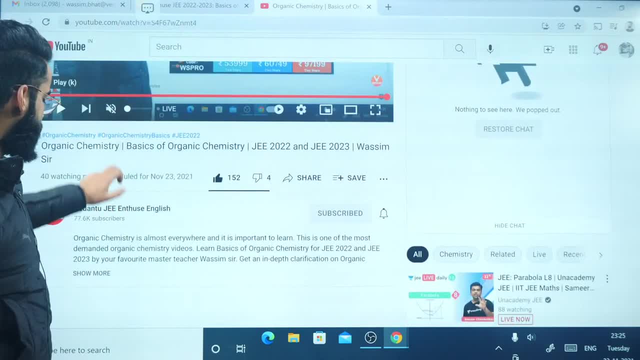 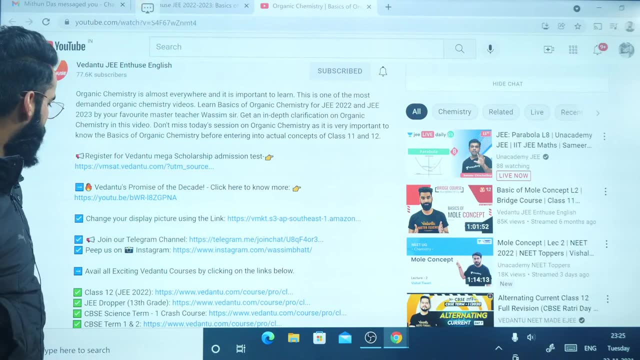 You need to drag this video a little down. And when you drag this video a little down, you need to click on this show more. There's a term show more over here. Click on this show more. After clicking on this show more, you'll be getting a lot of links. my dear people, 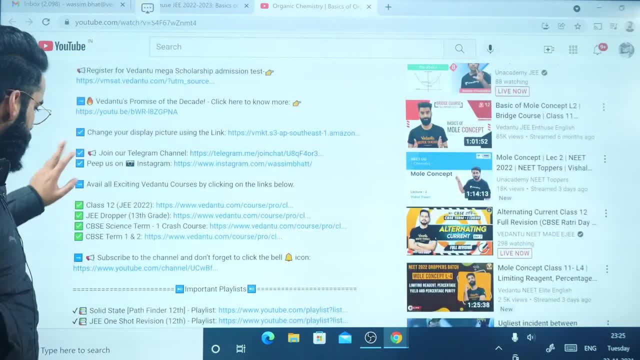 You'll be getting a lot of links. Yes See, let me show you which link you're going to click on. Just a second, Let me find the link first. Well, I'm not finding it. Where is it? Where is it? 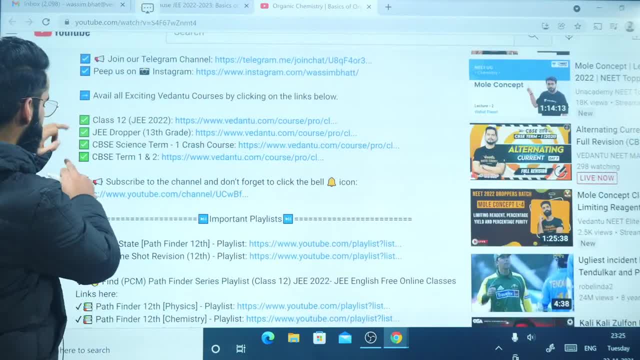 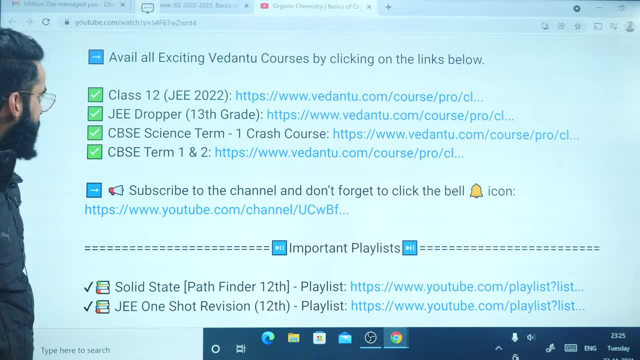 Where is it? Yes, see, there are. I'm zooming it in right. These four links will be there, right? Yes, on which you have got this green colored tick. Okay, So any of these plans you guys can take, right.